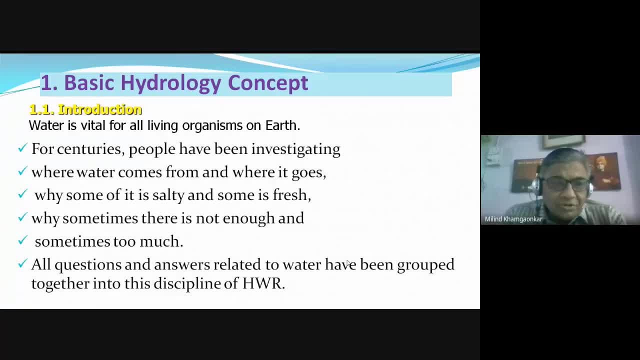 know that the water is the important part of our life and therefore the living organisms and the thinking organisms, like the human beings. they have always this question in mind, since centuries: that where from this water comes, where it goes, why some water is salty and some is fresh. why sometimes it is not. So let us see how much we can cover within this duration of one hour, or we will say we will take a bit more. So let us see how much we can cover within this duration of one hour, or we will say we will take a bit more. 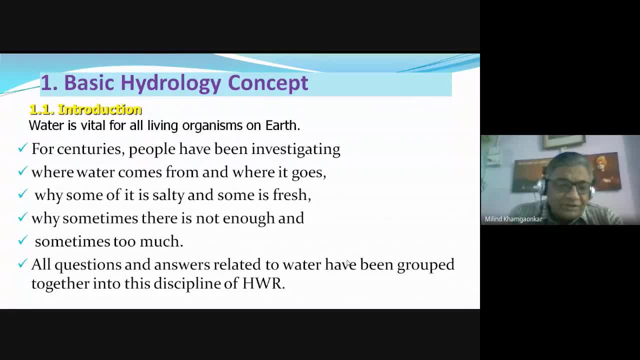 Sometimes there is not enough rainfall and sometimes there is excess rainfall, And all this human culture, or all human beings are 101%- depend on the water, because without water we cannot live for an hour. So therefore, that is the importance of water and all the cultures from the Mohenjo-daro Harappa to you can take your small towns and cities and villages. 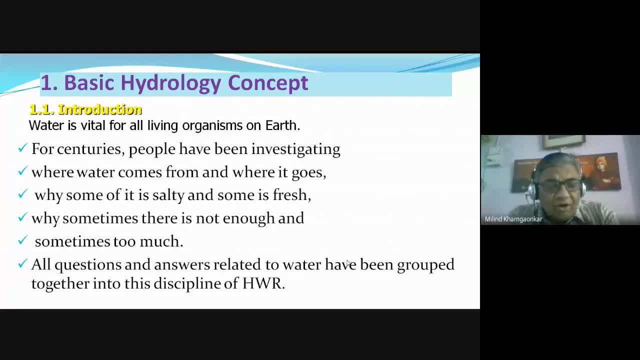 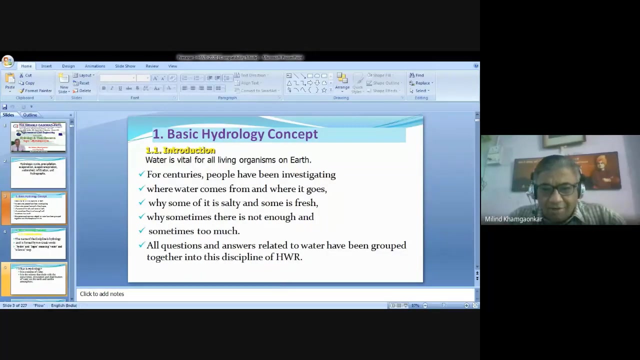 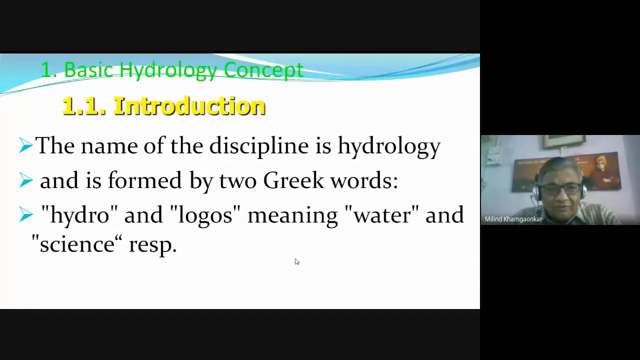 all are situated almost on the river banks or on the river nearby the river, so that they we should get the permanent water supply. So all these questions related to the water are being covered in the subject that is called the hydrology, Wherein this hydro and the loogie- both these words- have originated from the Greek greek alphabets. 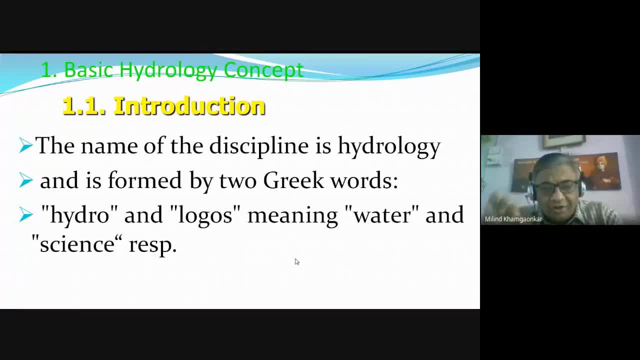 There are joins which have lot of water and tendtmost bodies to form fuel strengths. There are some춤 that are very different from those used in the past. By nature, a filtration path is created from the water itself. So earlier during the times when we were based, for example, when we used towards other soil, the water was not flowed to water Falling down and Emma would shed earth just to yak out and that water would thick and önemich the slAG because the water was not, please, connected with place to the recipient. 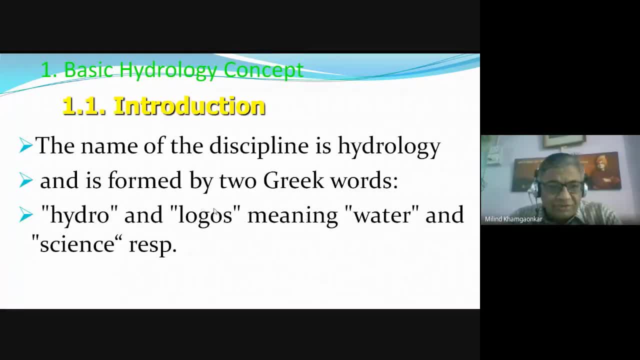 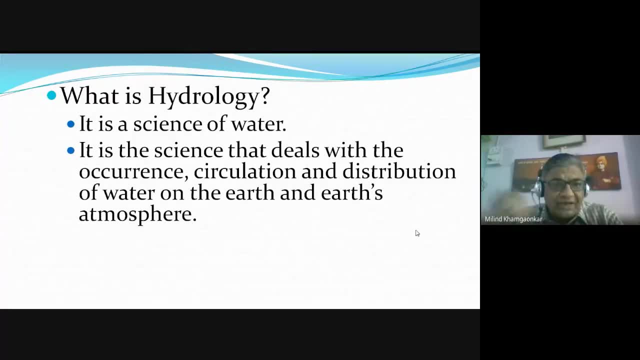 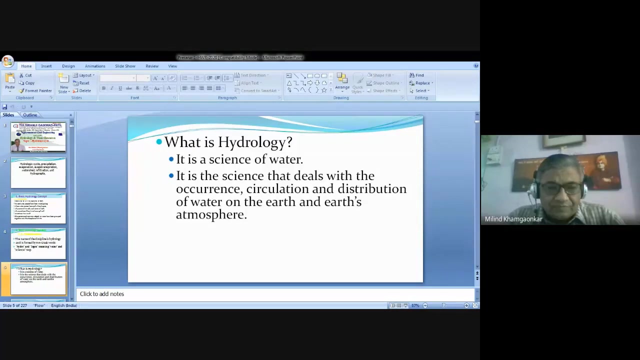 water and logy or logos means science. therefore, the hydrology world has evolved from this. so definitely it is the science of water. okay, this science deals with the occurrence, means where from this water comes, the circulation, how this water gets circulated in different forms. may be a liquid form, may be a solid form or maybe a gaseous form. so this is being studied in this. 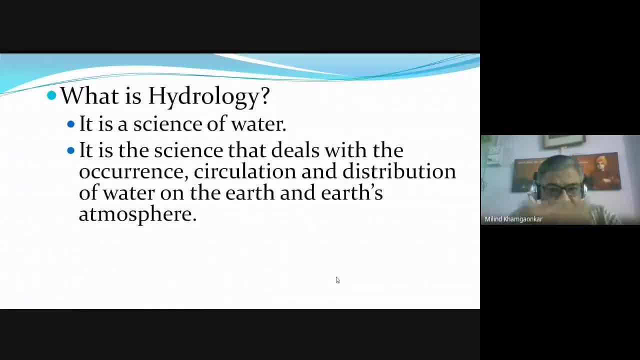 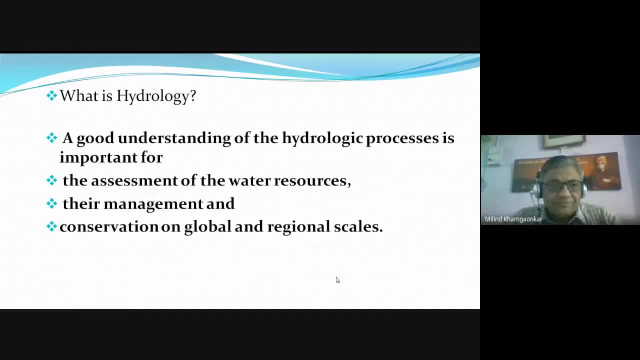 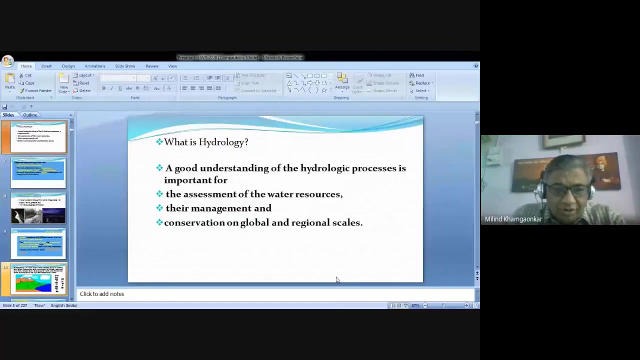 subject which is called as the hydrology, that is, the occurrence, circulation and distribution of water on the earth and the Earth's atmosphere. and, as I have been telling you again and again, a very good understanding of this hydrologic process, or the hydrology, helps us in exact 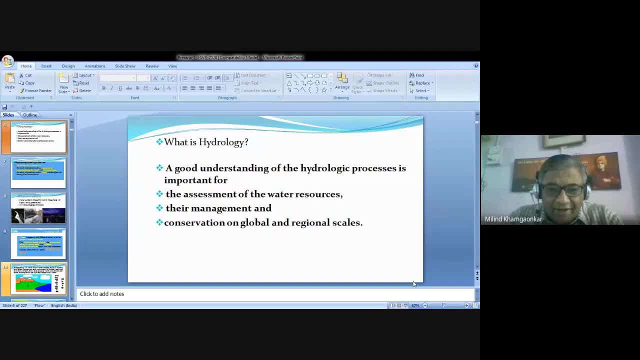 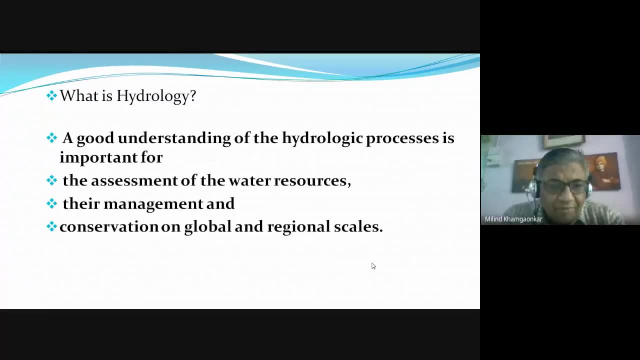 assessment or exact finding of the quantity of the water that will be available, that we can assess in advance so that we can manage that water which will be available to us. and also the conservation of water on the local scale, district scale, regional scale, on on country scale has become a very importance, important subject. 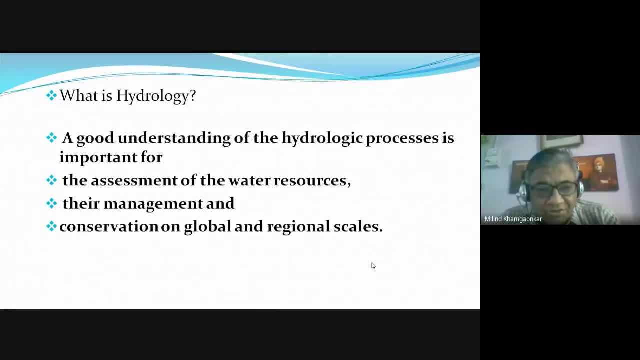 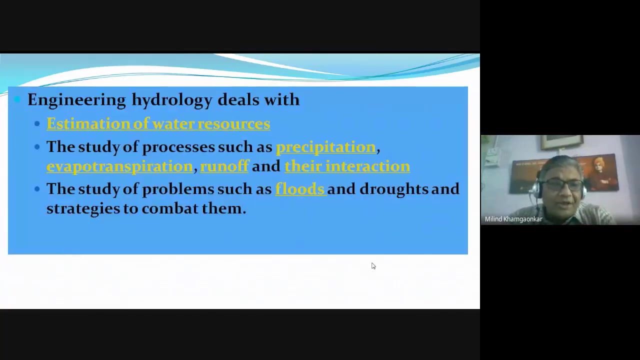 nowadays, because the nature has. nature is now very fluctuating. sometimes it rains very heavy and sometimes there are certain patches, certain periods when the rain does not occur. so conservation of water is also very important. so engineering hydraulic deals with the estimation of water resources. it includes, or the study process includes, precipitation, that is, the water precipitation at use, clean seawater. 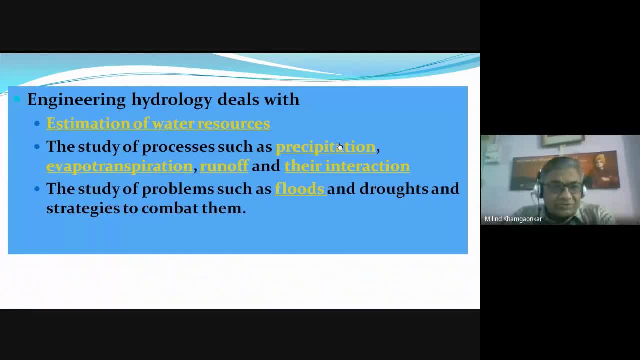 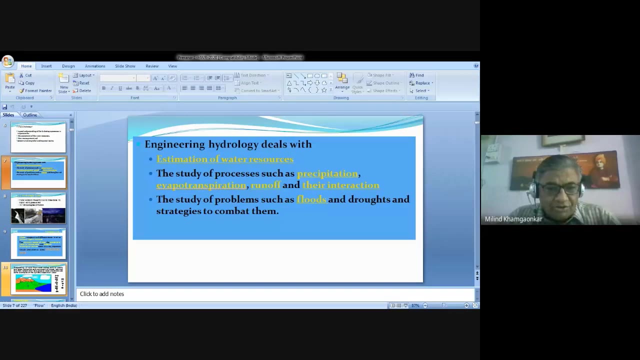 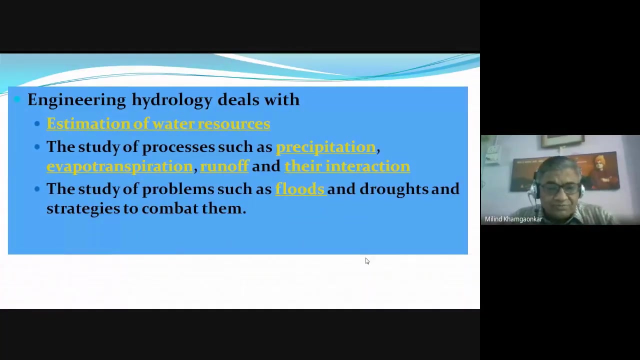 is the rainfall in our, from our sense, evapotranspiration, that is, the evaporation and transpiration, the runoff, and what is their interaction with how they are related to each other? then the question of the floods, because, due to this excess rainfall, for a longer duration, the water crosses the banks of 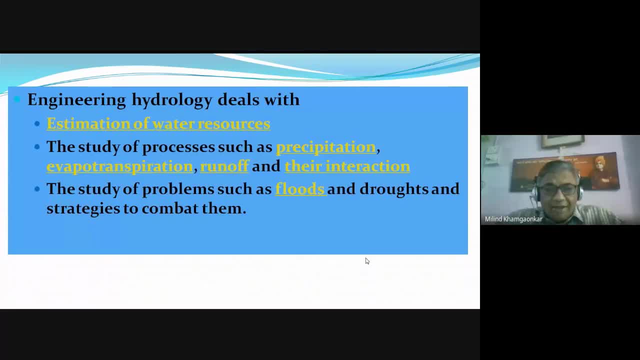 the river and encroaches outside the bank banks and destroys not only human and the animal life but also the other properties also, like that is, the agriculture, the houses, roads, bridges and etc. so on the one side, hidrology helps in tackling the floods as well as on 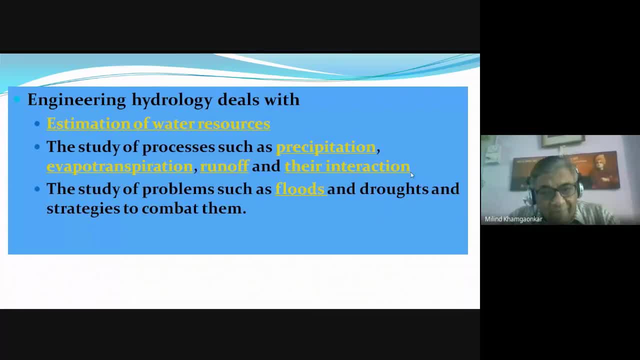 other side, the droughts, that is, the famine, is what we call mahinvi, agree, so many times when it is raining and not anymore. so we face the problem of drought. and if we have the proper study of all this, hydrology and is the science which deals with the occurrence, distribution of the water and 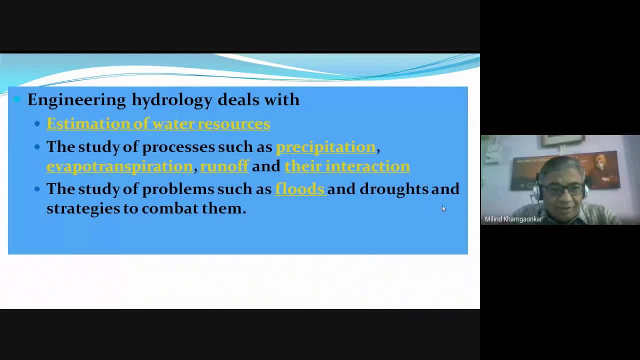 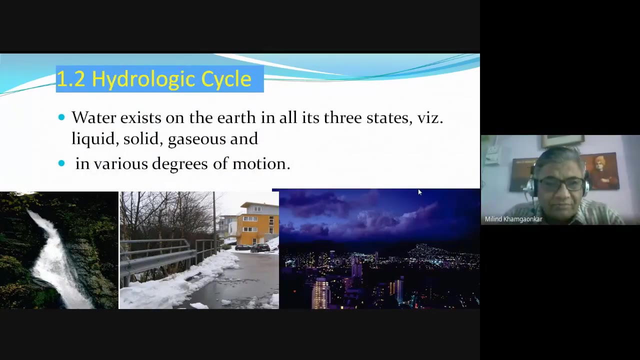 circulation of the water, then we can well in advance plan the strategies to face these two problems of the floods and the droughts. now, a very simple term, a simple phenomena. we will try to understand the hydrologic cycle. friends. we all know, as I have told you just now, that water exists on the earth in three 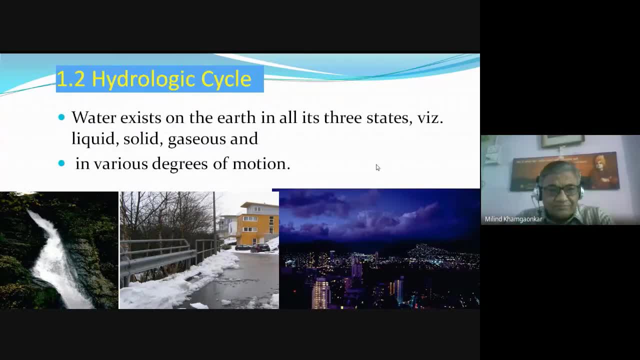 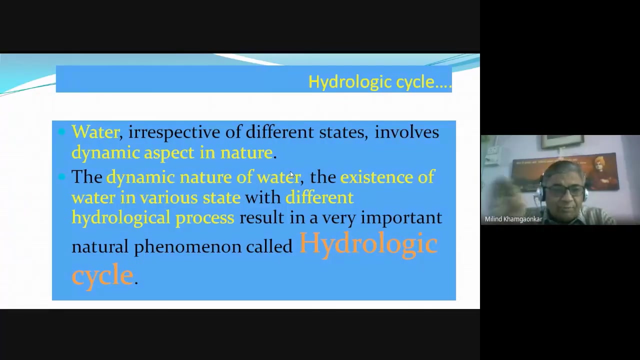 states, that is, a liquid, solid and the gaseous state, and in all these three states the water has the tendency to move from one place to another. okay, so it is always has the property of dynamism that is the movement. it has got this movement property, that is dynamic aspect. it has, or it has a dynamic nature. so due 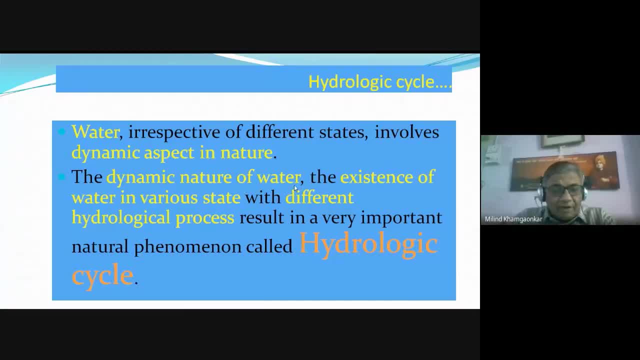 to this dynamic nature that is the movement property, as well as the three states of the water, that is, existence of water in liquid gas and the solid state, a very nice natural phenomena occurs. that natural phenomena is called as the hydrological process, or that is also that hydrological process. 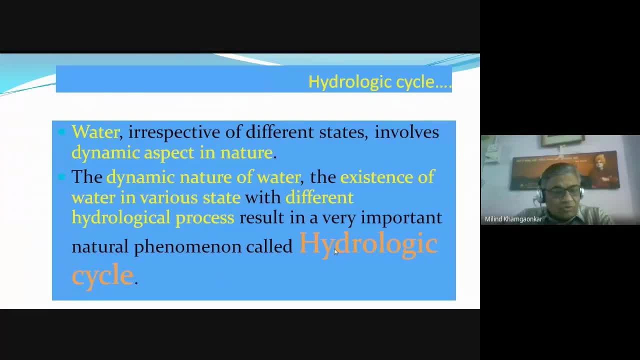 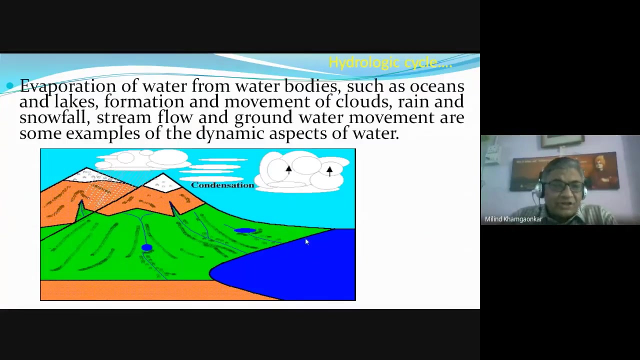 is called as the hydrological cycle. okay, so a very beautiful natural phenomena which is the result of the hydrological process called as the hydrological cycle, by means of which the water in the liquid states gets converted into the gaseous state due to evaporation from the water body that is like the ocean. 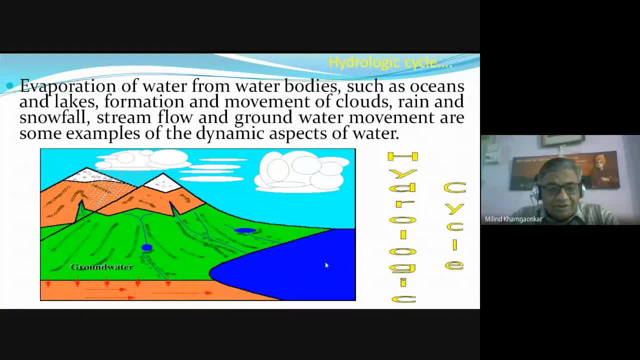 seas, rivers, reservoirs, lakes. due to the solar radiation, due to the solar heat, and after this water gets converted into the vapor state that is due to the evaporation, its density being less than the air, it moves upwards and get to the and after reaching certain height. 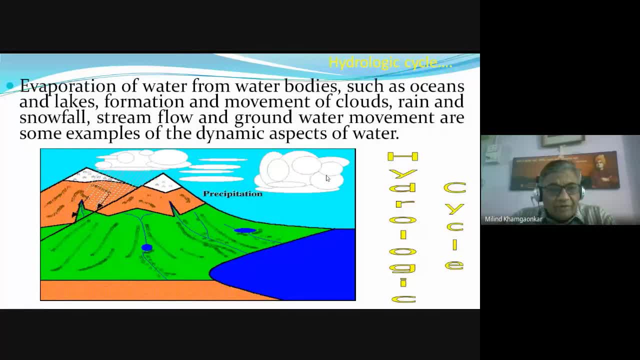 these vapor particles, being very light in nature, they flow with the wind, wind which is called as the flowing air. they flow with the wind and from the water body they reach to the land, sometimes land, and when all these evaporated water particles, that is, the vapor particles. 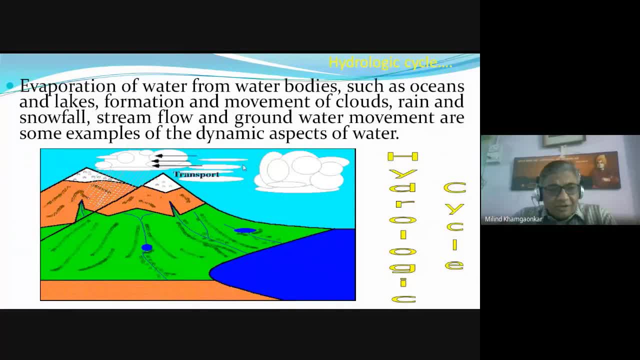 they come very close to each other. due to the cohesion of all these vapor particles, a scientific process called as condensation occurs. condensation means accumulation of the water vapor particles or molecules at one place, resulting in formation of the clouds, and when all these clouds comes very close to each other. 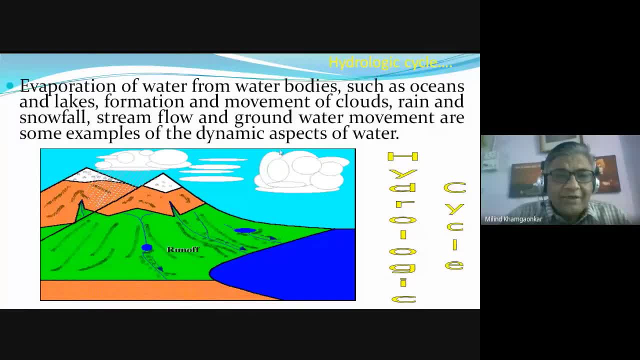 and they become very dense. and if the atmospheric temperature at that height- cloud height- is too less, it is cold. then these condensed cloud particles gets converted into the water particles or sometimes to the ice particles, and these water particles or the ice crystals, the ice particles being heavier than the air due to the gravitational force. 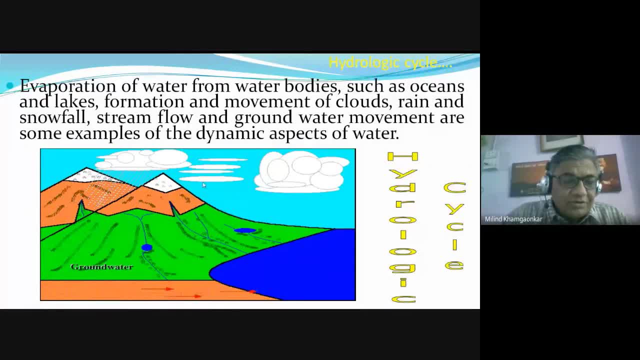 they fall over the earth, maybe on the water body or maybe on the ground or the soil part, and after it falls, this falling of the water particle from the clouds to the ground is called as the precipitation. okay, so this precipitated water falls on the ground either? water precipitation not only includes the fall. 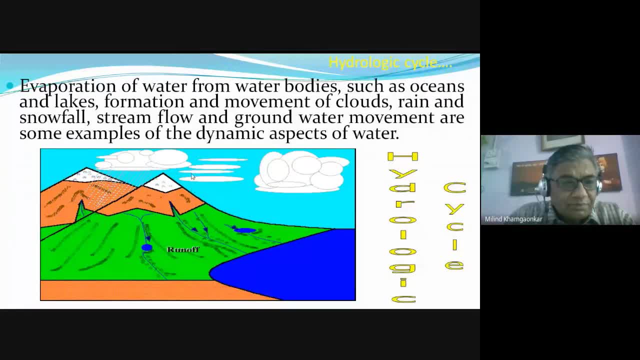 of the water, water particles, rain drops. we call it as, but it also includes the fall of the ice particles also. so it rains, it precipitates on the earth and after falling over the earth, the water particle saturates the soil surface. it fills all the whites of the soil surface and then some water percolates into the. 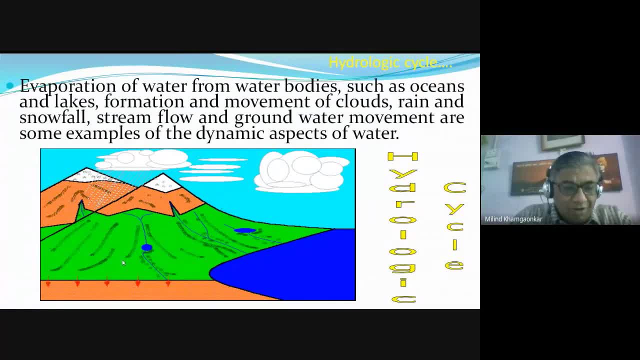 ground, which is called as the infiltration, the watch. some part of the water which is infiltrated also follows the topography of the background and, after saturation of the soil, soil at the top, the water on the precipitation water. some part of the precipitation water follows the stream, the rivers. they are called as the 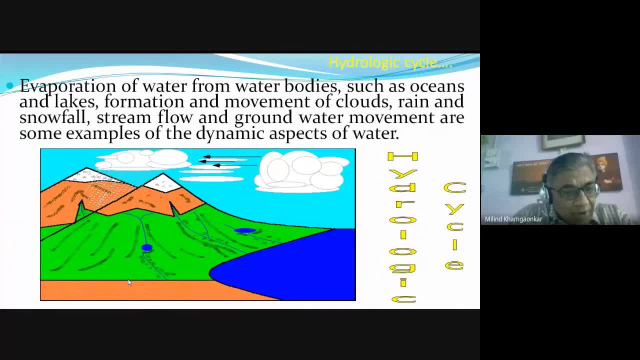 surface runoff. the water which percolates into the ground and follows the topography of the ground is called as the infiltration of the soil surface, which is called as the subsurface runoff, and certain part of the water, due to the gravity, percolates or infiltrates below the ground surface and it reaches the 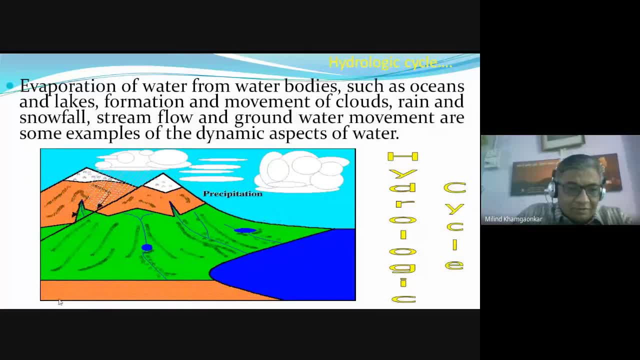 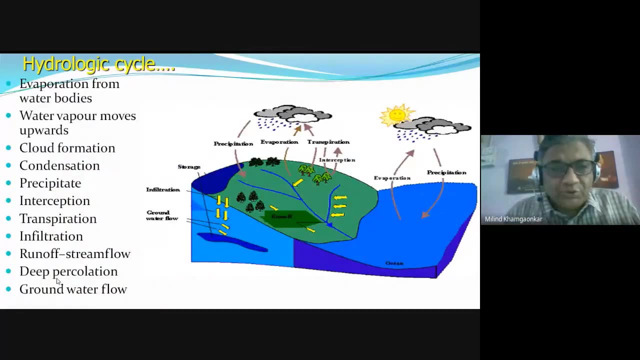 groundwater table and raises the groundwater table is called as the, that runoff is called as the groundwater flow, or that runoff is called as the base flow. and after this water, from the surface as well as subsurface runoff, reaches to the stream or to the water body, maybe ocean, maybe a sea or a lake. 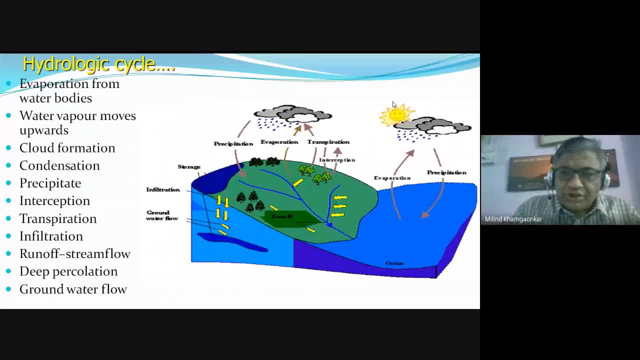 or a reservoir. again due to the sun rays, due to the solar radiation, this water, which is in the liquid form, gets again converted into the vapor, and again this vapor gets converted into the clouds- moment of the clouds- and again falls on the ground. precipitation, condensation, cooling, precipitation. so this process is 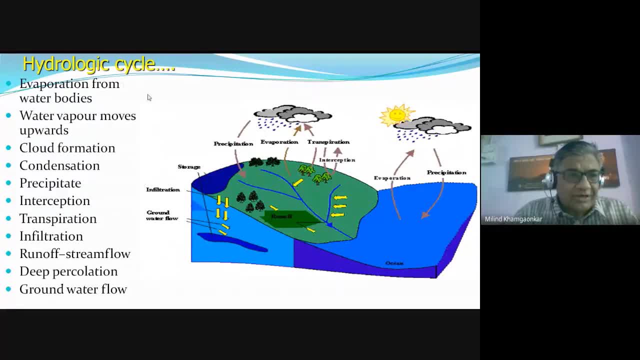 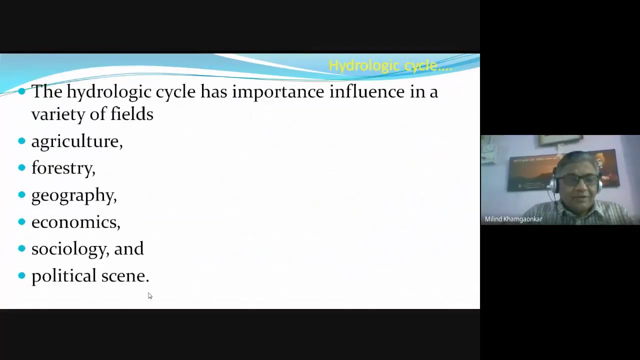 called as the hydraulic cycle, hydrologic cycle or hydraulic cycle. so it includes all these parts. that is, evaporation from water body, water vapor moves upwards, cloud for men, session formation, condensation, precipitation, interception, transpiration, infiltration, runoff, deep percolation, groundwater. the hydraulic side, hydrologic cycle, is very 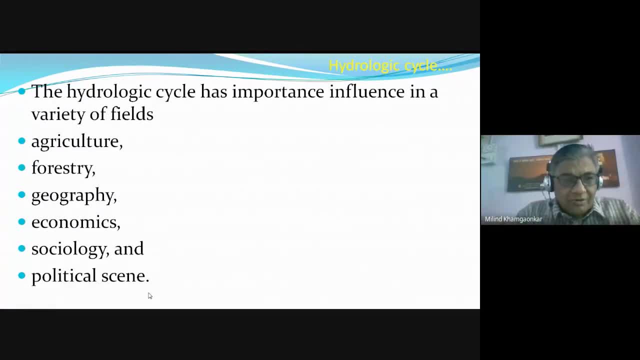 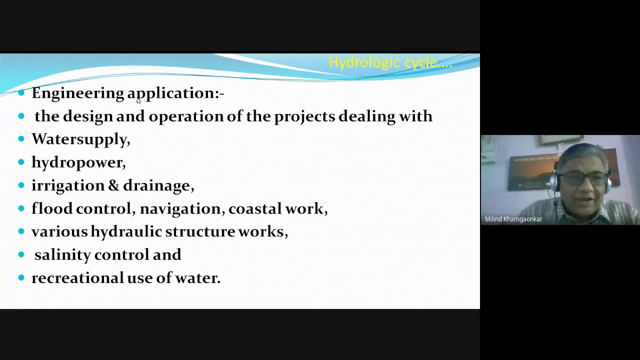 important to our day-to-day life. it is important from the point of view of agriculture, forestry, geography, economics of the country, of the world depends on the precipitation, rainfall, sociological and political scene. from our engineers point of view, the hydrologic study, or hydrologics cycle study, is important from our hydraulic. 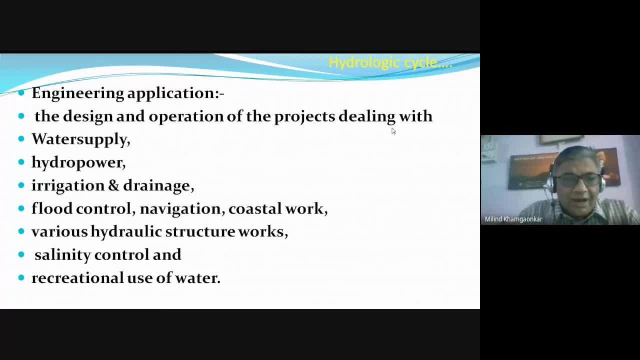 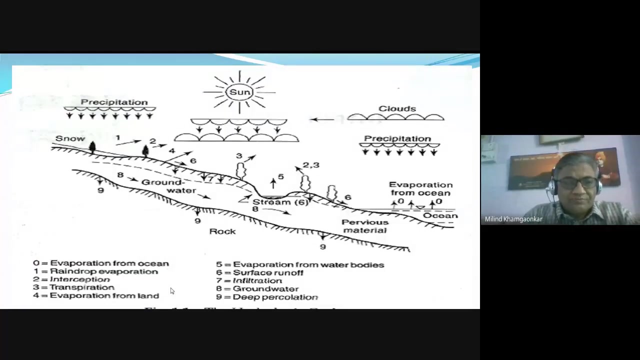 structures for the design and operation of the water. we do seismic life faster BOB days without the water. suddenly that gives us zero amount of tidal species in our water surfacewhere. there is no over why it says it does so at the end of the question. you will start with the one. critical these things of water resources. 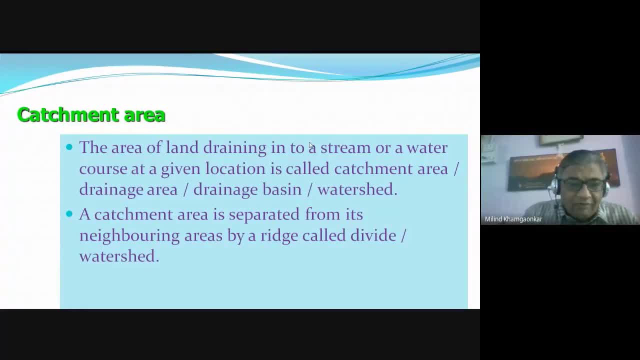 to consistency matters, the einenookie building, the best and the fastiest way. so to��서, we collaborate with the Hy dashboard in your home and this problem, we all agree with that, and you will ask us this question: when can we adjust it? when you about one of the term called as the catchment area, the water, the 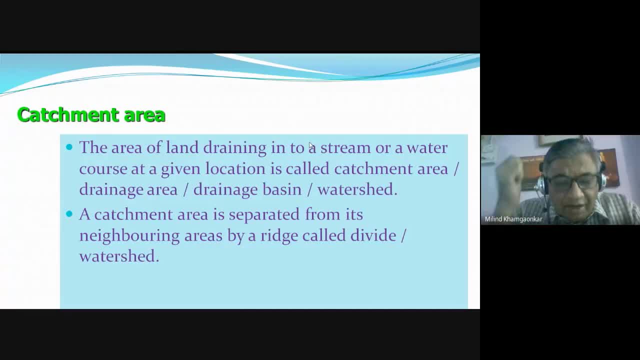 precipitation after falling over the land. the part of the precipitation which falls over the land to a certain area which supplies 100% water. that is the surface as well as the surf. subsurface runoff as well as the base flow, that is the groundwater flow, groundwater runoff, that part or that area which supplies. 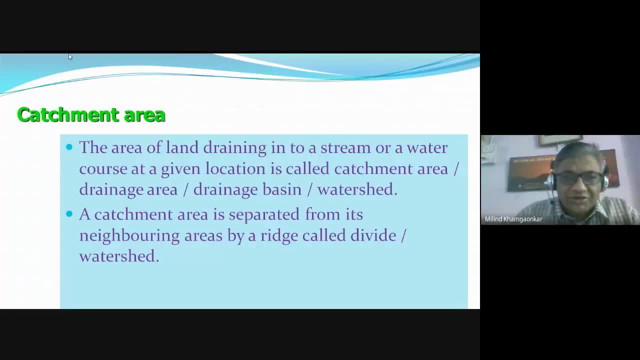 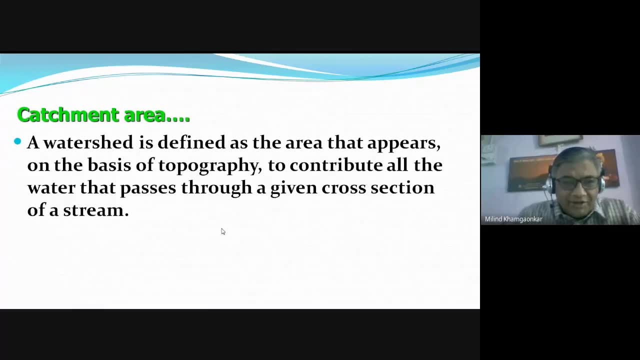 water to certain stream is called as the catchment area. the catchment area is separated by the Regis. the catchment area or watershed. it is also called as. it is also called as the drainage basin. it is defined as the area that appears on the basis of the topography to 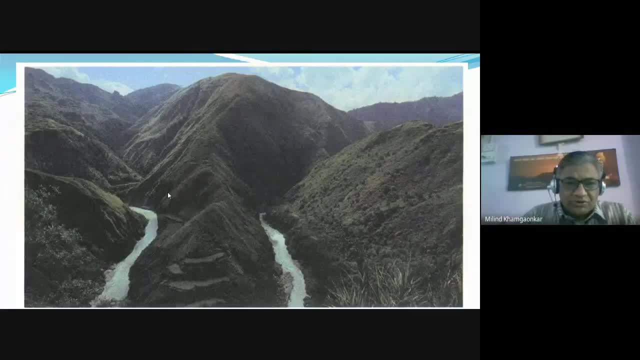 contribute all water that passes through the given cross section to the stream. I always show this picture to distinguish the catchment area. this is the reach. as I have told you just now, this region divides the catchment area of this stream as well as this stream that is. the catchment area is nothing but all. 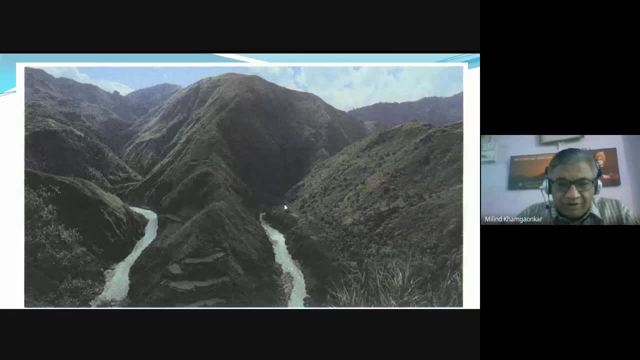 this area, between this reach and this stream, this reach for this stream, over which, when the rainfall occurs, the water reaches to this stream, as well as for this stream also, this reach and this, all these reaches in between all the area over which the rainfall occurs, it reaches. 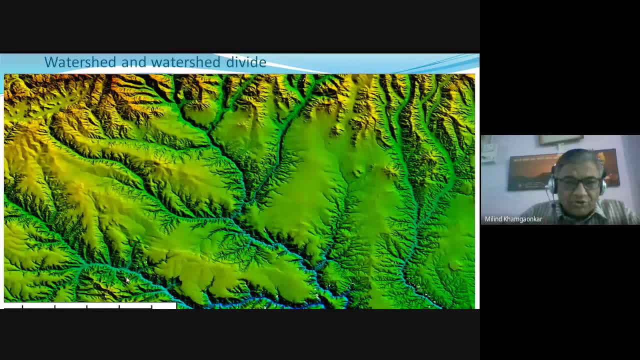 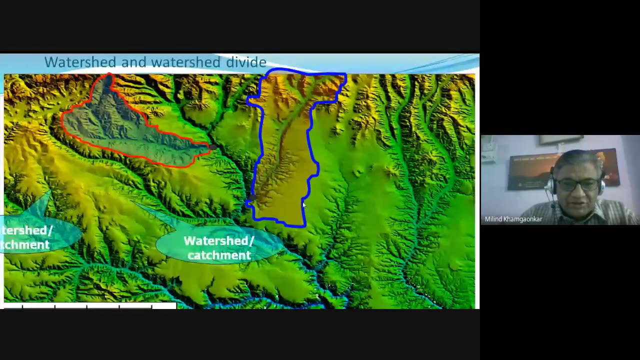 to the stream. I also show this media presentation to understand the catchment areas, as has been shown by this red color and the blue color boundary lines. that is, the watershed or catchment area of this stream. watershed and catchment area of this stream. various types of the catchment areas are there: fan shaped. 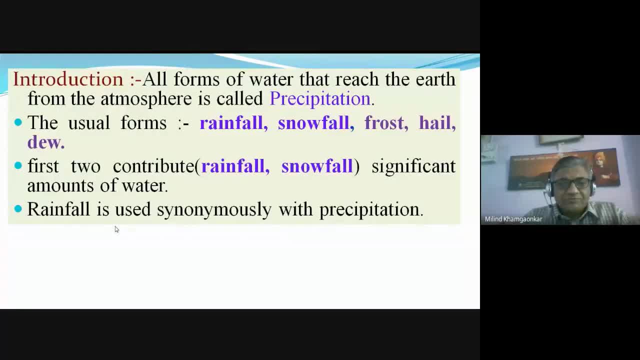 catchment area for leaf shaped catchment area. then we will move on to the next part, that is, the precipitation. as I one of the important component of the precipitation, as I one of the important component of the hydrologic cycle, that is, the precipitation in our precipitation is. 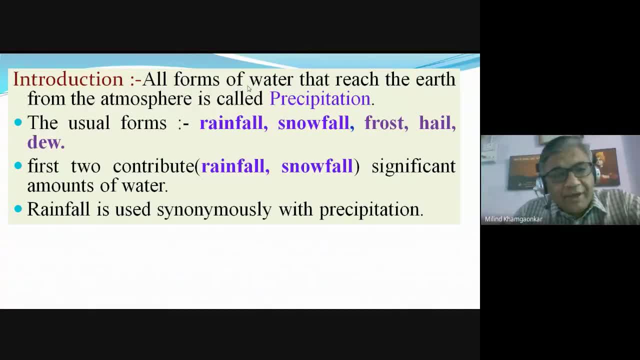 nothing but the all forms of the water may be a liquid form, may be a gaseous for vapor form, or maybe a solid form, that is, the ice form that reaches the earth from the atmosphere is called as the precipitation. the usual forms of the water which falls or which reaches the earth from the 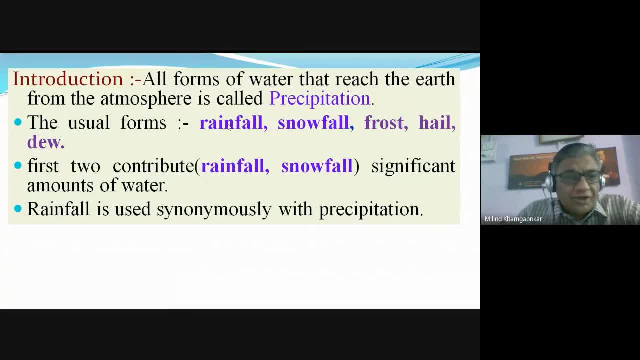 atmosphere to the land are the rainfall, which we regularly experience in our area, the snowfall, the frost, the hell and the deuce. okay, frasco, home in the may- yeah, Marathi may, but he may was- could do kakar cable. they took a hell means he is kumar at him a. garp it with you to school hell. 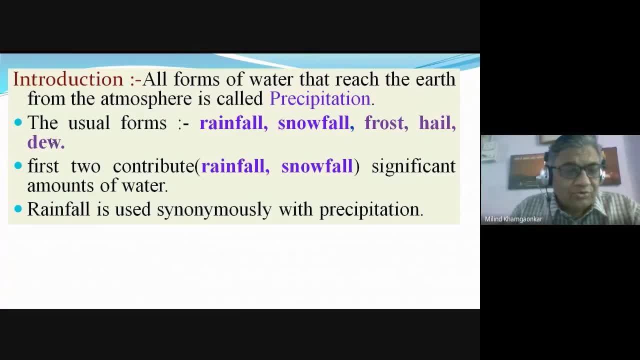 multi, or abuse, of course, of kumar luma, key to the vapor particles, which gets converted into very small, tiny water particles. they are called as the deuce. the first two, that is, the rainfall and the snowfall, contribute to largest quantity or amount of water that has been available that is being made. 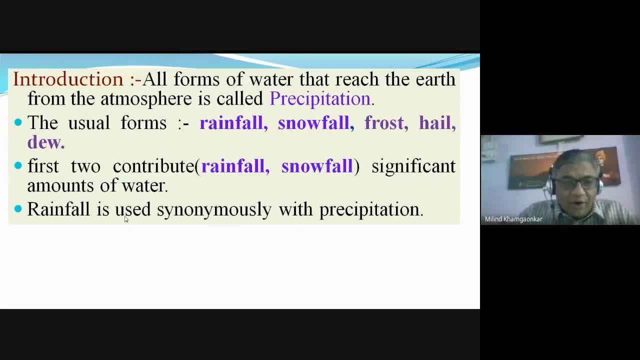 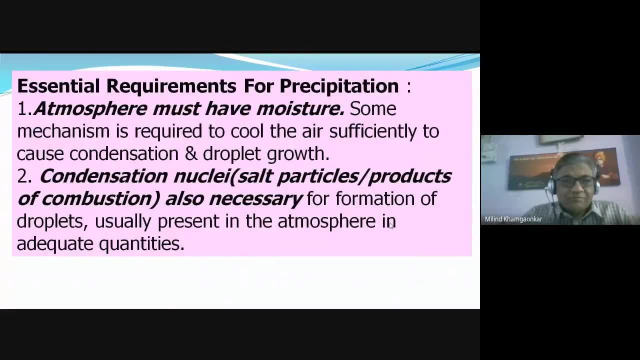 available on the earth and rainfall is considered, or is usually called as precipitation in our region. the essential requirements of the precipitation are the rainfall and the atmosphere must have moisture. okay, the atmosphere must have moisture. moisture means we have water vapor, water vapor concentration. so more water vapor concentration, more are the chances of occurrence of the. 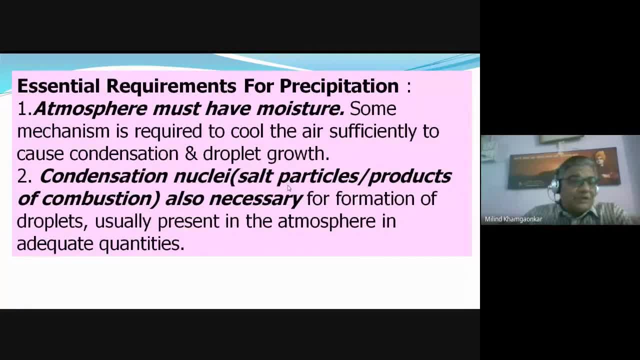 precipitation, condensation nuclei is very important a thing which is needed for the precipitation or the rainfall. this condensation nuclei are nothing but the very micro salt particles, are certain particles which are products of the combustion or maybe are part of certain lightening. or you can say: 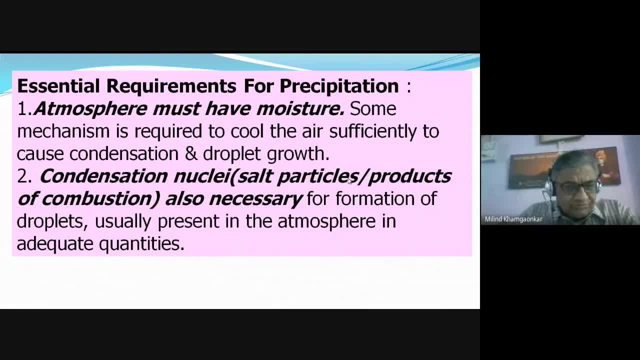 very micro or tiny particles of the dust. these are very necessary for the rainfall to occur, because the rain drop, or the water particles- Adidas to these salt particlesnymph, ignorance to these salt particles or to this dust particles guest park, You Are All Exactly On Series되- predominantly someulk into the retreat of the interest of the sought parts. theseстве I am sure that we will be make just that. this cools more. that carries the scale of geolocation and these particles, or so that these Internals are sitting, say we were very אותו yogi. 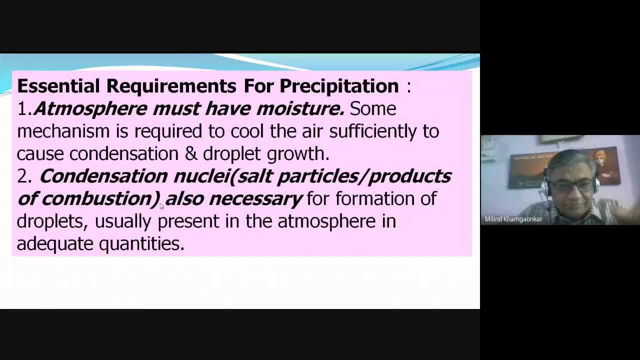 of these Suburban and geological phenomena in the region. a green teach education forecasting to add wood products from as a fast through the my teacher climb into information, they may become bigger and bigger. as they become large, then, and only then, they become heavier than the air or the wind and then, with the help of the 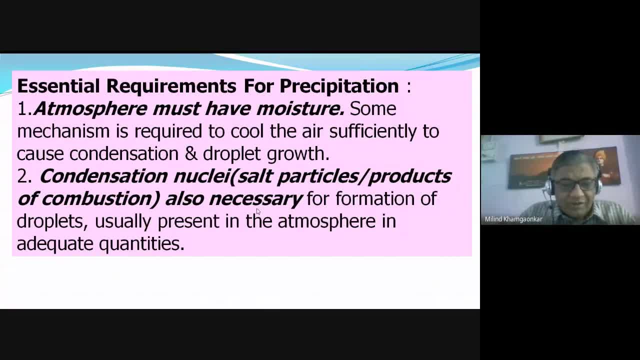 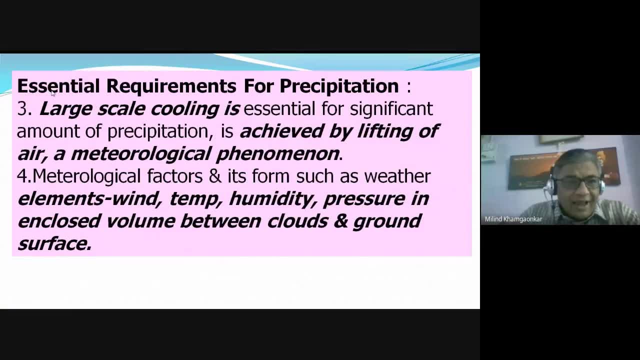 gravity they reaches to the earth. so therefore condensation nuclear is the must to form the droplet. larger scale cooling is also one of the requirement. unless and until the cooling app appears, the conversion of the water vapor particles into the droplets of water, as well as into the ice, could not. 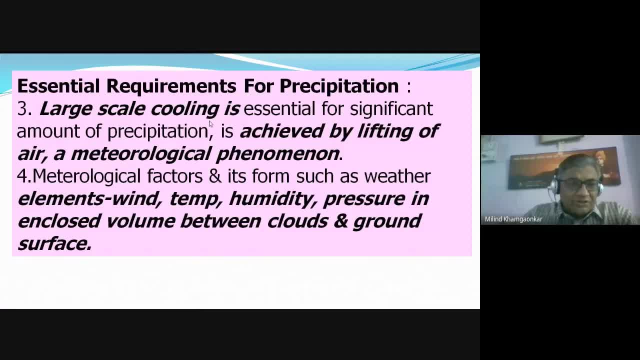 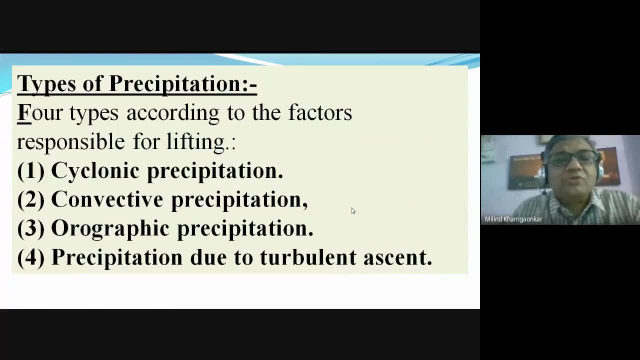 take place. so, therefore, cooling is necessary and other metrological factors, such as the wind, temperature, humidity, atmospheric pressure, etc. these are needed for the precipitation to occur. various types of the precipitation are there. they are the cyclonic precipitation, convective precipitation, orographic precipitation and precipitation due to turbulent acid. okay, we generally 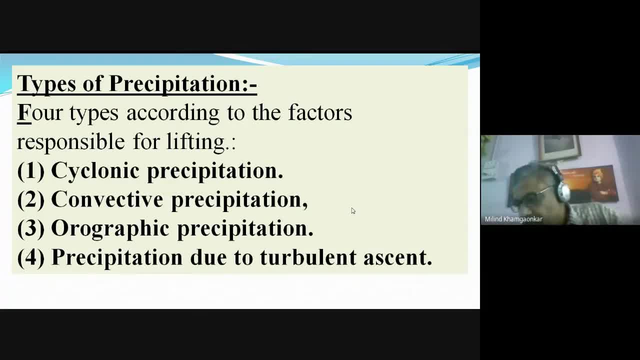 correlate precipitation to the rainfall. so the rainfall that occurs occurs on the earth or reaches to the earth by various processes. those various processes are divided or are called as the types of precipitation, various phenomena. they are the cyclonic, convective, orographic and the precipitation due to turbulent acid. 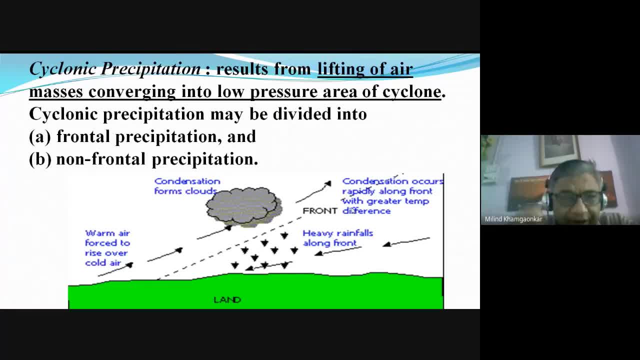 When the hot air along with the water vapor comes in contact or it flows from the water body, like the sea, and it reaches to the land and comes in contact with the cooler and the denser atmosphere, there is a front or a layer formed between the hot water vapor or the warm. 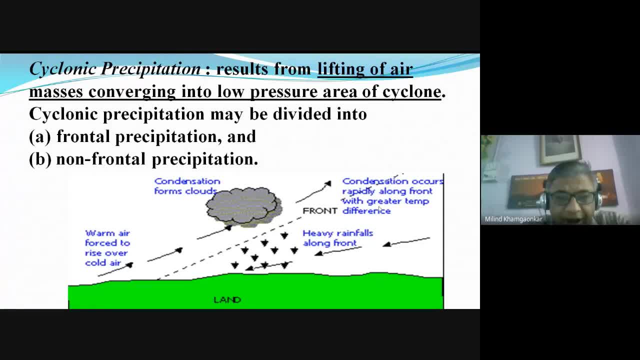 air and the cold air, and this front acts as a sliding plane and this hot air or warm air moves upwards, reaches to certain height where the temperature is higher, When the temperature is too cool, because, you know, almost with 1 Km rise above the earth, the 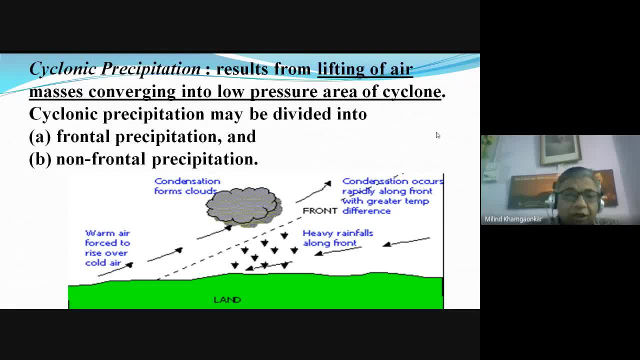 temperature reduces almost by 5 to 6 degrees. So as we move upwards, the temperature reduction is evident and therefore the cooler, more is the height from the earth, cooler is the atmosphere. So this warm air, along with the pressure of the water vapor, reaches to the temperature. and will come in contact with the water in the air, and this is the cold air. So, according to this, it is very cold air. it is very cold air So, as it moves up the temperature, when the temperature goes down, the temperature is higher. 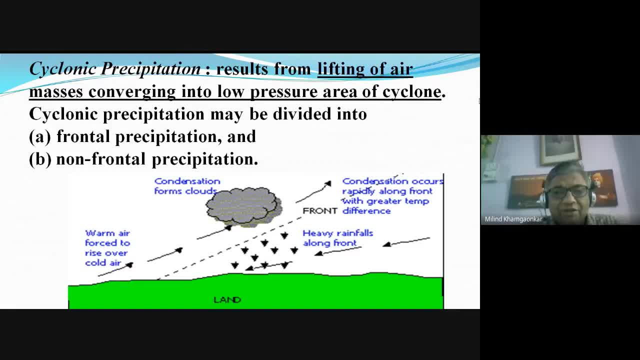 the water vapor reaches to that height and then converted into the water particle, and the phenomena of precipitation, that is, the fall of this water or the ice particle to the earth, occurs. this process is called as the cyclonic. this type of the precipitation is called as cyclonic precipitation. this 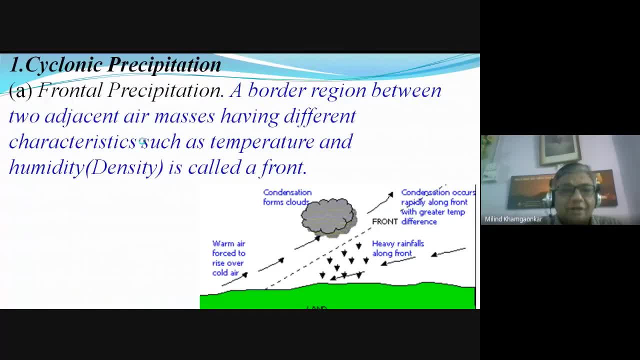 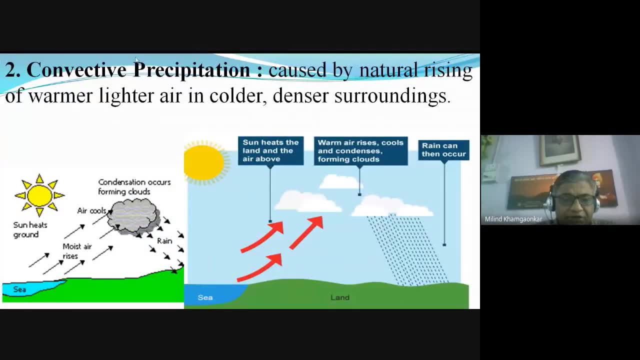 is further divided into frontal or non frontal precipitation. the next precipitation is called as the convective precipitation, wherein, again, the phenomena of reaching the warm air along with the water vapor or the clouds reaching to certain cooler height is there, and the precipitation is called as the convective precipitation where the 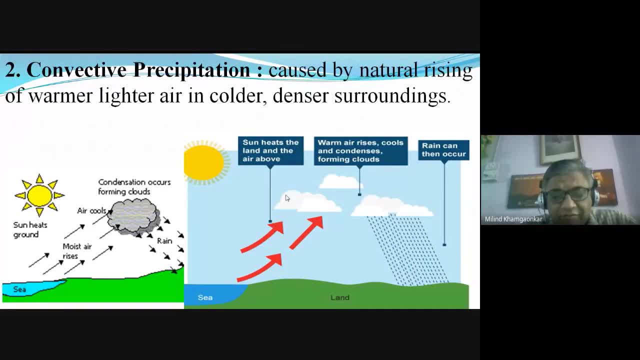 condenser and thezia rain. both take care of rain surface and comes forth and after cooling the condensed clouds converts into the rain. this is common in all the four types. only here no such France or frontal phenomena occurs as has been discussed earlier, but it is only due to natural rising of the warm light air in colder of theagensur. 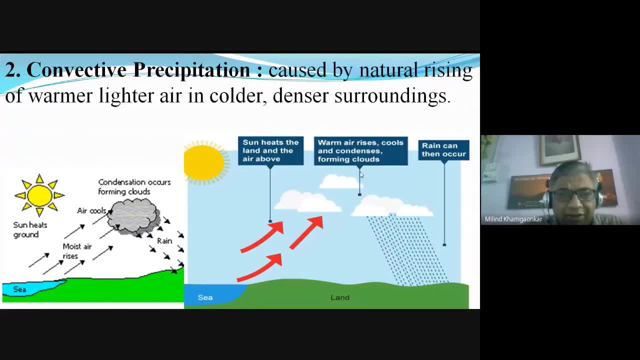 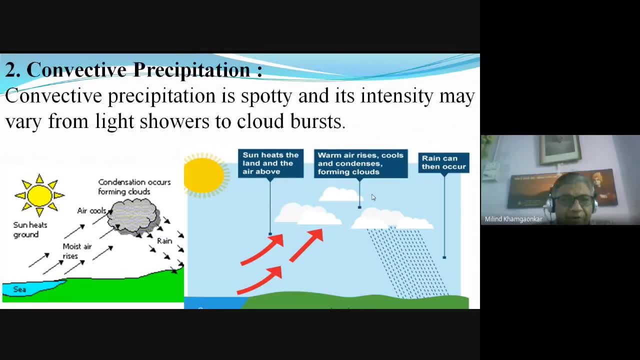 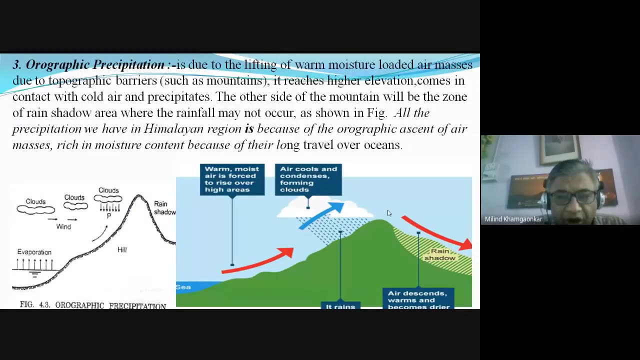 Natural resin And again the same condensation, cooling and the conversion. This is the convective precipitation. The next is orographic precipitation. This orographic precipitation occurs into the hilly area or into the mountainous area. So, as has been shown here, the clouds- it is also shown in this sketch also. the clouds moves towards the mountains And as the peak of the mountain is much higher, it is at much higher elevation that these clouds cannot cross to this peak. 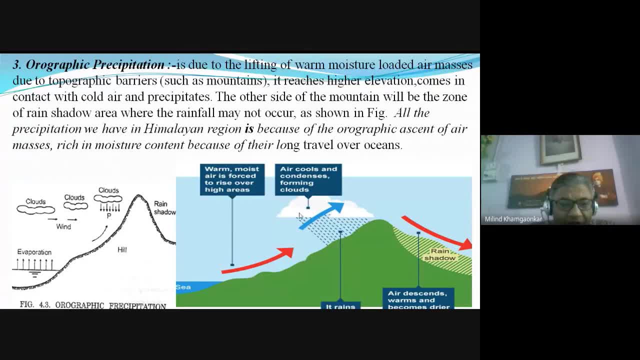 And therefore they get accumulated. They get accumulated before this mountain peak And after accumulation the condensation occurs And the condensed clouds which are bunched of the water vapor particles they get converted into, either to the water particles, raindrops, or to the ice particles. 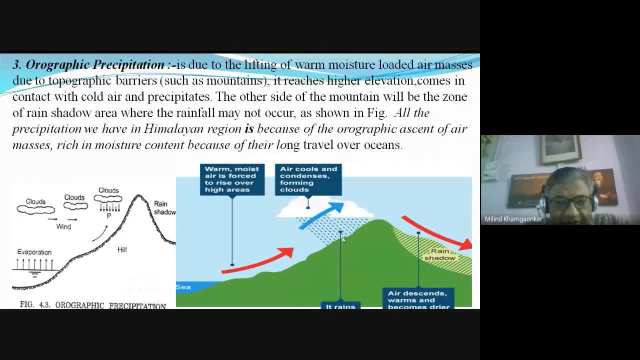 And they fall or they reach to the earth in the form of the precipitation. This is called as the orographic precipitation. In the Himalayan region northern region, as well as into the Sayadri ranges alongside the Kokand and the Kerala and some part of the Karnataka, the rainfall that occurs is due to this orographic precipitation. 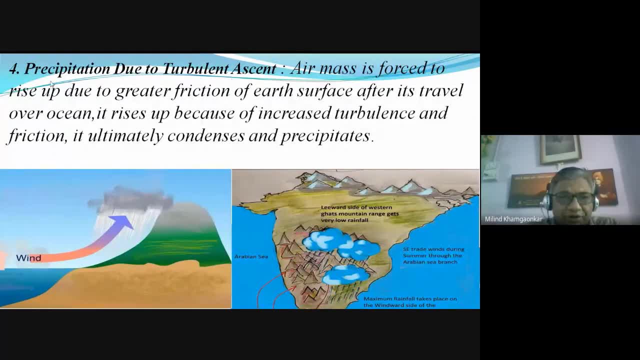 And last but not the least is precipitation due to turbulent ascent, Sometimes again due to the atmospheric changes, formation of the turbulent air movement. the warm air gets lifted over the cold air part due to the atmospheric movement, like the hurricanes, etc. and due to this turbulence the rainfall occurs. that rainfall is called. 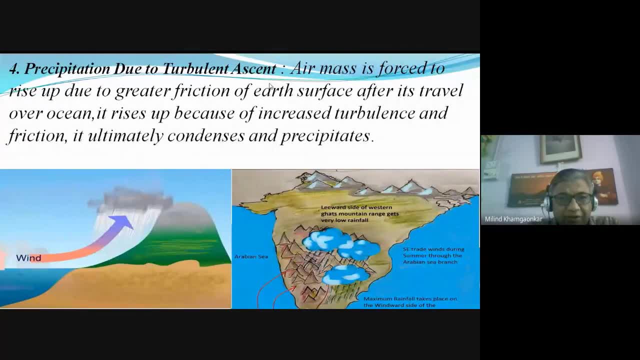 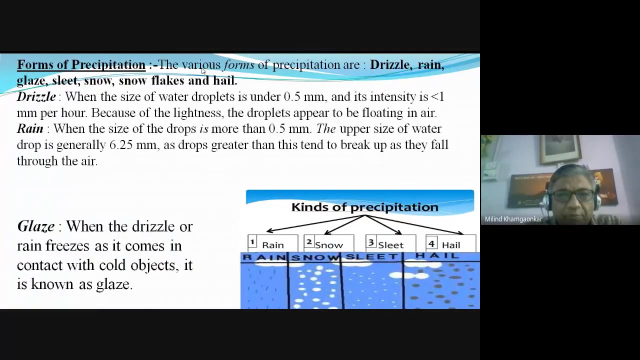 as the precipitation due to turbulent acid, whatever rainfall that occurs due to the hurricanes. that rainfall occurs as a result of this turbulent acid. various types or various forms of the precipitation are the drizzle, rain, glaze, sleet, snow, snowflakes and the hail. okay and result. these are: 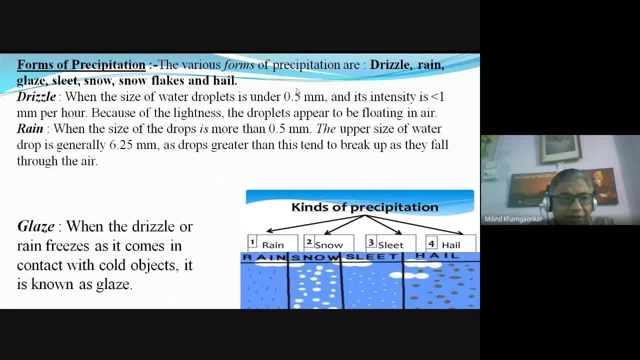 the various types you can see of the precipitation. drizzle means very small water droplets which falls over the earth. they are less than 0.5 mm diameter and the intensity is 1 millimeter per hour. rain, rainfall, as we call. the raindrops are more than 0.5. 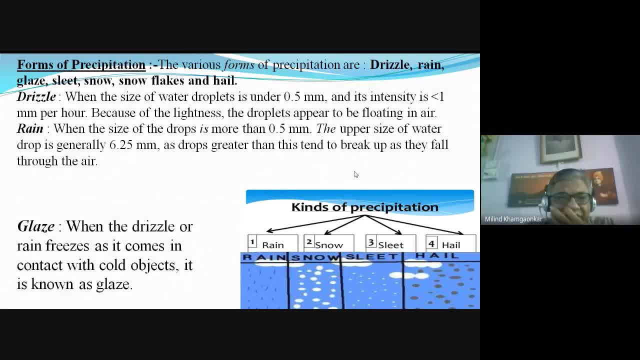 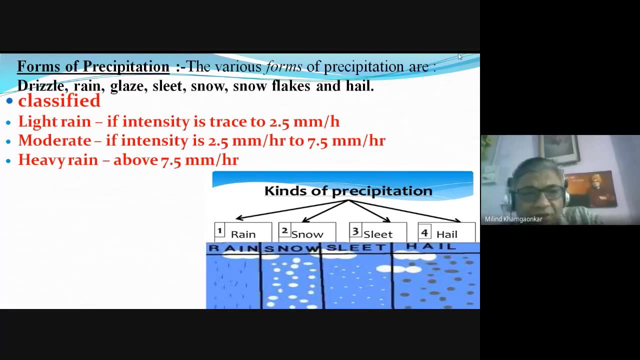 millimeters diameter. the intensity is also more than 1 millimeters per hour. when the drizzle or the rain freezes and gets converted into the ice flakes, it is called as the glaze. the rain is also further divided, or the precipitation. rainfall is further divided into three. 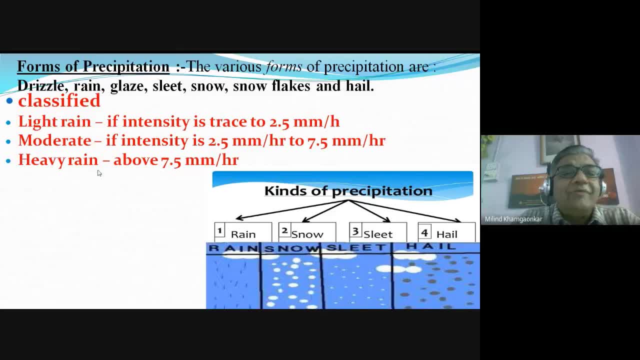 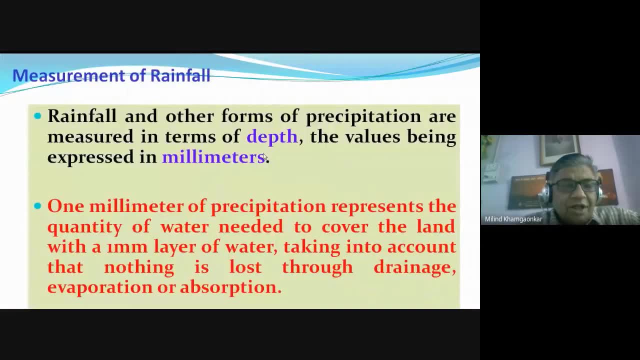 part, that is, the light rain, moderate rain, heavy rain, again depending of, depending on the rainfall intensity. now the measurement of the rainfall, as all this rainfall is converted as the glaze is converted as the snowfall, now the measurement of the rainfall and all these hydrological cycle and the hydrological events are very much important for us. 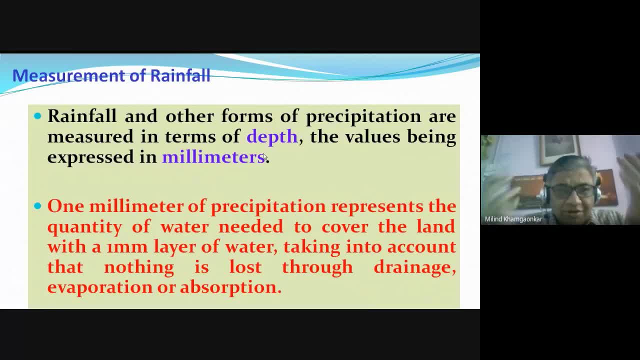 from the point of view of the design of hydraulic hydraulic structures. therefore, the necessity to measure the rainfall, how much precipitation has occurred. so the rainfall is measured in terms of the depth and it is expressed in millimeters or in centimeters. one millimeter of the precipitation. 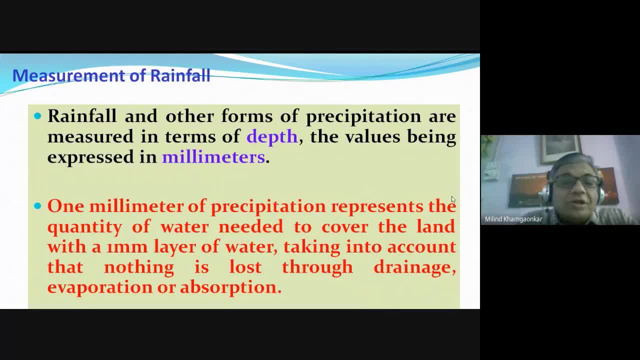 represents the quantity of water needed to cover the land with a 1 millimeter layer or thickness of water, taking into account that nothing is lying on that surface yet, this has to be always affected it. it is essential that no to drainage, evaporation or absorption. now how the rainfall is measured there. 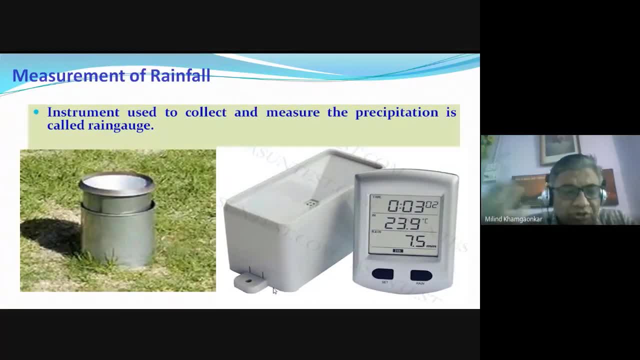 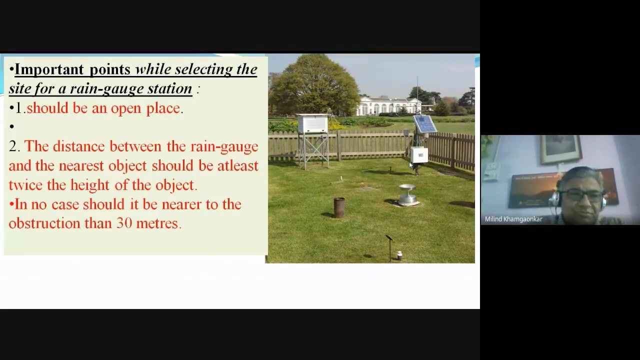 are various instruments which are used to measure the rainfall in again depth, that is, centimeters or the millimeter wherein the following rain, the precipitating water, is collected and is measured in terms of the depth in the equipments called as the rain gauges. there are very important aspects that 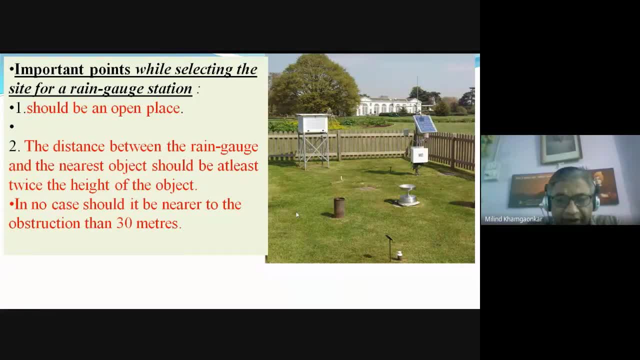 how to select the rain gauge station means where this rain gauge is to be installed. what is rain gauge station? rain gauge station is nothing but the location or the area wherein these rain gauges or rain fall measuring equipments are fixed. it should be in a open place that ring a station should be. 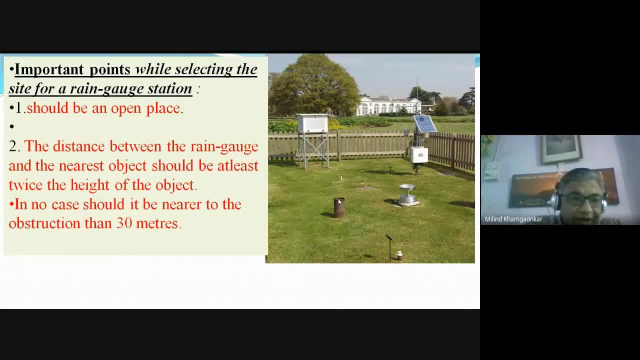 in open place, the distance between the rain gauge and the nearest object, like the tree or like the building, should be at location or the area wherein these rain gauges or rain fall measuring equipment least twice the height of the object means the distance between the rain gas station and the object that is like the tree or any building should be at. 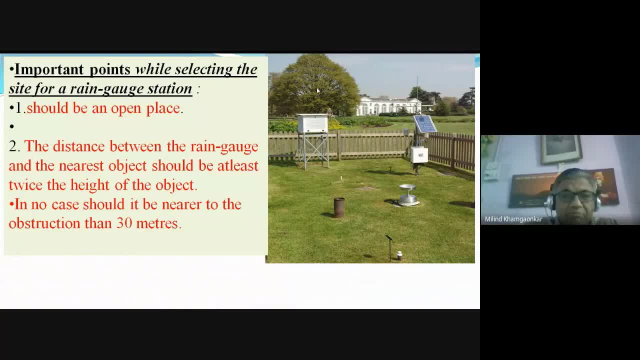 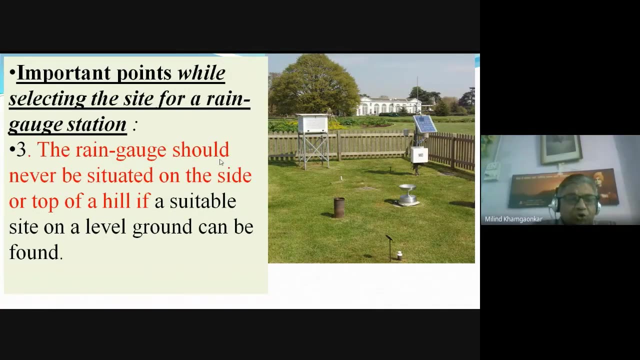 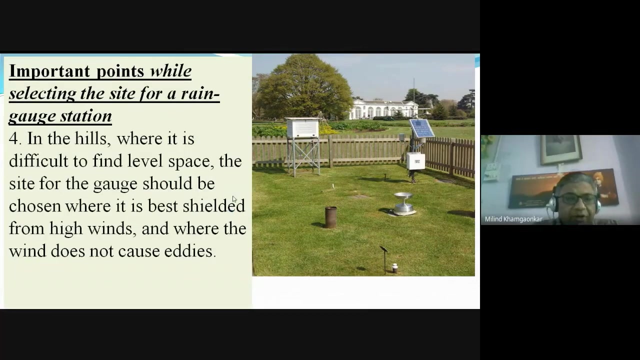 least more than double the height of the that object, that is, the tree or the building, but should not be in any case less than 30 meters. these meters say, come near energy. it should never be situated on the side of top of him. if we want to locate the rain gas station into at the hills, then as far as possible. 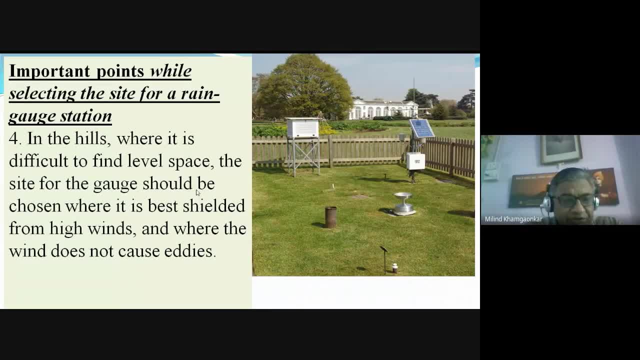 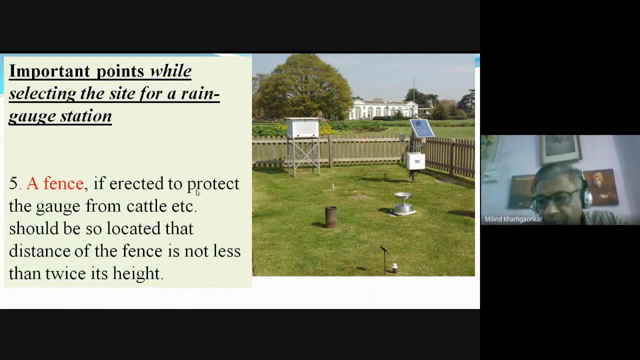 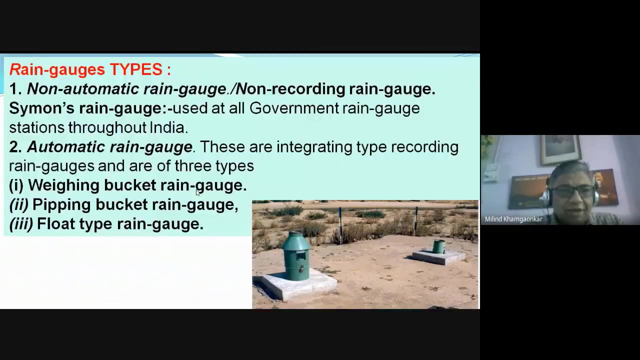 find the level place or level space, so that the ultimate thinking is that you, the rain falling or the precipitation occurring should not be obstructed. and, last but not the least, that all these rain gas stations must have a barricade or the compound or the fence, so that no external disturbance, either from the 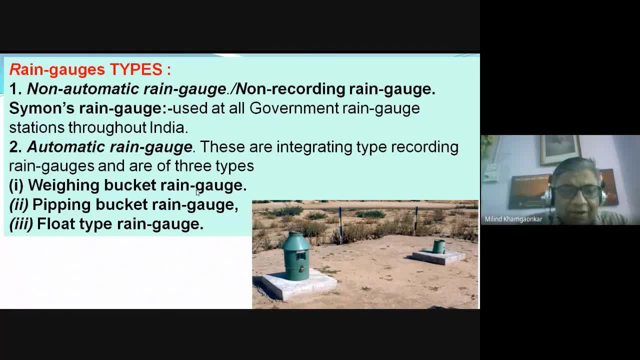 main, as well as the animal, should be there so that the accuracy in rainfall measurement should be there, so that the accuracy in rainfall measurement should be there, so that the accuracy in rainfall measurement will be affected. there are two types of these rain. gas stations are the rain. 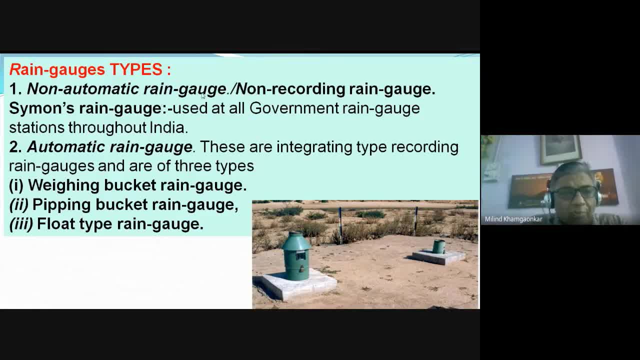 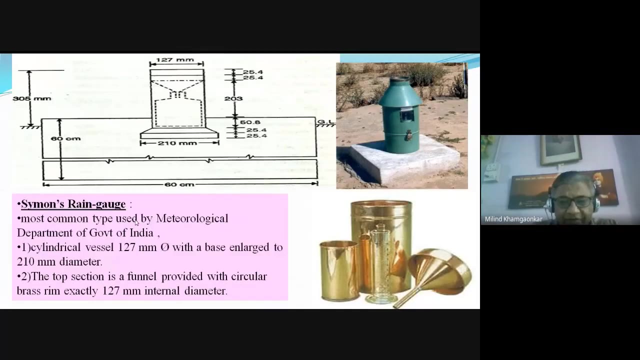 gauges. they are the automatic and non-automatic type. then in non-automatic type, the equipment or the rain gauge that is used is the Simon's rain gauge. in automatic rain gauges, the weighing bucket type the rain gauge, piping bucket, float type rain gauges- these are the various rain gauges- are there and the rain gauges are there. 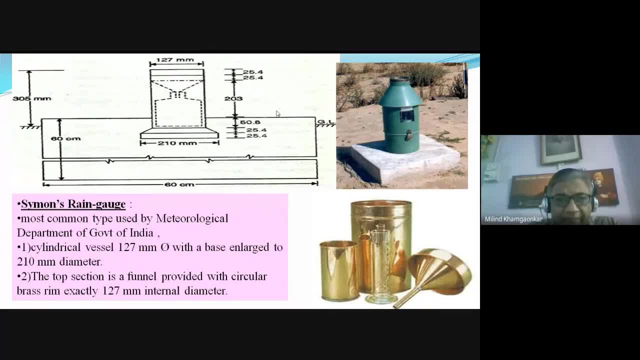 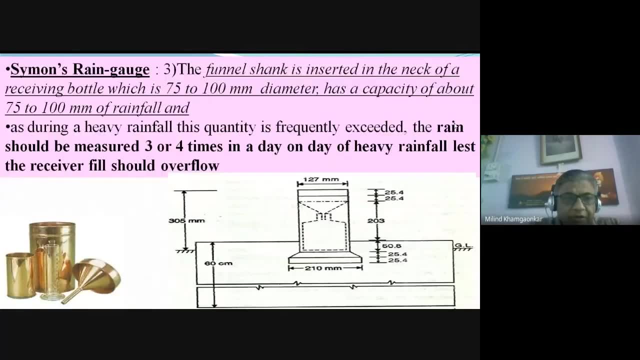 ok, this is the sketch of the Simon's or the non-automatic type rain gauge in our. ok. this is the sketch of the Simon's or the non-automatic type rain gauge in our India generally, this rain gauge being robust in nature, it is used all over the. 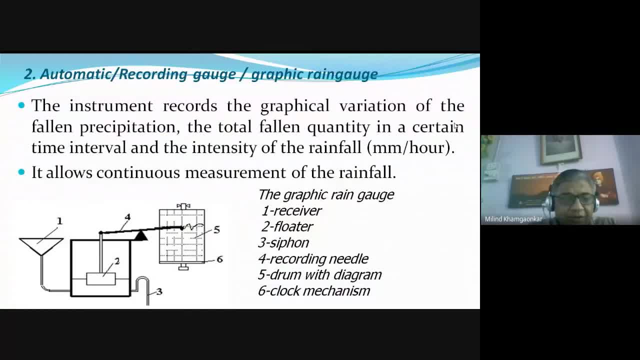 India generally. this rain gauge being robust in nature, it is used all over the Indian metrological rain gauge stations. now certain automatic or recording type Indian metrological rain gauge stations. now certain automatic or recording type. or the graphic rain gauge a. now certain automatic or recording type or the graphic rain gauge a. 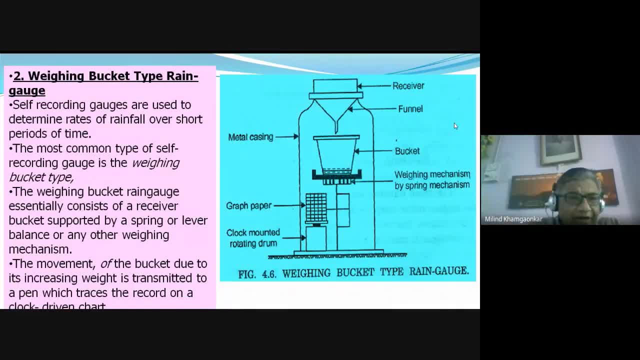 equipments are there. they are the weighing bucket type rain gauge wearing equipments are there. they are the weighing bucket type rain gauge wearing equipments are there. they are the weighing bucket type rain gauge wearing. the basic fundamental is the collected rain. the basic fundamental is the collected rain. the basic fundamental is the collected rain. either weighing bucket type tipping. 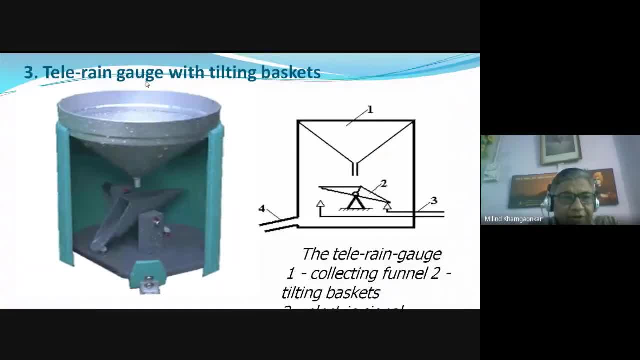 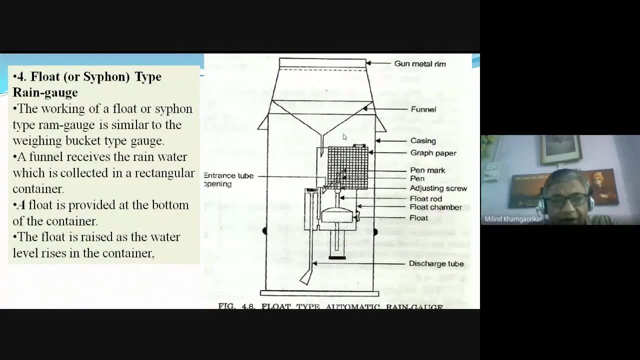 either weighing bucket type, tipping bucket type, or the third one is the float, or the third one is the float or the third one is the float. or the siphon type ringage. is there, the? or the siphon type ringage is there, the? or the siphon type ringage is there. the fundamental is the water or the rainfall. 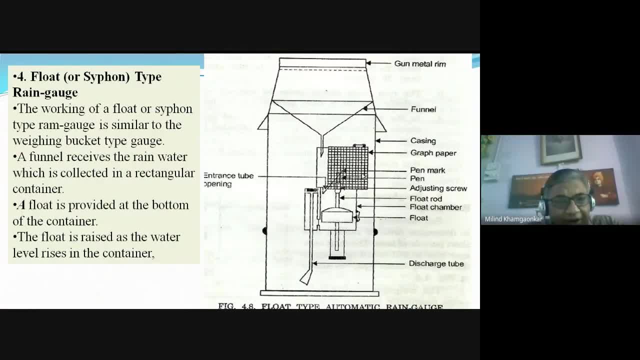 fundamental is the water or the rainfall. fundamental is the water or the rainfall, or the precipitation is being collected as, or the precipitation is being collected as, or the precipitation is being collected as, either into the weighing bucket or the, either into the weighing bucket or the, either into the weighing bucket or the tipping bucket, or into this float type in. 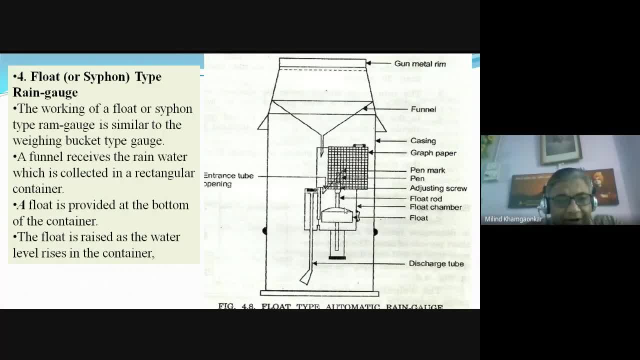 tipping bucket, or into this float type in tipping bucket, or into this float type in certain container, and that contained certain container and that contained certain container and that contained the water quantity is being calibrated with. the water quantity is being calibrated with. the water quantity is being calibrated with the help of certain graphs and the. 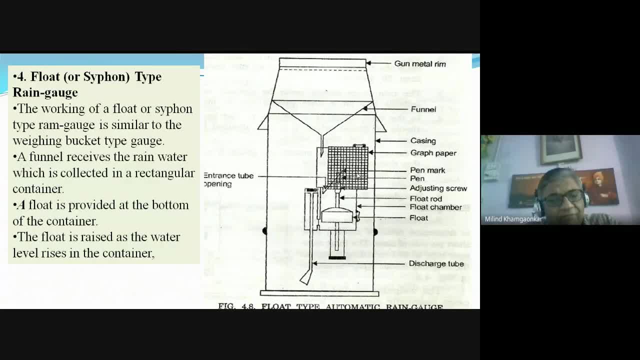 the help of certain graphs and the, the help of certain graphs and the pens continuously for the 24 hours, or maybe pens continuously for the 24 hours, or maybe pens continuously for the 24 hours, or maybe for the days together, so that there, for the days together, so that there. 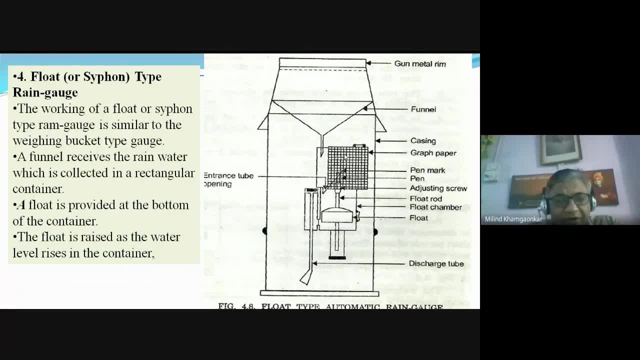 for the days together, so that there will not be any, will not be any, will not be any interference of the human or the animal and interference of the human or the animal and interference of the human or the animal, and we will get automatically the quantity. we will get automatically the quantity. 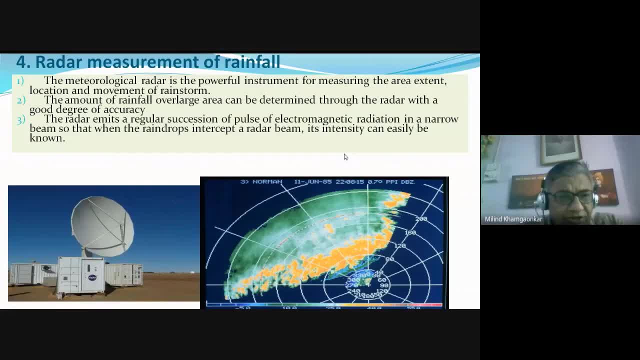 we will get automatically the quantity of the rainfall a large, but not the of the rainfall a large, but not the of the rainfall a large, but not the least. nowadays, the rainfall, or least nowadays the rainfall, or least nowadays the rainfall or precipitation, is also being measured with. 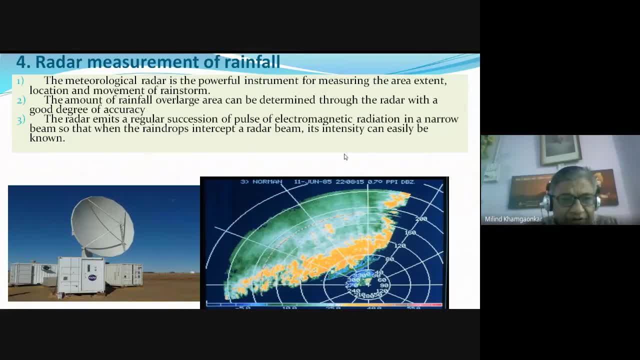 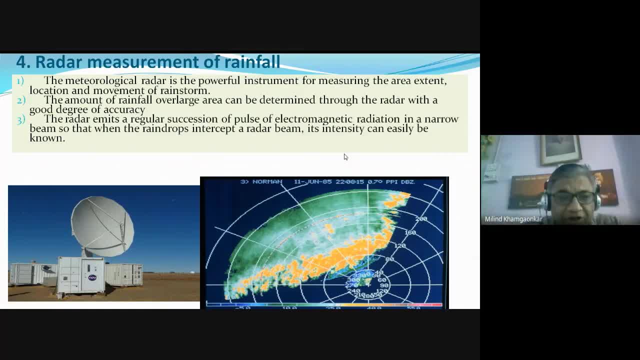 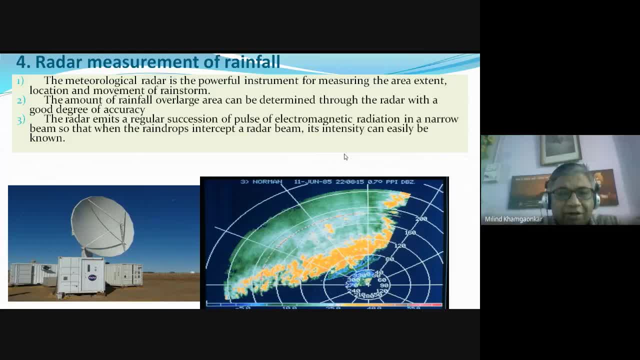 precipitation is being distributed. it also gives the intensity that at what also gives the intensity that at what also gives the intensity that at what intensity the precipitation is being intensity, the precipitation is being intensity, the precipitation is being occurring as well, as it also gives the occurring as well as it also gives the 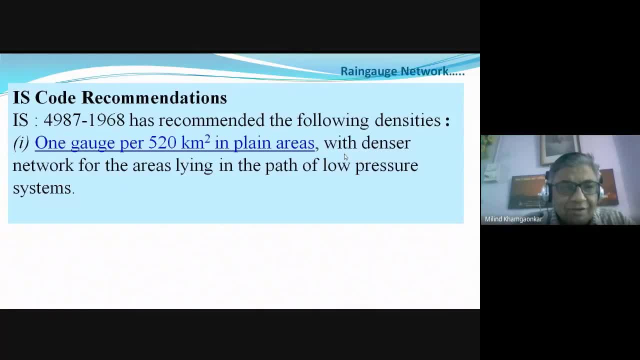 occurring, as well, as it also gives the quantity of the precipitation. how much quantity of the precipitation, how much quantity of the precipitation? how much rain gauge stations are to be provided? rain gauge stations are to be provided. rain gauge stations are to be provided in certain catchment area is being 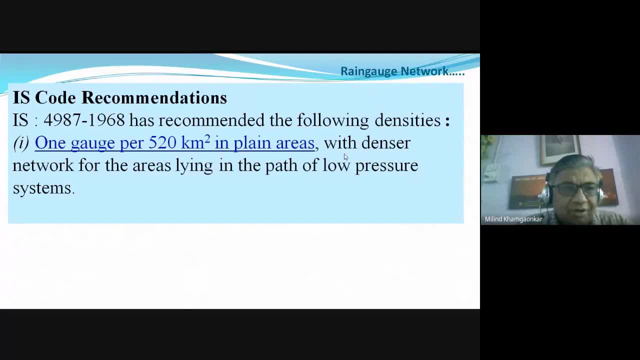 in certain catchment area, is being in certain catchment area, is being finalized, or the finalized, or the finalized, or the guidelines are being given by the Indian guidelines are being given by the Indian guidelines are being given by the Indian Standard Code or Bureau of Indian Standard Code or Bureau of Indian. 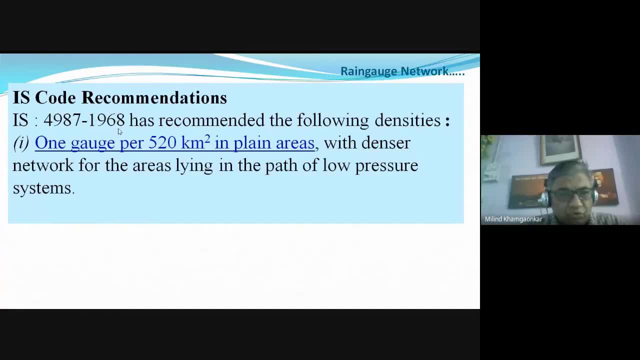 Standard Code or Bureau of Indian Standard Code: 4987 1968: okay. Standard Code 4987 1968: okay. Standard Code 4987 1968: okay. wherein they have said that for 520. wherein they have said that for 520. wherein they have said that for 520 kilometer square of the plain area after. 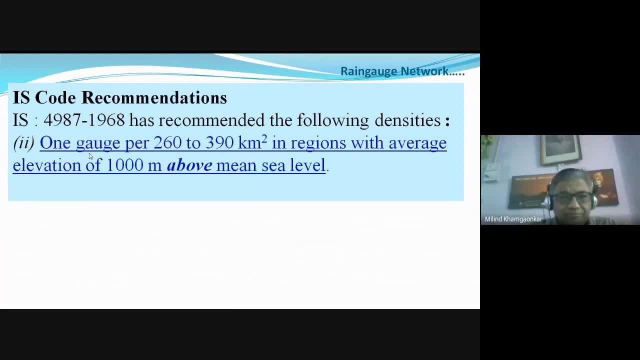 kilometer square of the plain area after kilometer square of the plain area after the catchment area. one rain gauge the catchment area after the catchment area. one rain gauge the catchment area after the catchment area. one rain gauge station can be provided for. 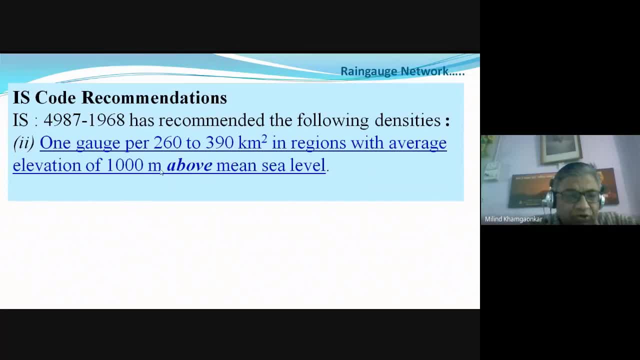 station can be provided for. station can be provided for the average in area which has got 1,000, the average in area which has got 1,000, the average in area which has got 1,000 meters and meters and meters and above height, for that 260 to 390. 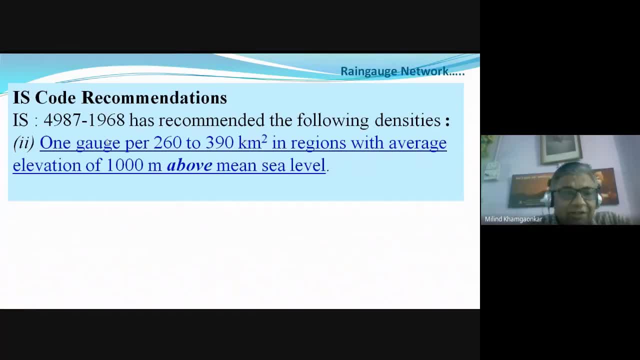 above height for that 260 to 390 above height. for that 260 to 390 kilometer square area or this area when kilometer square area or this area when kilometer square area or this area when they're engaged station can be provided, they're engaged station can be provided. 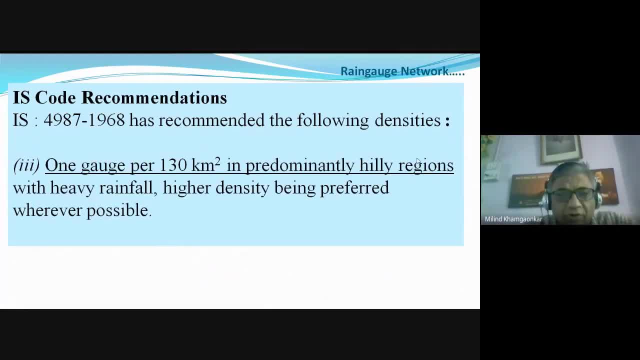 they're engaged, station can be provided, and for very hilly region- mountainous. and for very hilly region- mountainous. and for very hilly region- mountainous region, for 130 kilometer squares of the region, for 130 kilometer squares of the region, for 130 kilometer squares of the area, one rain gauge station should be. 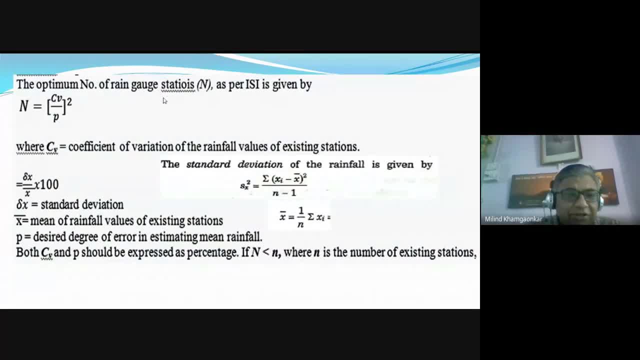 area one rain gauge station should be area one rain gauge station should be provided the optimum rain gauge stations provided the optimum rain gauge stations provided the optimum rain gauge stations to be provided in certain catchment area. to be provided in certain catchment area. to be provided in certain catchment area is given by the Indian standard. by this. 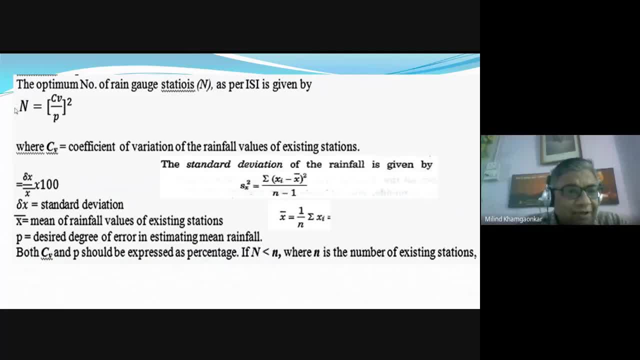 is given by the Indian standard, by this is given by the Indian standard, by this equation or by this formula, and that is equation, or by this formula, and that is equation, or by this formula. and that is the maximum number of rain gauge stations. the maximum number of rain gauge stations. 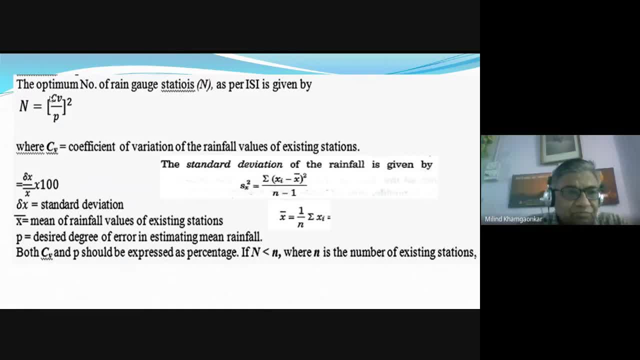 the maximum number of rain gauge stations is equal to coefficient of variation. is equal to coefficient of variation. is equal to coefficient of variation divided by the percentage of error in divided by the percentage of error in divided by the percentage of error in observation of the rainfall permitted. 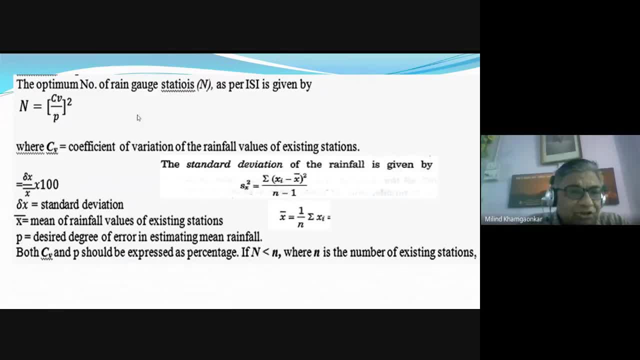 observation of the rainfall permitted. observation of the rainfall permitted. this ratio and if it is squared, the this ratio and if it is squared, the this ratio and if it is squared, the square of this ratio, will give you square of this ratio, will give you square of this ratio, will give you maximum number of the rain gauge stations. 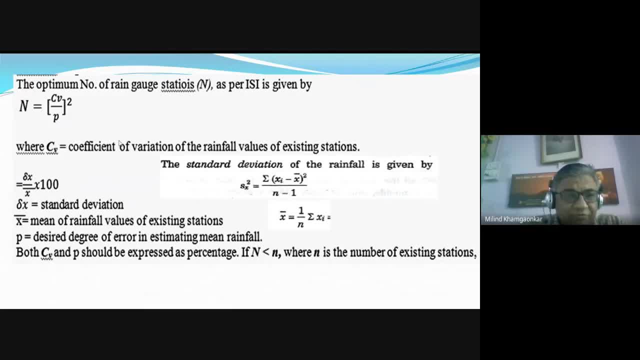 maximum number of the rain gauge stations. maximum number of the rain gauge stations that are provided, that are provided. that are provided into the catchment area. the coefficient of into the catchment area. the coefficient of into the catchment area, the coefficient of variation, is being found out by the: 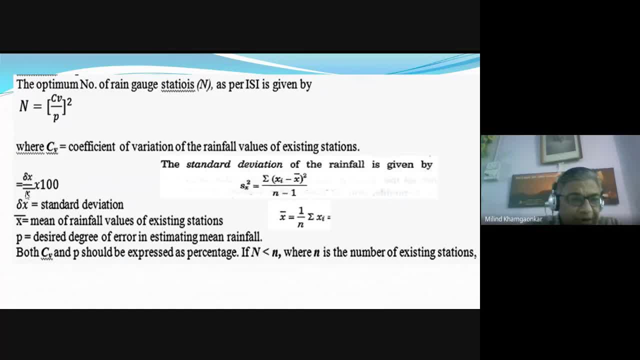 variation is being found out by: the variation is being found out by: the formula CV is equal to Delta X upon X bar. formula CV is equal to Delta X upon X bar. formula CV is equal to Delta X upon X bar into 100, wherein Delta X or S X is. 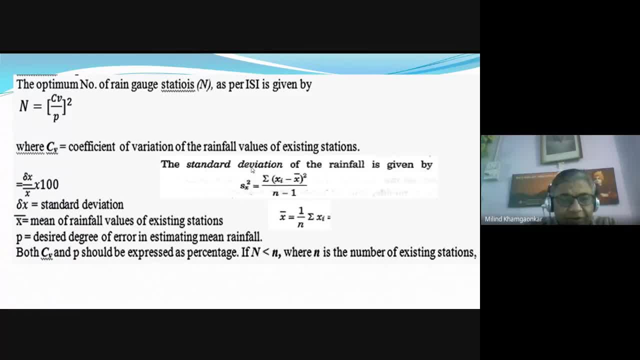 into 100, wherein Delta X or S X is into 100, wherein Delta X or S X is called as the standard deviation, the called as the standard deviation, the called as the standard deviation. the standard deviation is also given by. standard deviation is also given by. standard deviation is also given by certain formula. S X square is equal to X. 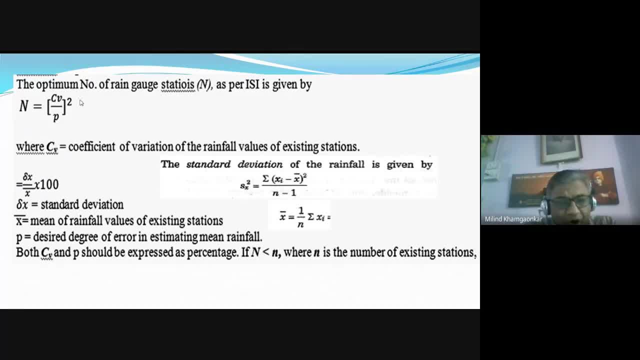 certain formula S X square is equal to X. certain formula S X square is equal to X minus X bar whole square upon n minus minus X bar whole square upon n minus minus X bar whole square upon n minus. so all this procedure is being adopted. so all this procedure is being adopted. 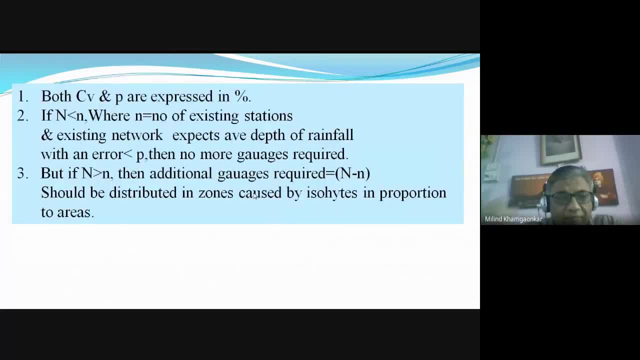 so all this procedure is being adopted based on the number of the existing rain. based on the number of the existing rain, based on the number of the existing rain gauge stations and whether additional gauge stations and whether additional gauge stations and whether additional rain gauge stations are needed to find. 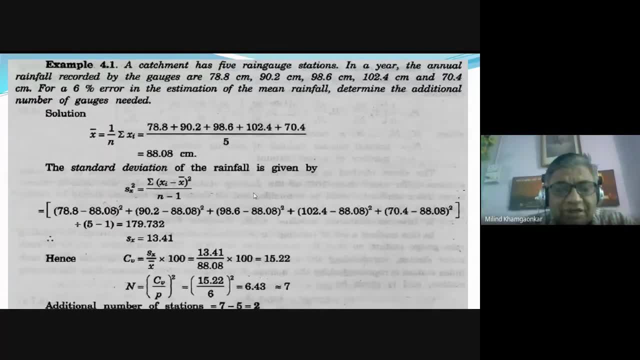 rain gauge stations are needed to find rain gauge stations are needed to find out the exact quantity of the rain. gauge out the exact quantity of the rain gauge out the exact quantity of the rain gauge into the certain catchment area. because into the certain catchment area, because 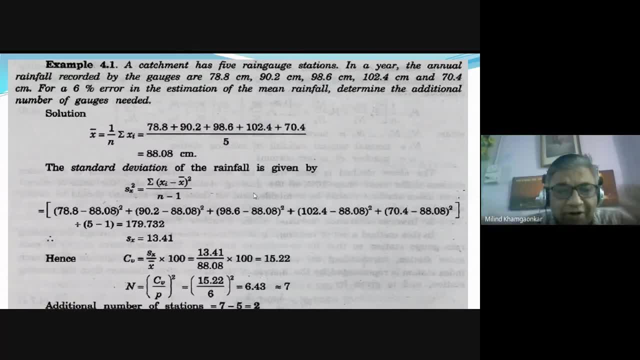 into the certain catchment area because, friends, the exact quantity calculation, friends, the exact quantity calculation, friends, the exact quantity calculation of this rainfall is very of this rainfall is very of this rainfall, is very important from the point of view of finding, important from the point of view of finding. 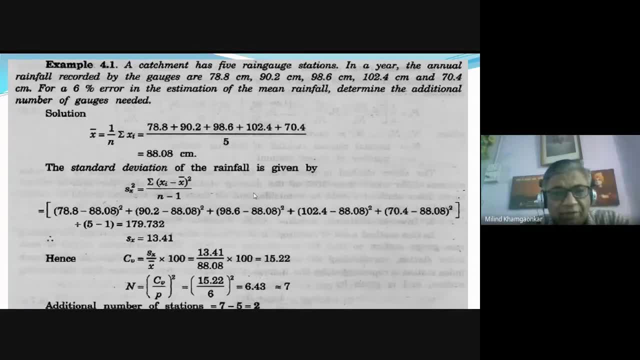 important from the point of view of finding the exact quantity of the runoff. the exact quantity of the runoff, the exact quantity of the runoff, which is very important from the point of which is very important, from the point of which is very important from the point of view of designing the hydraulic 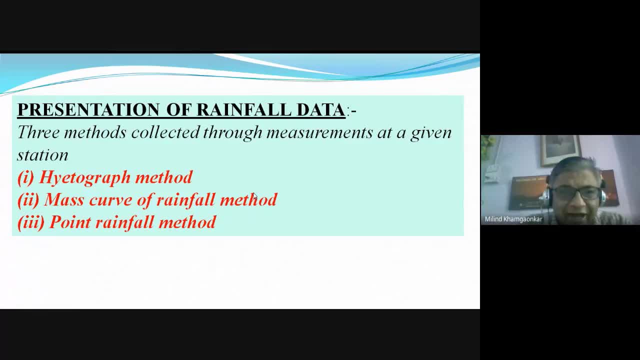 view of designing the hydraulic view of designing the hydraulic structures. this rainfall data may be structures. this rainfall data may be structures. this rainfall data may be available for one day. may be available. available for one day. may be available. available for one day. may be available for one week. may be available for one. 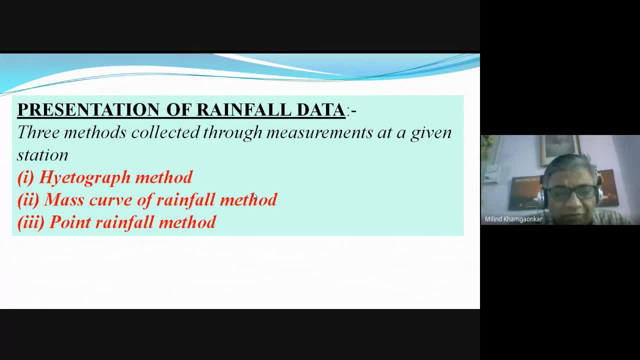 for one week may be available for one for one week may be available for one month. one year or four hundred years or month. one year or four hundred years or month. one year or four hundred years or four twenty fifty years is being four. twenty fifty years is being. 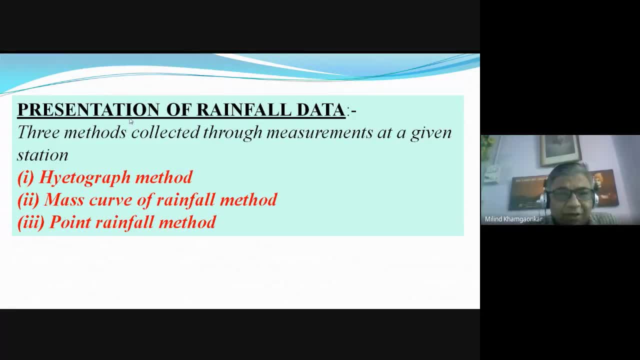 four, twenty, fifty years is being reported or is being prepared in various reported, or is being prepared in various reported, or is being prepared in various forms. that is called as the forms, that is called as the forms, that is called as the presentation of the rainfall. they are: 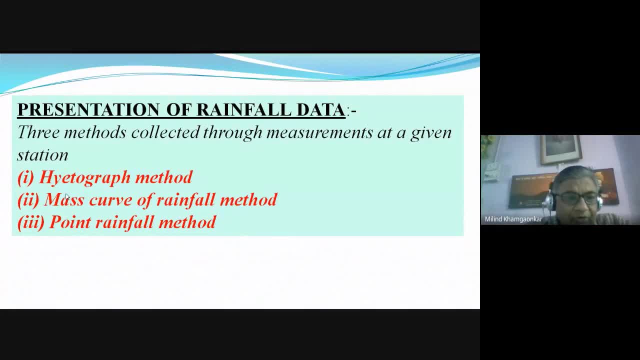 presentation of the rainfall. they are presentation of the rainfall. they are either presented in hydrograph form or either presented in hydrograph form, or either presented in hydrograph form or hydrograph method. mass curve of the hydrograph method. mass curve of the hydrograph method. mass curve of the rainfall point. rainfall method. these are: 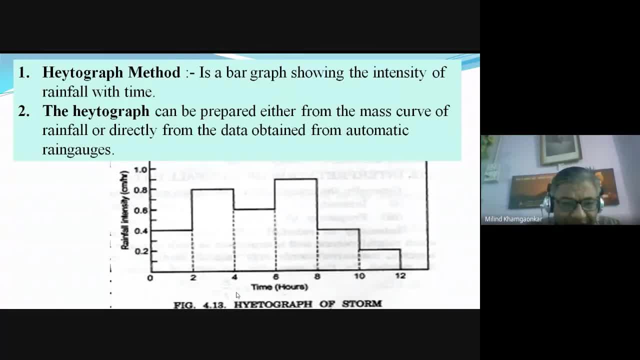 rainfall point, rainfall method. these are rainfall point, rainfall method. these are the various methods. I to graph is very. the various methods. I to graph is very. the various methods. I to graph is very important. it is the graph between the important. it is the graph between the important. it is the graph between the duration may be in center, may be in. 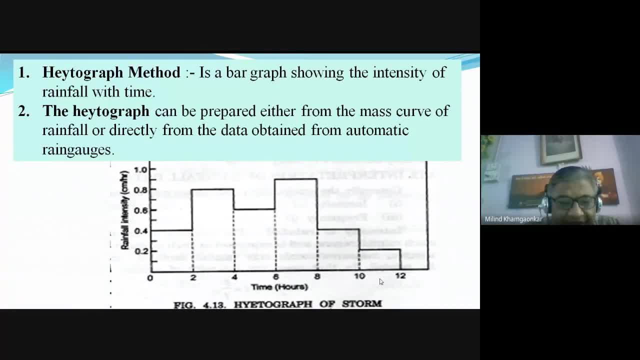 duration: may be in center. may be in. duration may be in center. may be in seconds. minutes hours, weeks days, month seconds minutes hours, weeks days. month seconds minutes hours, weeks days, month. year to rainfall intensity. this graph is year to rainfall intensity. this graph is year to rainfall intensity. this graph is called as the hydrograph there the. 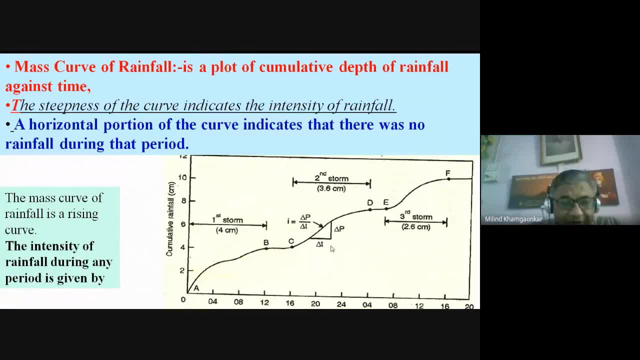 called as the hydrograph there, the called as the hydrograph there. the another very important is mass curve of another very important is mass curve of another very important is mass curve of the rainfall. again it is the curve, the rainfall, again it is the curve, the rainfall, again. it is the curve between the duration and cumulative. 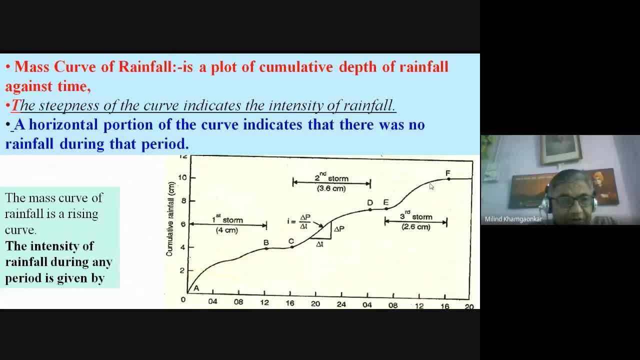 between the duration and cumulative, between the duration and cumulative rainfall. so this is very important, the rainfall, so this is very important, the rainfall, so this is very important. the third is point rainfall method. let third is point rainfall method. let third is point rainfall method. let is be rainfall from the individual. 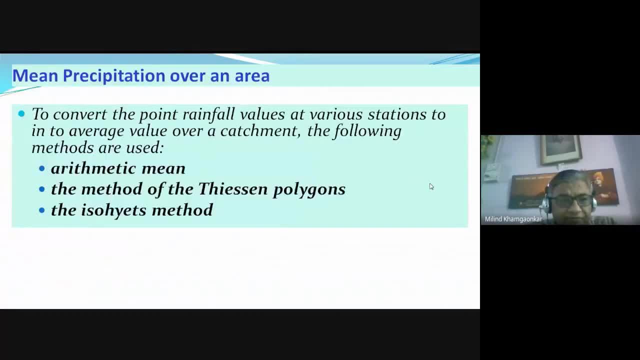 is be rainfall from the individual is be rainfall from the individual. rain gauge station maintained daily. rain gauge station maintained daily. rain gauge station maintained daily, then for finding the average rainfall, or then for finding the average rainfall, or then for finding the average rainfall or precipitation over a certain area. there. 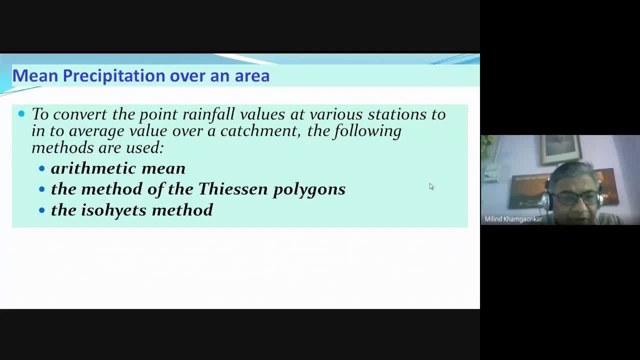 precipitation over a certain area. there. precipitation over a certain area. there are three methods. they are called as the are three methods. they are called as the are three methods. they are called as: the arithmetic mean method, method of the arithmetic mean method, method of the arithmetic mean method, method of the Thyssen polygon and I saw height method. 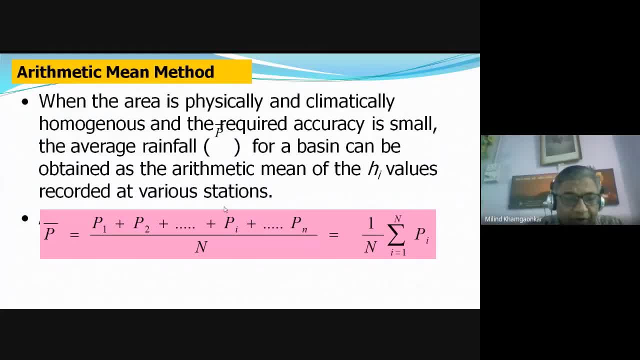 Thyssen polygon and I saw height method. Thyssen polygon and I saw height method in arithmetic method. whatever number in arithmetic method, whatever number in arithmetic method, whatever number of the rain gauge stations, we have of the rain gauge stations, we have of the rain gauge stations. we have, that is, capital N and the precipitation. 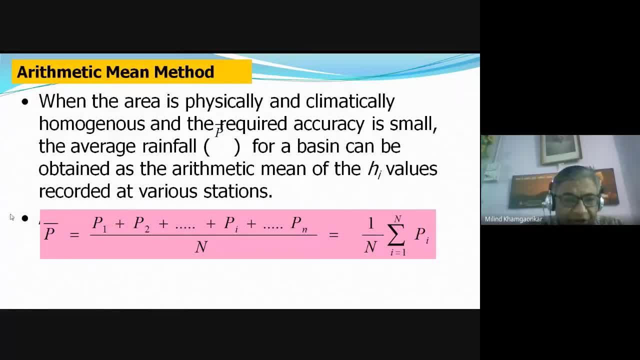 that is capital N and the precipitation that is capital N and the precipitation data from those rain gauge stations. for data from those rain gauge stations for data from those rain gauge stations for a certain duration or period is added. a certain duration or period is added. a certain duration or period is added and divided by the number of the rain. 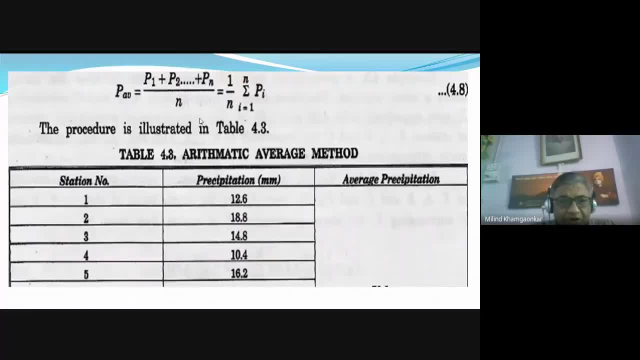 and divided by the number of the rain. and divided by the number of the rain gauge stations, will give you the average gauge stations, will give you the average gauge stations will give you the average precipitation over certain catchment area. precipitation over certain catchment area. precipitation over certain catchment area. now another method is Thyssen's polygon. 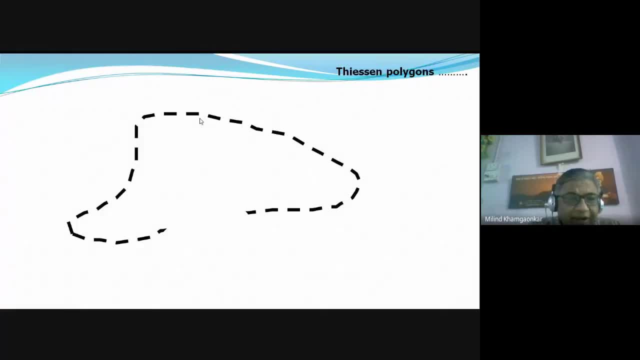 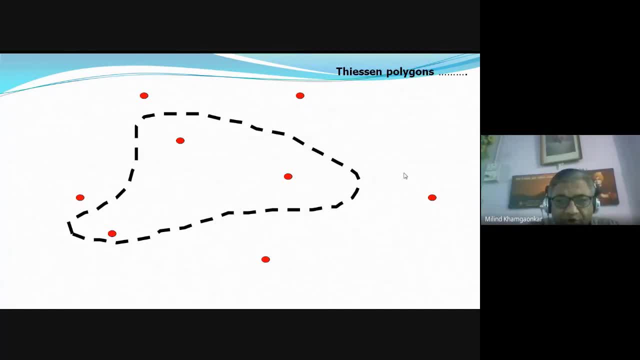 subdivided based on the weightage given to the rain gauge stations, as has been the rain gauge stations, as has been the rain gauge stations, as has been shown here by the red dots and the shown here by the red dots and the shown here by the red dots, and the catchment is shown by the dotted line. so 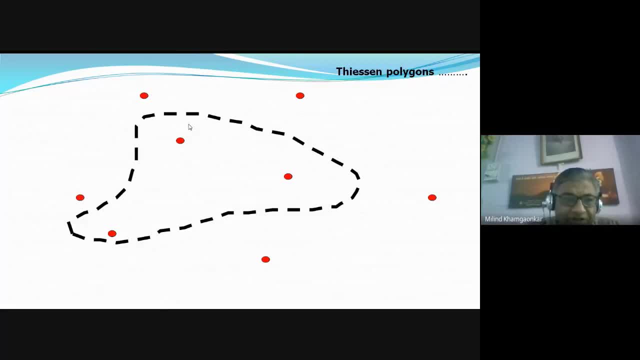 catchment is shown by the dotted line. so, catchment is shown by the dotted line. so, for all these rain gauge stations, or for all these rain gauge stations, or for all these rain gauge stations or rain measuring stations, which area is rain measuring stations? which area is? rain measuring stations. which area is being important from that being important, from that being important from that rain gauge stations. that is called as the rain gauge stations. that is called as the rain gauge stations. that is called as the weighing of the area is being done by. weighing of the area is being done by. 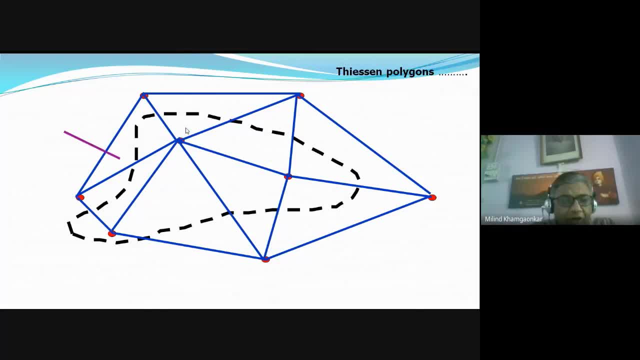 weighing of the area is being done by certain scientific method, wearing all certain scientific method, wearing all certain scientific method, wearing all those are joined their perpendicular. those are joined their perpendicular, those are joined their perpendicular. bisectors are drawn. they are connected. bisectors are drawn. they are connected. 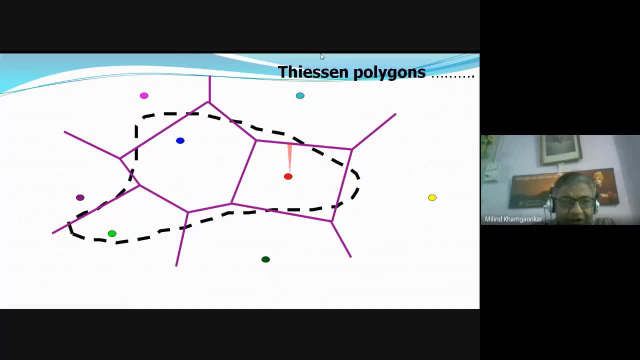 bisectors are drawn, they are connected, and then the catch the weight a weird. and then the catch the weight a weird, and then the catch the weight a weird. area or weighted area as has been shown. area or weighted area as has been shown. area or weighted area as has been shown here for the p1 rain gauge station a1. 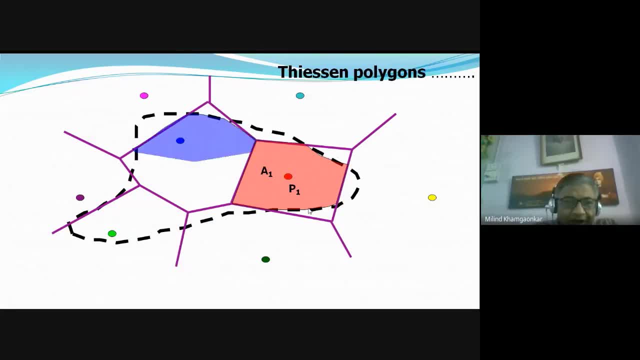 here for the p1 rain gauge station a1. here for the p1 rain gauge station. a1 is the weighted area for the another. p2 is the weighted area for the another. p2 is the weighted area for the another p2 rain gauge station. this is the another. 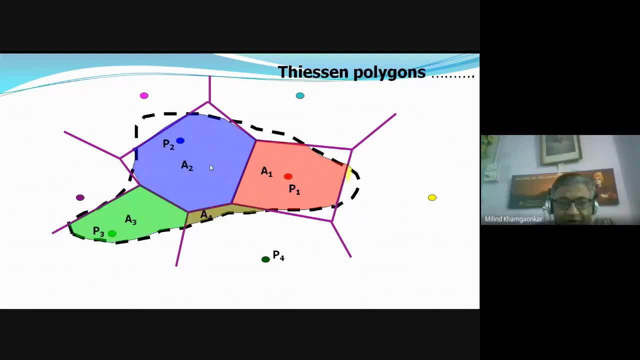 rain gauge station. this is the another rain gauge station, this is the another area. so in this way, all the areas are area. so in this way, all the areas are area. so in this way, all the areas are found out. and again a formula which is found out, and again a formula which is: 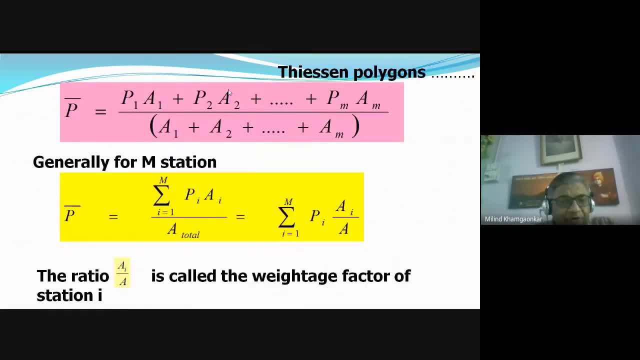 found out, and again, a formula which is equal to p1 into the concerned, weighted, equal to p1 into the concerned, weighted equal to p1 into the concerned weighted area, plus p2 into concerned weighted area, plus p2 into concerned weighted area, plus p2 into concerned weighted area, and so on, divided by the total area. 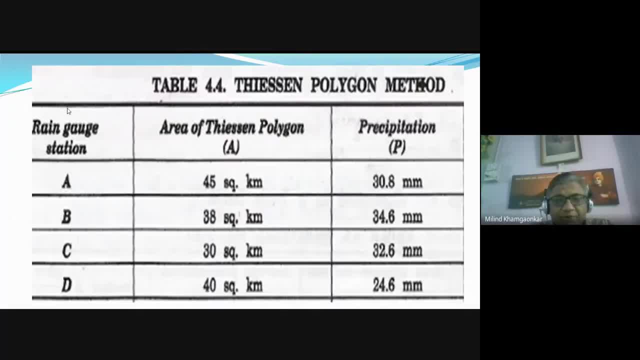 area, and so on. divided by the total area, area and so on, divided by the total area will give you the average or the mean will give you the average or the mean will give you the average or the mean. precipitation over the catchment area. precipitation over the catchment area. 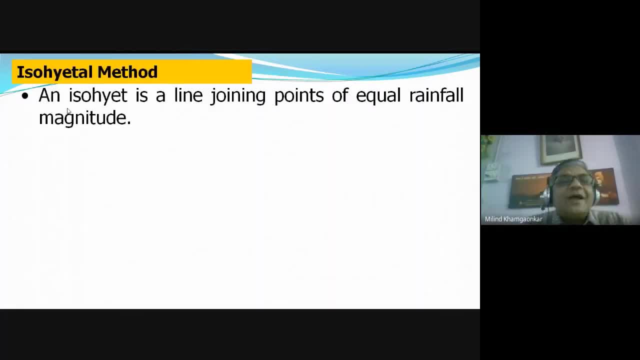 precipitation over the catchment area. this is one of the salt numerical over. this is one of the salt numerical over. this is one of the salt numerical over the and the third or the last is the the and the third or the last is the the and the third or the last is the isohytal method. isohyte friends is a. 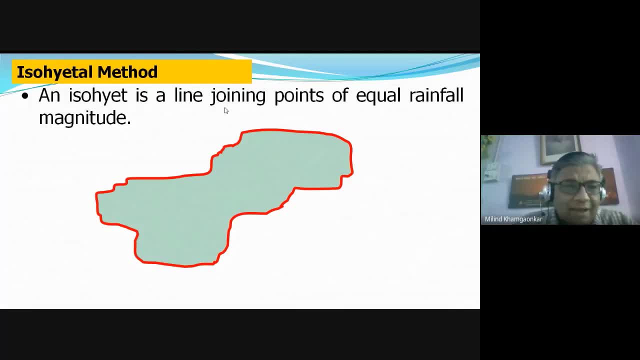 isohytal method. isohyte friends is a isohytal method. isohyte friends is a line joining points of equal or equal line. joining points of equal or equal line. joining points of equal or equal rainfall magnitude is called as the rainfall magnitude is called as the 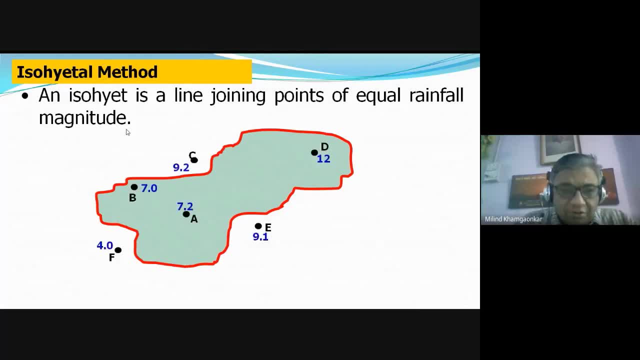 rainfall magnitude is called as the isoids, as like the season polygon. the isoids as like the season polygon, the isoids as like the season polygon. the whole catchment area is again further whole catchment area is again further whole catchment area is again further subdivided between the various ISO. 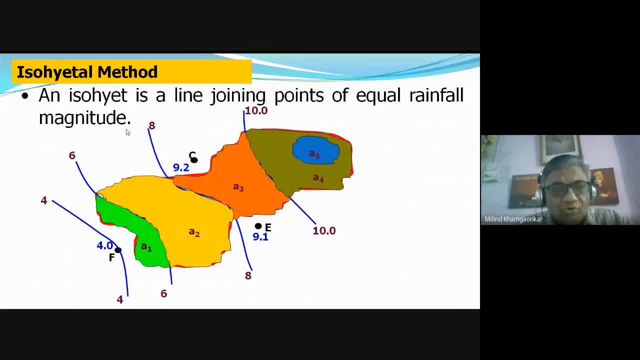 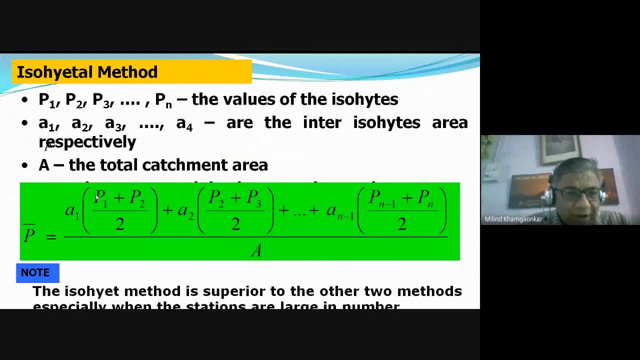 subdivided between the various ISO, subdivided between the various ISO heights, and is being read according to heights. and is being read according to heights, and is being read according to those isoids, and again that area, those isoids, and again that area, those isoids, and again that area multiplied by the area which is bounded. 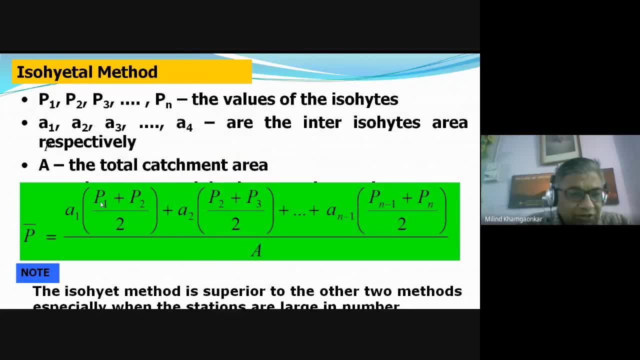 multiplied by the area which is bounded. multiplied by the area which is bounded by two isoids of rainfall intensity, p1. by two isoids of rainfall intensity, p1. by two isoids of rainfall intensity, p1 and p2, so average of this rainfall and p2, so average of this rainfall. 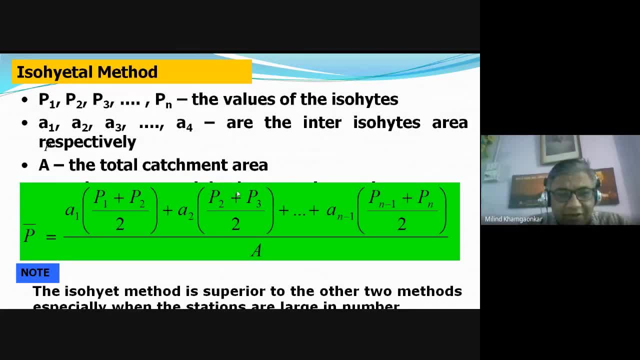 and p2. so average of this rainfall. intensities of the isoid multiplied intensities of the isoid multiplied intensities of the isoid multiplied by that area. in this way, all areas. and by that area, in this way, all areas. and by that area, in this way, all areas and their corresponding average. 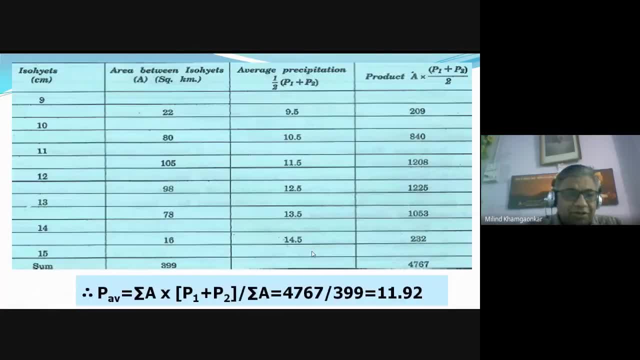 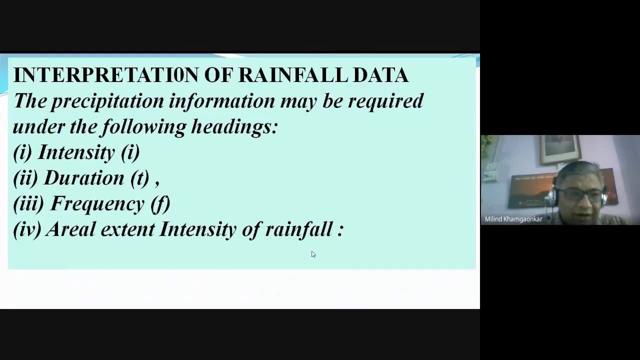 their corresponding average. their corresponding average. precipitation average: it is being worked. precipitation average: it is being worked. precipitation average: it is being worked out. and the overall average out and the overall average out, and the overall average precipitation is being formed. the precipitation is being formed. the precipitation is being formed. the interpretation of the rainfall data is: 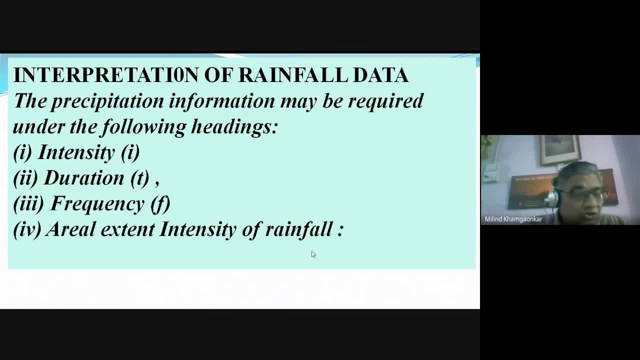 interpretation of the rainfall data is. interpretation of the rainfall data is done in the four types. this is very done in the four types. this is very done in the four types. this is very important. that is the intensity of important. that is the intensity of important. that is the intensity of rainfall duration: duration, frequency and 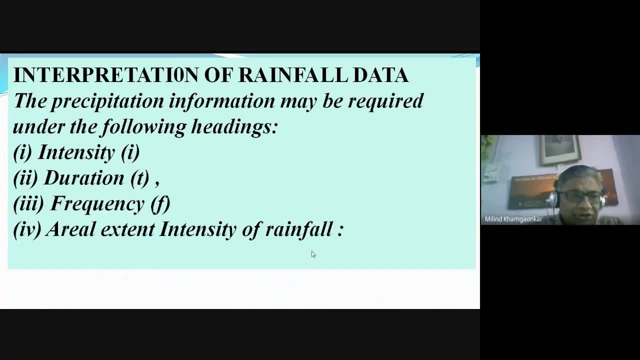 rainfall: duration, duration, frequency and rainfall duration, frequency and aerial extent. intensity of rainfall- aerial extent- intensity of rainfall- aerial extent. intensity of rainfall. intensity is always measured in intensity is always measured in intensity is always measured in centimeters per hour. duration is measured: centimeters per hour. duration is measured. 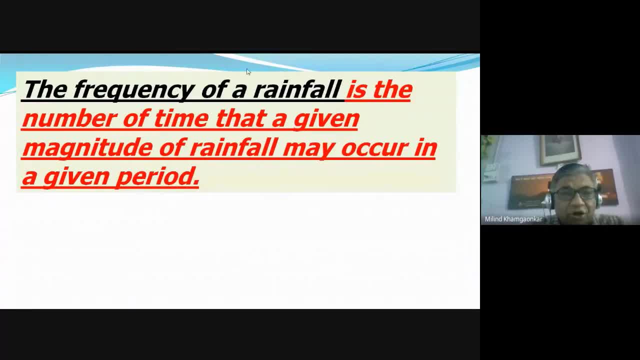 centimeters per hour. duration is measured in either minute second or our. in either minute second or our. in either minute second or our. frequency of rainfall is the number of frequency of rainfall is. the number of frequency of rainfall is the number of time that, given magnitude of rainfall, 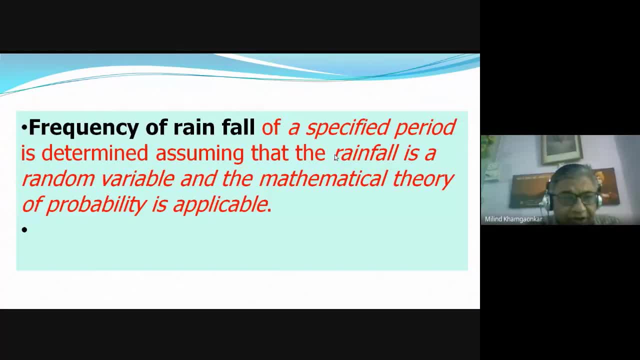 time that, given magnitude of rainfall, time that, given magnitude of rainfall, may occur in certain duration. that may occur in certain duration. that may occur in certain duration. that duration may be ten years, five years. duration may be ten years. five years. duration may be ten years, five years, fifty years, that frequency of rainfall. 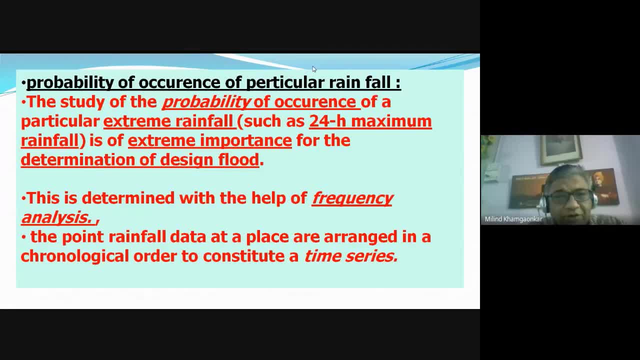 fifty years, that frequency of rainfall fifty years, that frequency of rainfall is very important from the probability of is very important from the probability of is very important from the probability of occurrence of particular rainfall, occurrence of particular rainfall, occurrence of particular rainfall quantity, so that for statistical study 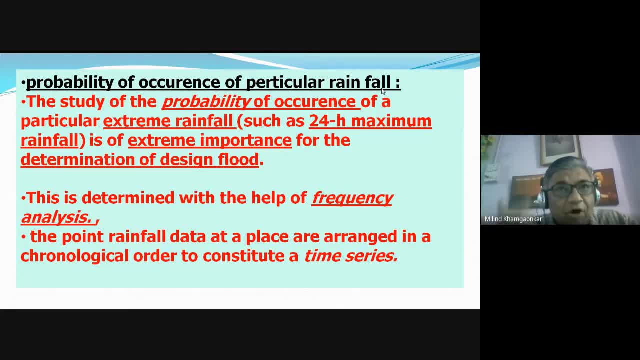 quantity so that for statistical study. quantity so that for statistical study to find out how much rainfall intensity, to find out how much rainfall intensity, to find out how much rainfall intensity or how much rainfall quantity will occur, or how much rainfall quantity will occur, or how much rainfall quantity will occur within 50 years, within 100 years, that 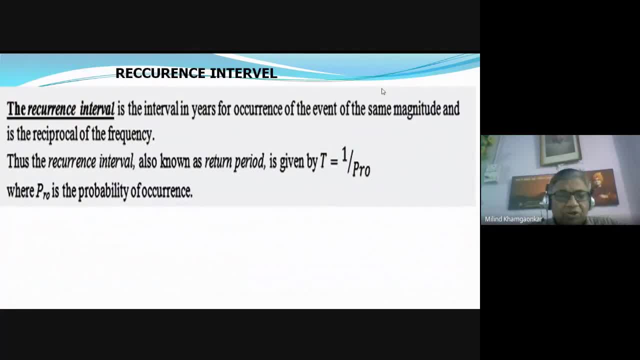 within 50 years, within 100 years, that within 50 years, within 100 years, that maximum quantity will help us to find maximum quantity, will help us to find maximum quantity, will help us to find out the floods and that return period a out the floods and that return period a. 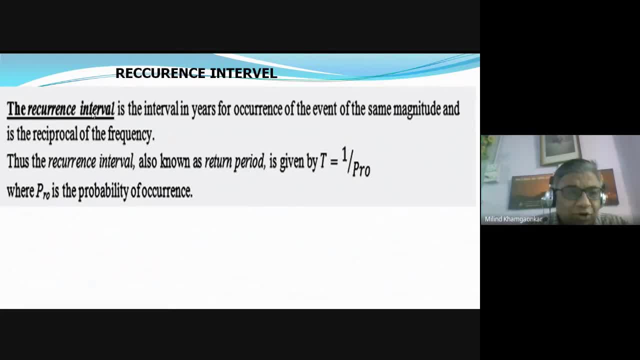 out the floods and that return period, a recurrence of the that rainfall. that is recurrence of the that rainfall, that is recurrence of the that rainfall. that is called as the recurrence interval, called as the recurrence interval, called as the recurrence interval or the return period. now, friends will 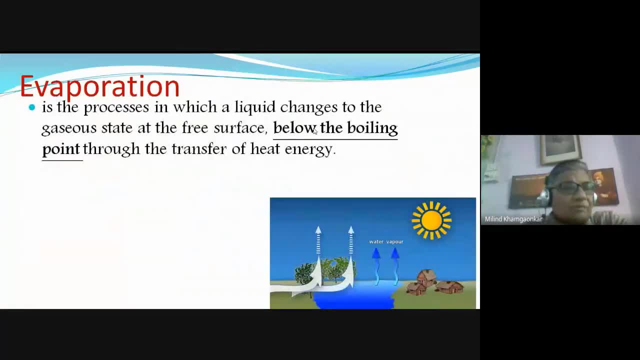 or the return period- now friends will, or the return period now, friends will move into the next component of the move, into the next component of the move, into the next component of the hydrologic cycle, that is the evaporation. hydrologic cycle: that is the evaporation. 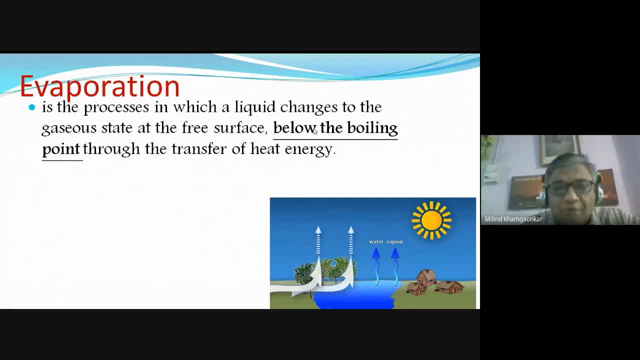 hydrologic cycle, that is the evaporation very important because in evaporation very important, because in evaporation very important, because in evaporation maximum part of the precipitation water, maximum part of the precipitation water, maximum part of the precipitation water gets lost. because we are interested in 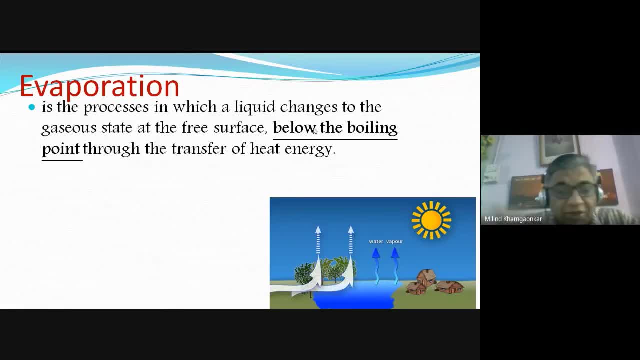 gets lost because we are interested in gets lost, because we are interested in conservation of the precipitation water, conservation of the precipitation water, conservation of the precipitation water, but in evaporation, but in evaporation, but in evaporation due to the solar radiation and solar heat in our India. 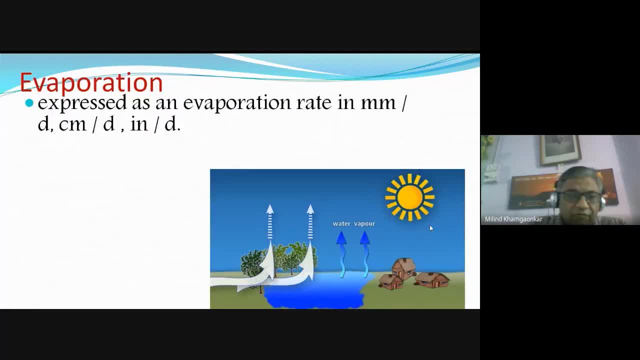 due to the solar radiation and solar heat in our India, due to the solar radiation and solar heat in our India, maximum water is lost, so maximum water is lost, so maximum water is lost. so therefore, the study of evaporation is. therefore the study of evaporation is. 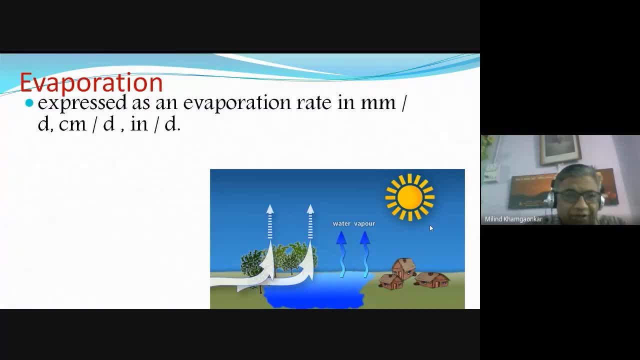 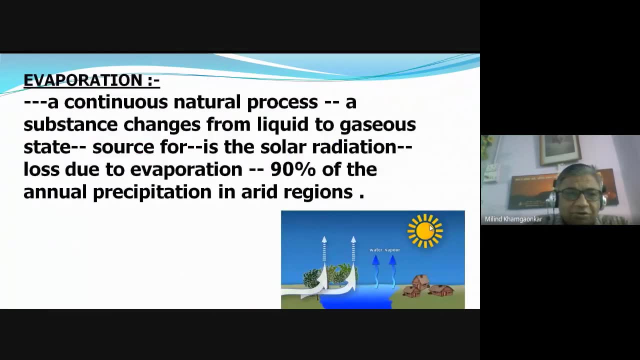 therefore, the study of evaporation is very important. it is measured in very important. it is measured in very important. it is measured in millimeters per day. centimeters per day. millimeters per day, centimeters per day. millimeters per day, centimeters per day. so it is the method wherein the water 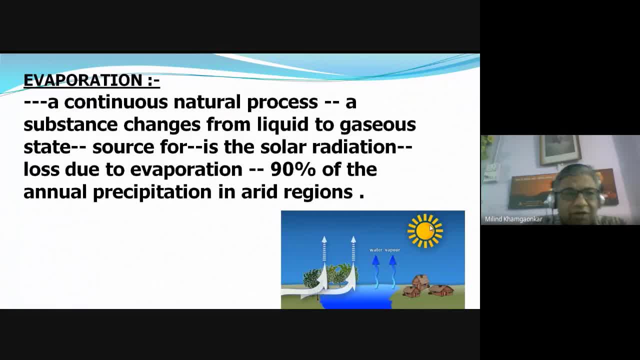 so it is the method wherein the water. so it is the method wherein the water vapor. the water in the liquid form gets vapor. the water in the liquid form gets vapor. the water in the liquid form gets converted into the gaseous state due to. converted into the gaseous state due to. 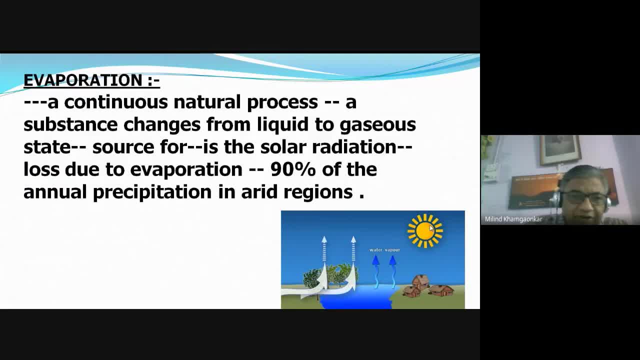 converted into the gaseous state due to the solar radiation, due to the heat. the solar radiation due to the heat, the solar radiation due to the heat, which is being provided with the help of, which, is being provided with the help of, which is being provided with the help of the solar radiation, and almost 90% of 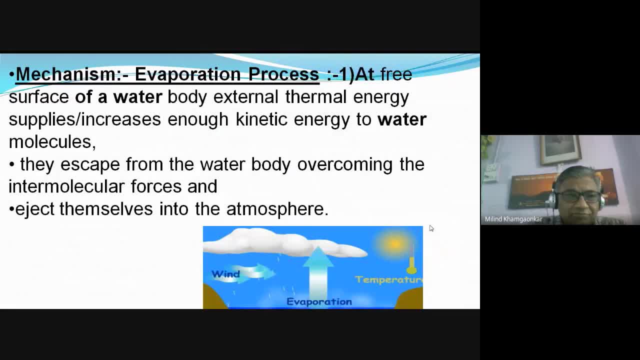 the solar radiation and almost 90% of the solar radiation and almost 90% of the water is lost in evaporation. the the water is lost in evaporation, the the water is lost in evaporation. the mechanism of the evaporation process is. mechanism of the evaporation process is: 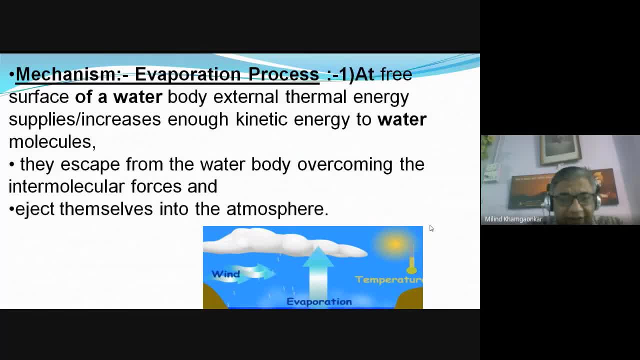 mechanism of the evaporation process is that the water molecules which are there, that the water molecules which are there, that the water molecules which are there at the surface of the water body gets at the surface of the water body. gets at the surface of the water body, gets external heat energy, thermal energy. 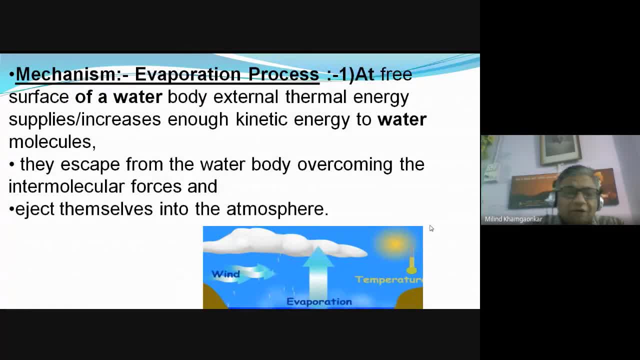 external heat energy. thermal energy. external heat energy: thermal energy from the atmosphere, or sometimes it from the atmosphere, or sometimes it from the atmosphere, or sometimes it gets the thermal energy from water body, gets the thermal energy from water body, gets the thermal energy from water body itself and due to this thermal energy. 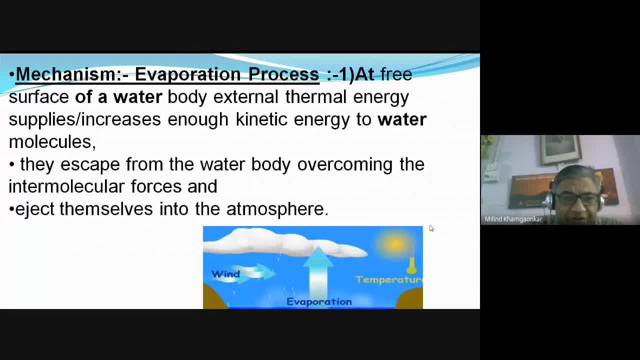 itself and due to this thermal energy itself and due to this thermal energy the molecules at the water surface gets the molecules at the water surface, gets the molecules at the water surface, gets kinetic energy, it starts moving. and when kinetic energy it starts moving, and when kinetic energy it starts moving and when their kinetic energy reaches to certain 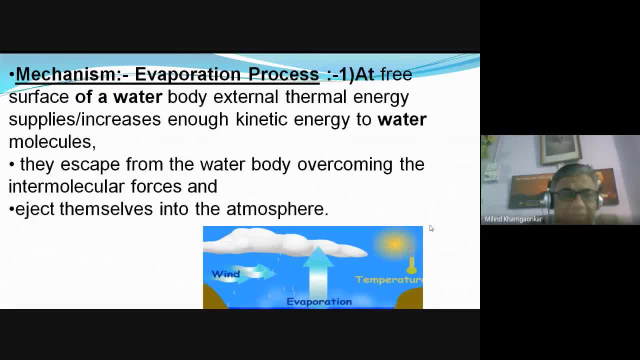 their kinetic energy reaches to certain. their kinetic energy reaches to certain value wherein now they cannot remain in value. wherein now they cannot remain in value. wherein now they cannot remain in the at the water surface of the water, the at the water surface of the water, the at the water surface of the water body. then they leave the water surface gets. 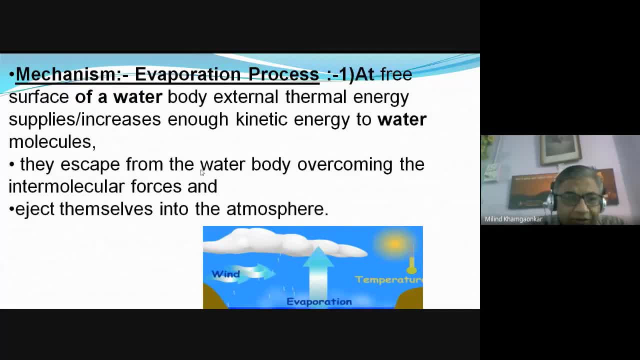 body, then they leave. the water surface gets body, then they leave. the water surface gets into the vapor, against the, into the vapor, against the, into the vapor, against the intermolecular forces of the water, intermolecular forces of the water, intermolecular forces of the water particle, and they get ejected into the 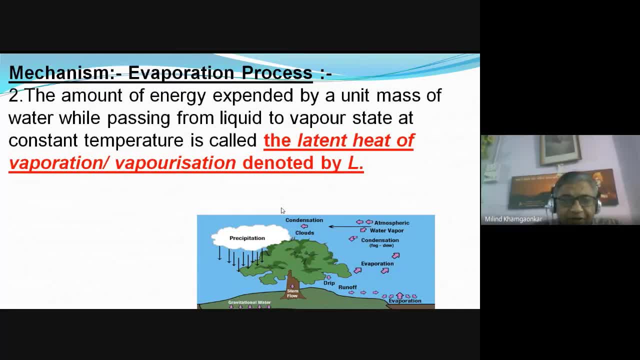 particle and they get ejected into the particle and they get ejected into the atmosphere. this is called as the atmosphere, this is called as the atmosphere. this is called as the evaporation, the heat which is the heat. evaporation, the heat which is the heat. evaporation, the heat which is the heat, either from the atmosphere or from the 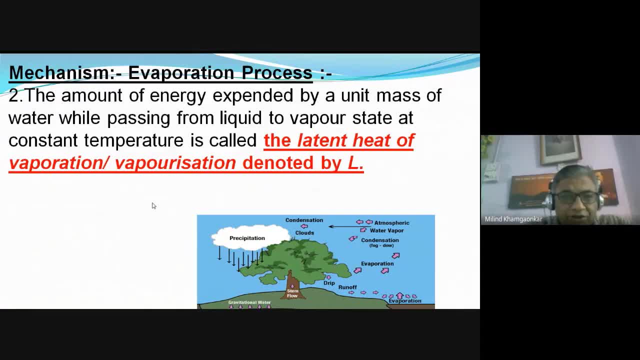 either from the atmosphere or from the- either from the atmosphere or from the water body that is being used for the water body that is being used for the water body that is being used for the evaporation is called as the latent heat. evaporation is called as the latent heat. 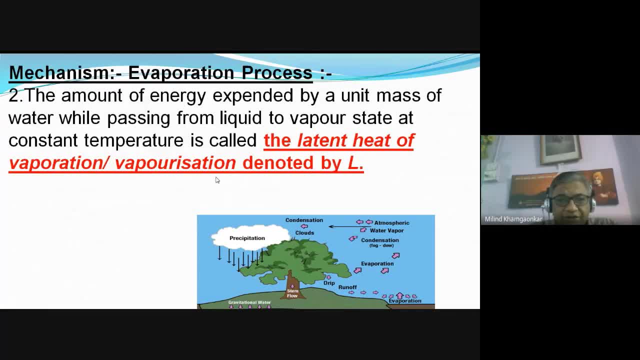 evaporation is called as the latent heat of evaporation or latent heat of of evaporation, or latent heat of of evaporation, or latent heat of vaporization. it is denoted by L as I have vaporization. it is denoted by L as I have. 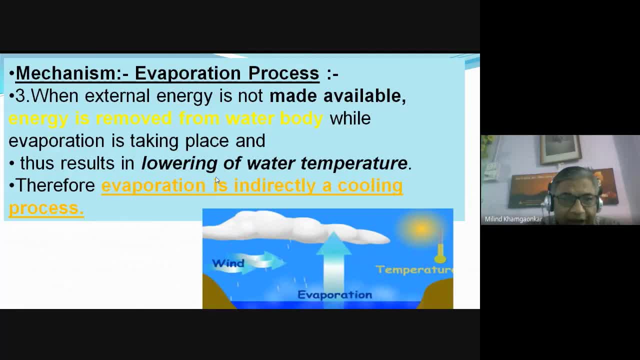 vaporization. it is denoted by L, as I have told you. either they get the energy, told you, either they get the energy, told you, either they get the energy from the atmosphere, or sometimes they get the from the atmosphere, or sometimes they get the from the atmosphere, or sometimes they get the energy from the water body and 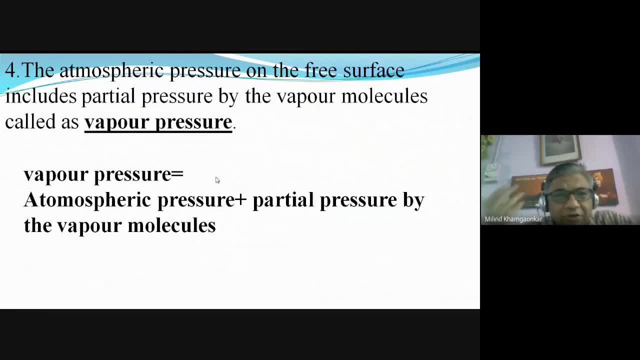 energy from the water body and energy from the water body and converts the water body into the cooler, converts the water body into the cooler, converts the water body into the cooler temperature. so therefore in evaporation temperature, so therefore in evaporation temperature. so therefore, in evaporation the water gets cooled also and the 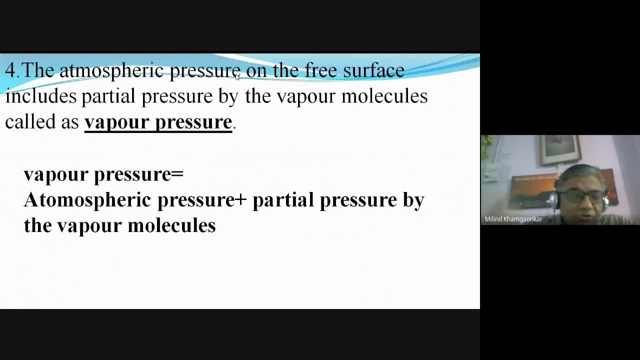 the water gets cooled also, and the the water gets cooled also, and the atmosphere also gets cooled. so atmosphere also gets cooled, so atmosphere also gets cooled. so evaporation is, though gets converted. evaporation is, though gets converted. evaporation is, though gets converted: conversion of the water vapor into the 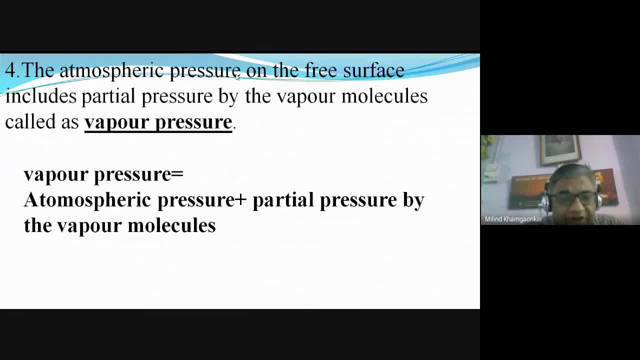 conversion of the water vapor into the conversion of the water vapor, into the conversion of water particle, into the conversion of water particle, into the conversion of water particle into the vapor state. but it cools either the water vapor state, but it cools either the water vapor state, but it cools either the water or to the atmosphere, the pressure. 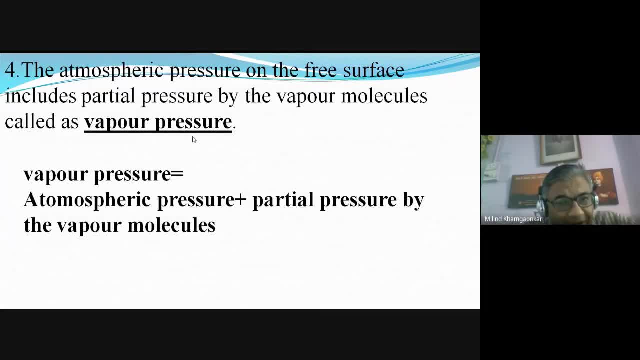 or to the atmosphere, the pressure or to the atmosphere, the pressure that has been created by the water vapor, that has been created by the water vapor, that has been created by the water vapor. particle over the water surface is particle over the water surface is particle over the water surface is called as the vapor pressure, which is 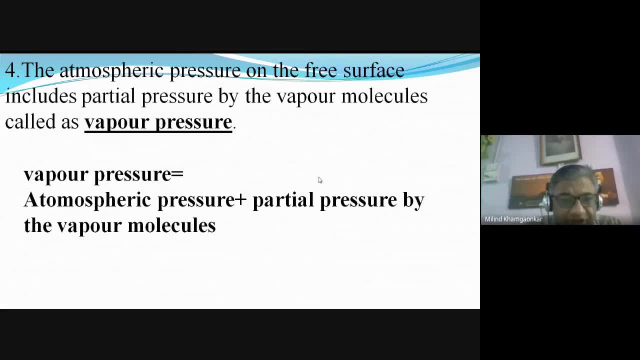 called as the vapor pressure, which is called as the vapor pressure, which is the vapor pressure, which is the the vapor pressure, which is the the vapor pressure, which is the summation of the pressure due to the summation of the pressure, due to the summation of the pressure due to the vapor molecule plus atmospheric pressure. 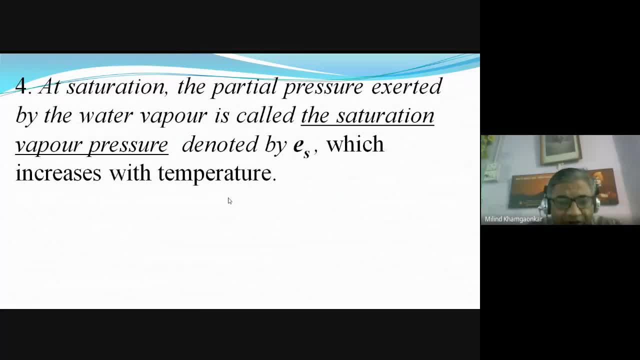 vapor molecule plus atmospheric pressure, vapor molecule plus atmospheric pressure, when this vapor molecules gets, when this vapor molecules gets, when this vapor molecules gets concentrated, concentrated over the water, concentrated, concentrated over the water, concentrated, concentrated over the water surface, and of at certain state at surface and of at certain state at. 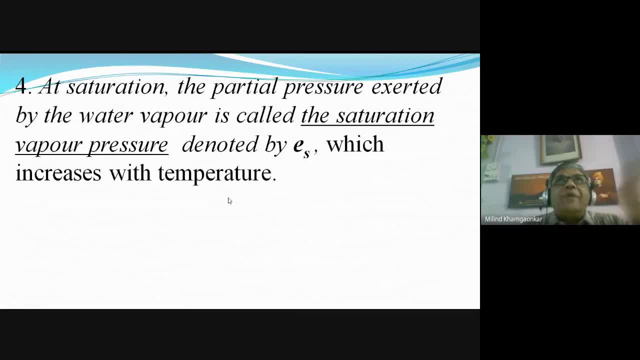 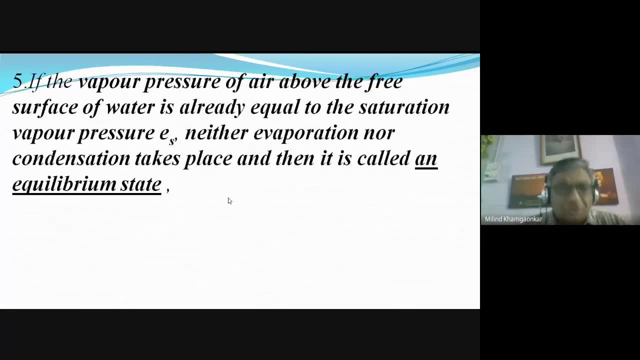 surface and of at certain state, at certain stage. this vapor cannot certain stage. this vapor cannot certain stage. this vapor cannot accommodate additional water vapor. that accommodate additional water vapor. that accommodate additional water vapor. that pressure is called as the saturation pressure, is called as the saturation pressure, is called as the saturation water pressure. and when this pressure 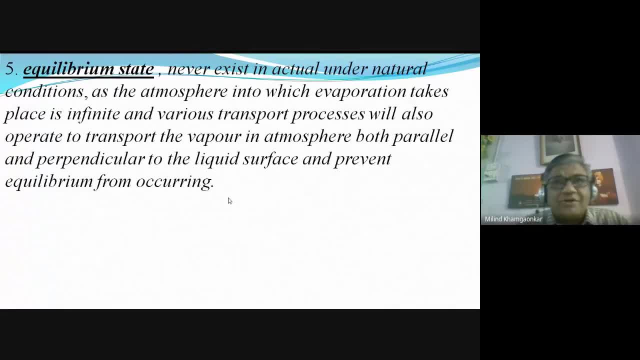 water pressure and when this pressure, water pressure, and when this pressure over the water surface reaches the over the water surface reaches the over the water surface, reaches the saturation water pressure, this water saturation water pressure, this water saturation water pressure, this water vapor does not allow the water from the 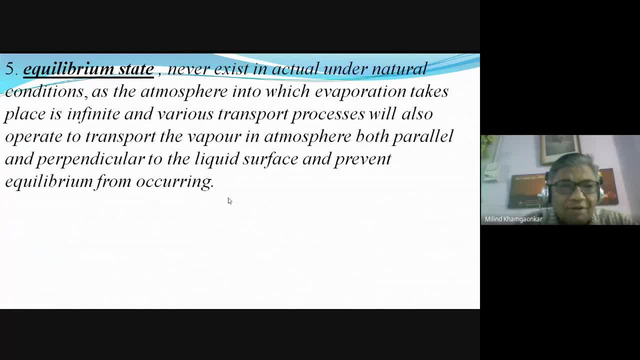 vapor does not allow the water from the vapor does not allow the water from the water body to convert into the vapor, water body to convert into the vapor, water body to convert into the vapor. this state is called as the equilibrium. this state is called as the equilibrium. 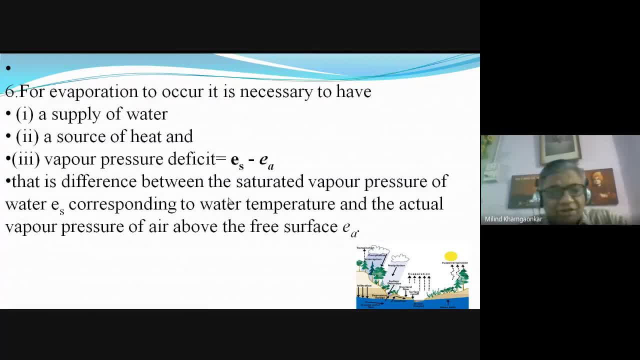 this state is called as the equilibrium state, and when this state reaches the state, and when this state reaches the state, and when this state reaches, the evaporation process decreases, so evaporation process decreases, so evaporation process decreases. so, therefore, for the evaporation to, therefore, for the evaporation to. 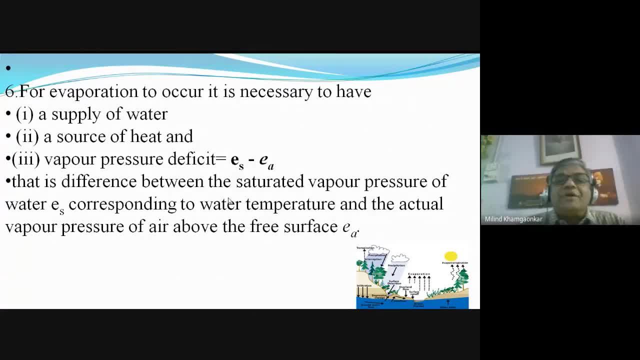 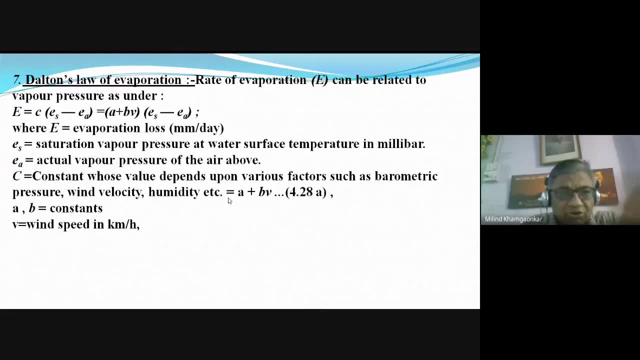 therefore, for the evaporation to occur, always the vapor pressure EA occur, always the vapor pressure EA occur, always the vapor pressure EA should be less than the saturation vapor, should be less than the saturation vapor, should be less than the saturation vapor pressure. there is one law based for: 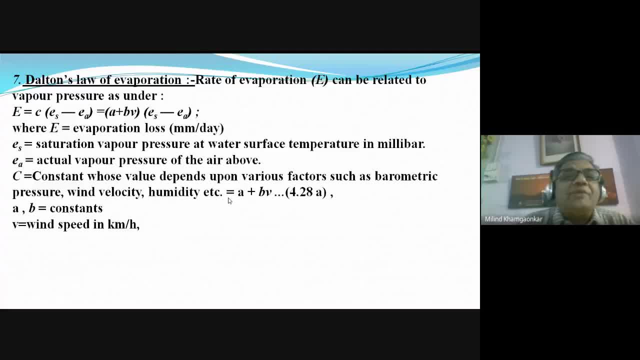 pressure. there is one law based for pressure. there is one law based for the process of the evaporation. that is the process of the evaporation. that is the process of the evaporation that is called as the Dalton's law of, called as the Dalton's law of. 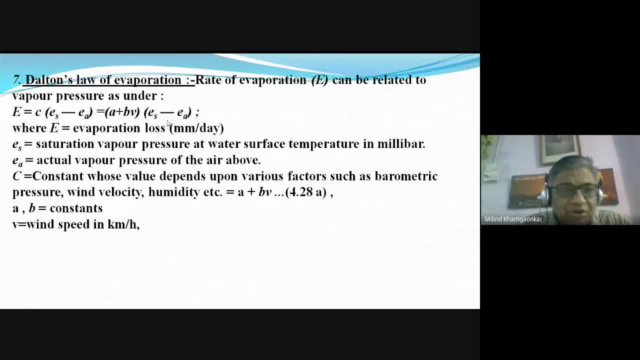 called as the Dalton's law of evaporation, which gives the evaporation, evaporation, which gives the evaporation, evaporation, which gives the evaporation loss. millimeters per day: ES is the loss. millimeters per day: ES is the loss. millimeters per day. ES is the saturation. vapor pressure. EA is the. 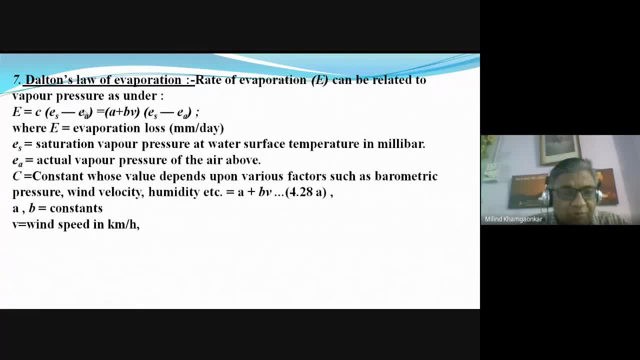 saturation vapor pressure. EA is the saturation vapor pressure, EA is the actual or the atmospheric vapor pressure. actual or the atmospheric vapor pressure? actual or the atmospheric vapor pressure? normal vapor pressure. so the deduction normal vapor pressure. so the deduction normal vapor pressure. so the deduction of this multiplied by the constant C is: 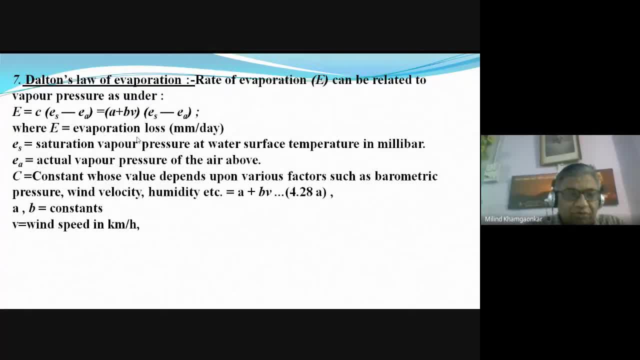 of this multiplied by the constant C is. of this, multiplied by the constant C, is called. is given by this. he gives us the called. is given by this. he gives us the called. is given by this. he gives us the evaporation loss. this is derived by mr. 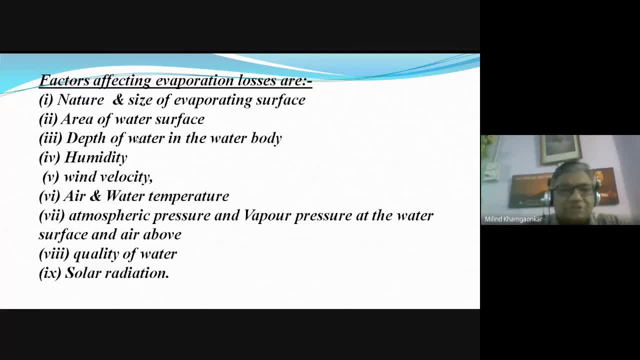 evaporation loss. this is derived by mr. evaporation loss. this is derived by mr. Dalton. when various factors are there, Dalton, when various factors are there. Dalton, when various factors are there which affects the evaporation, the again which affects the evaporation, the again which affects the evaporation, the again metrological or atmospheric pressure. 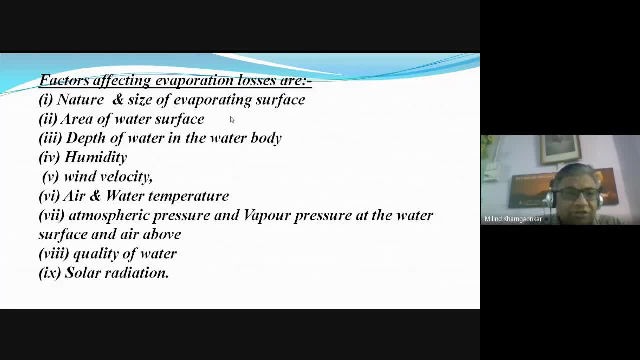 metrological or atmospheric pressure. metrological or atmospheric pressure, atmospheric factors: that is nature and atmospheric factors: that is nature. and atmospheric factors. that is nature and size of the surface area. depth of water. size of the surface area. depth of water. size of the surface area. depth of water, humidity, wind, velocity, temperature. 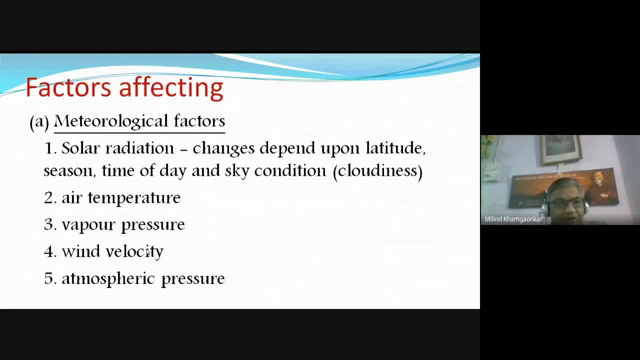 humidity, wind velocity, temperature. humidity, wind velocity, temperature. atmospheric pressure, quality of water. atmospheric pressure, quality of water. atmospheric pressure, quality of water. solar radiation: various factors are solar radiation. various factors are solar radiation. various factors are there. they can also be divided into the there. they can also be divided into the. 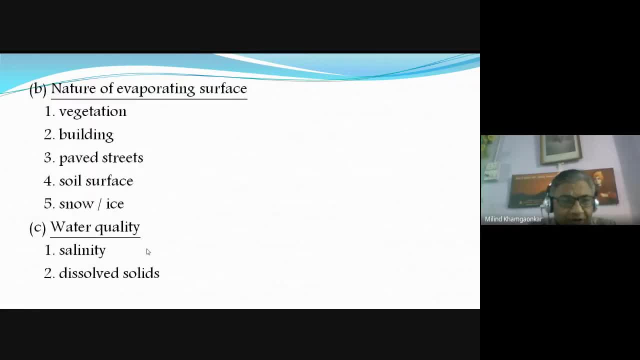 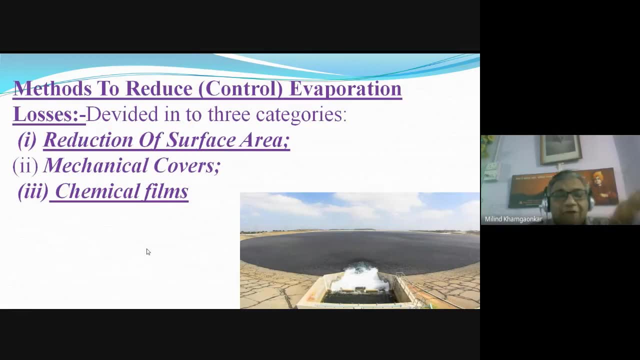 there. they can also be divided into the metrological, the soil surface. metrological, the soil surface, metrological, the soil surface characteristics. the water care quality characteristics, the water care quality characteristics, the water care quality characteristics. so as we have seen characteristics, so as we have seen characteristics, so as we have seen almost 90%. 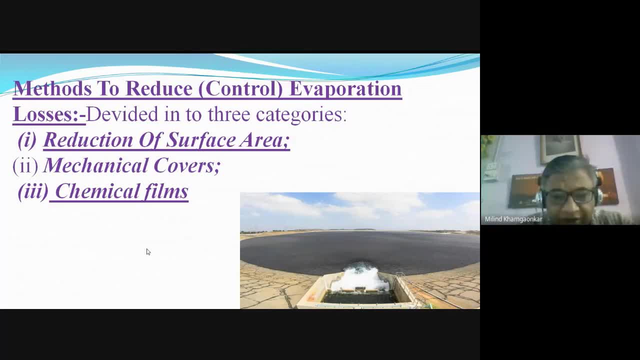 almost 90%, almost 90% of the precipitation water gets converted. of the precipitation water gets converted. of the precipitation water gets converted into the vapor. this much losses are into the vapor. this much losses are into the vapor. this much losses are there. there are various methods to. 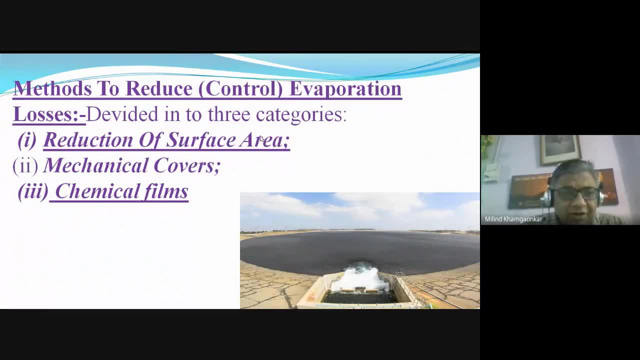 there. there are various methods to there. there are various methods to reduce the evaporation losses. they are: reduce the evaporation losses. they are: reduce the evaporation losses. they are: the reduction of the surface area. the reduction of the surface area, the reduction of the surface area, mechanical covers and chemical fields. so 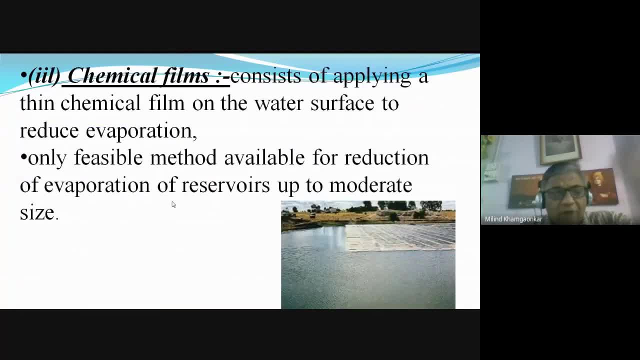 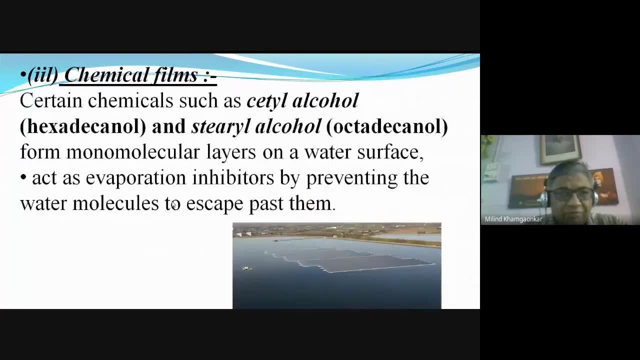 mechanical covers and chemical fields. so mechanical covers and chemical fields. so either providing the mechanical covers, either providing the mechanical covers, either providing the mechanical covers, or by increasing the depth of water, or by or by increasing the depth of water, or by or by increasing the depth of water, or by providing the chemical films, we can. 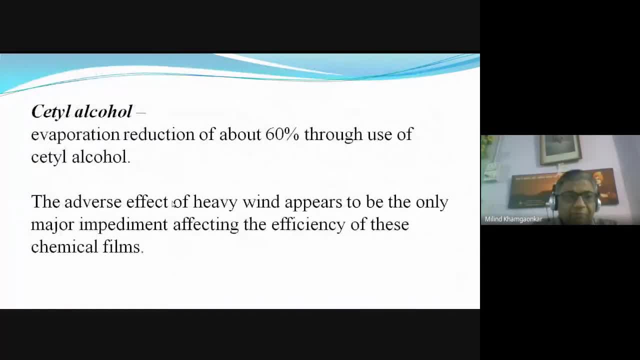 providing the chemical films. we can providing the chemical films. we can reduce the evaporation losses, mainly the reduce the evaporation losses, mainly the reduce the evaporation losses. mainly the CTL alcohol type B chemicals are used. CTL alcohol type B chemicals are used. CTL alcohol type B chemicals are used are sprayed over the water body, over the. 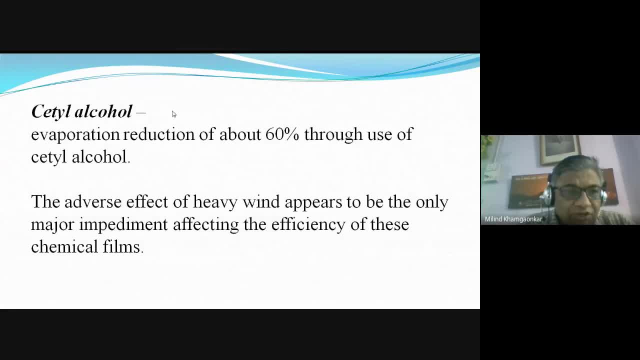 are sprayed over the water body, over the are sprayed over the water body, over the surface of water. you will hear you keep surface of water. you will hear you keep surface of water. you will hear you keep this name in your mind: CTL alcohol. is this name in your mind? CTL alcohol is. 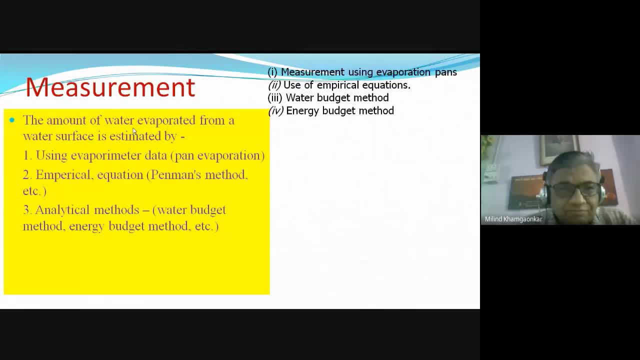 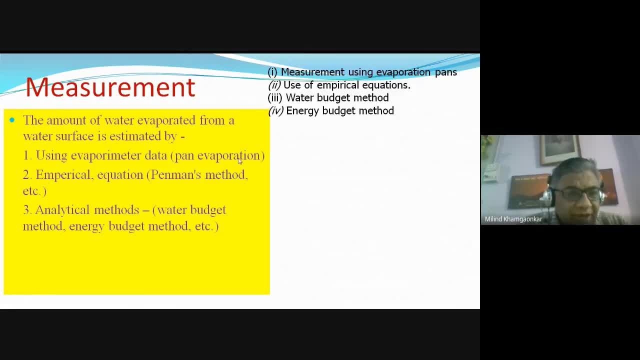 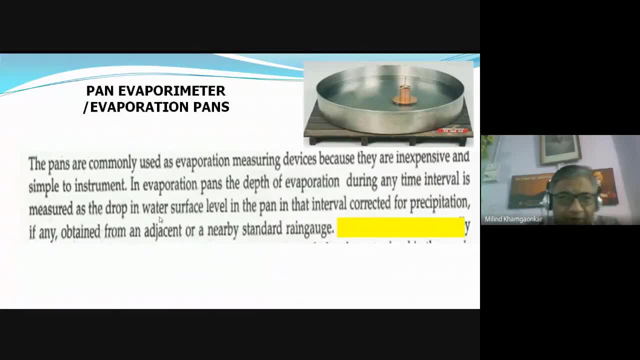 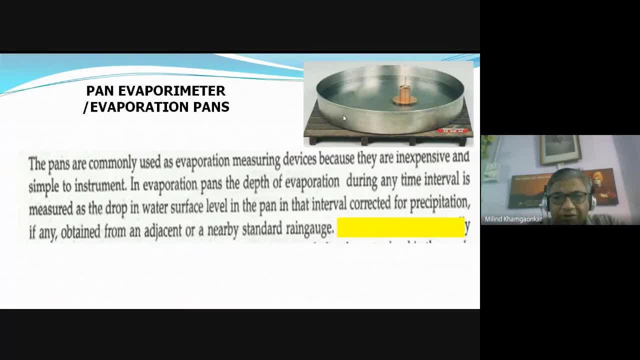 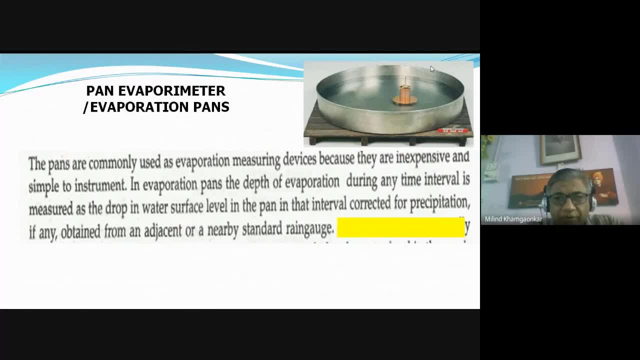 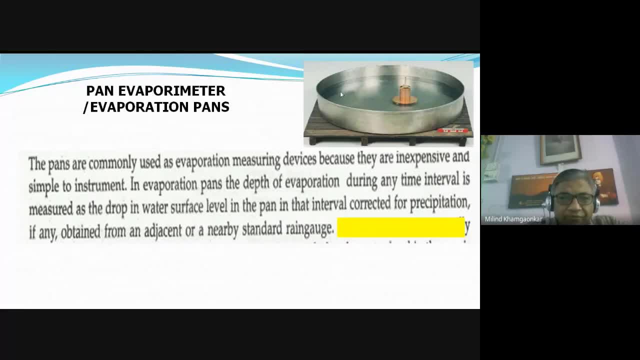 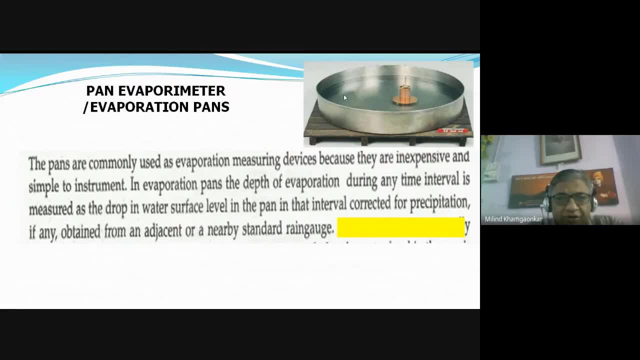 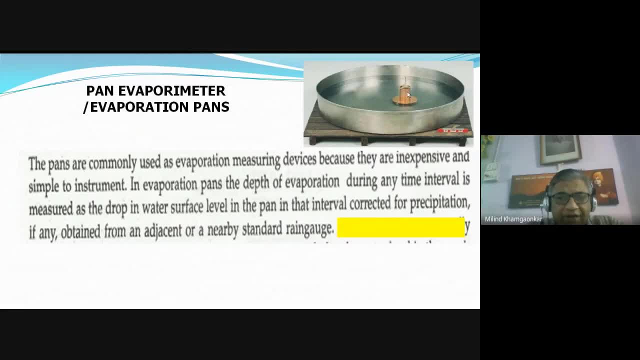 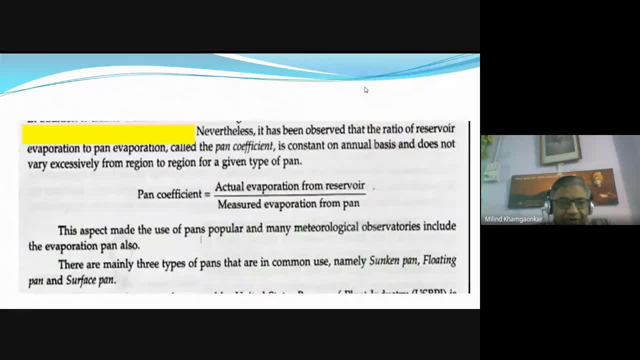 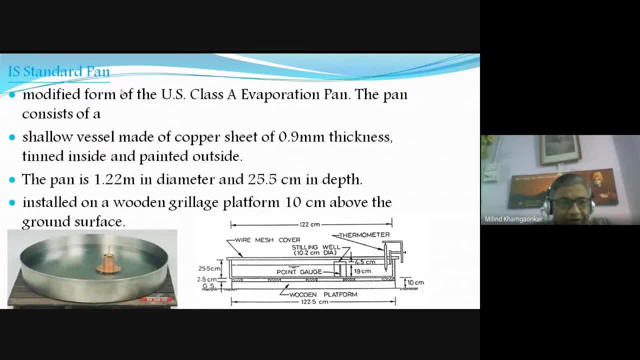 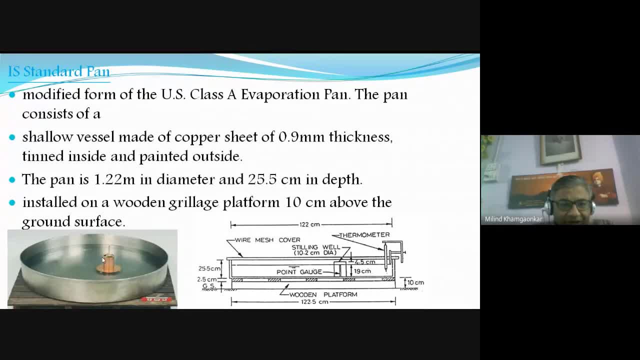 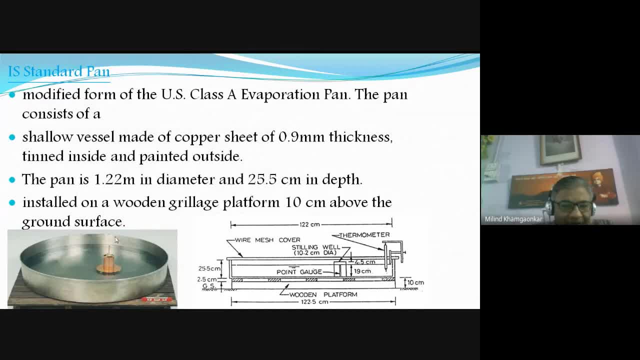 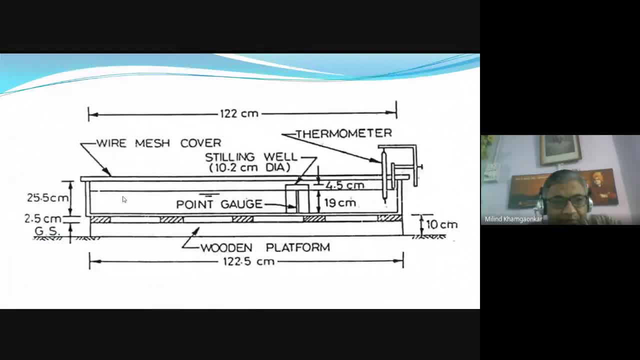 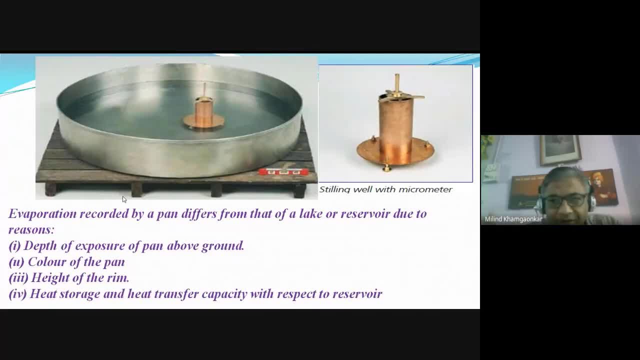 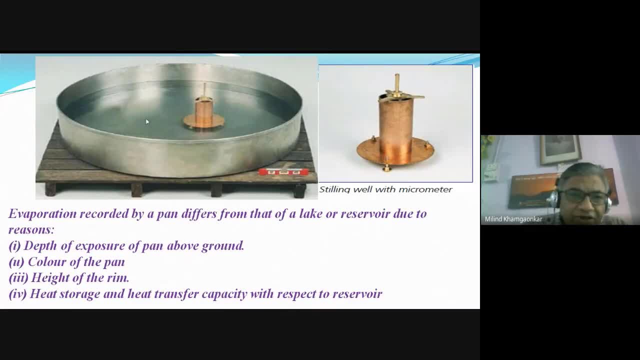 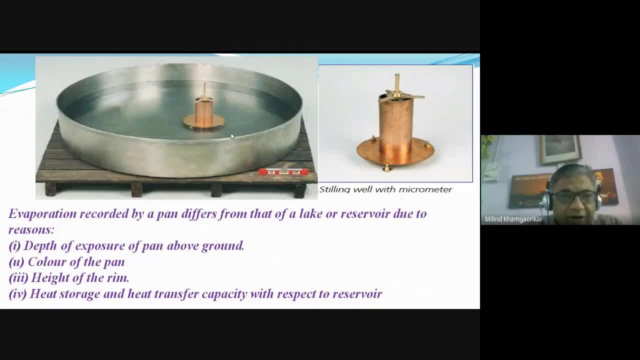 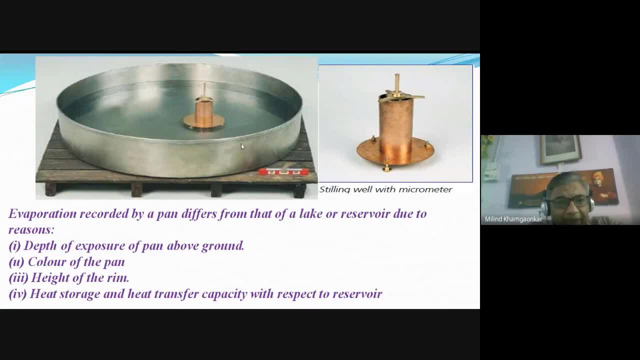 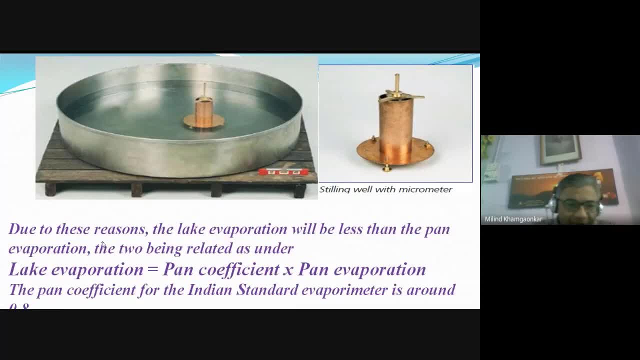 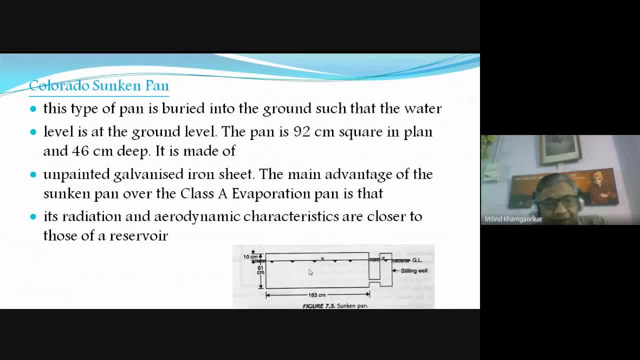 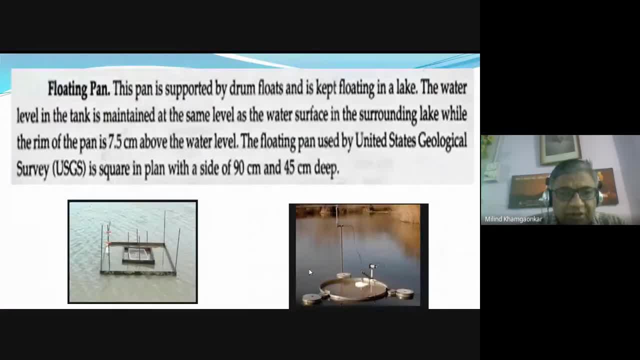 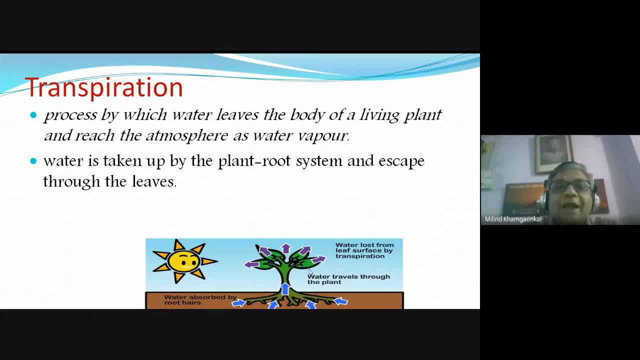 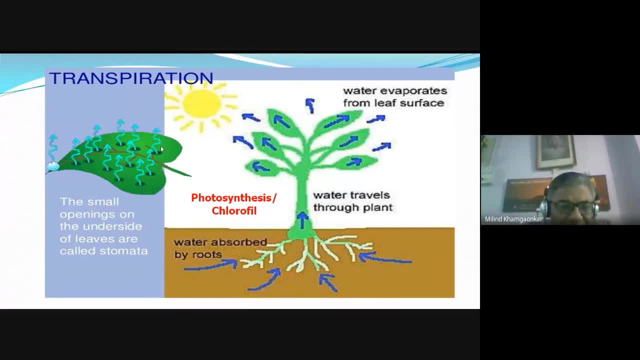 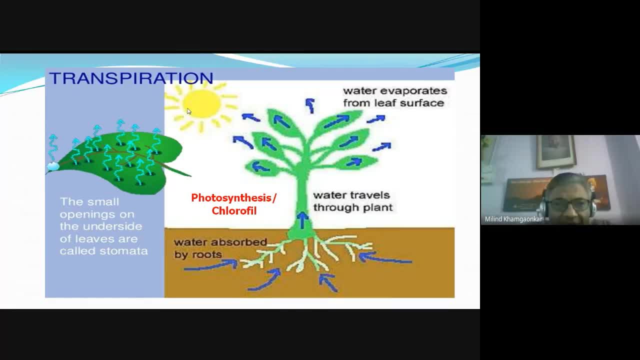 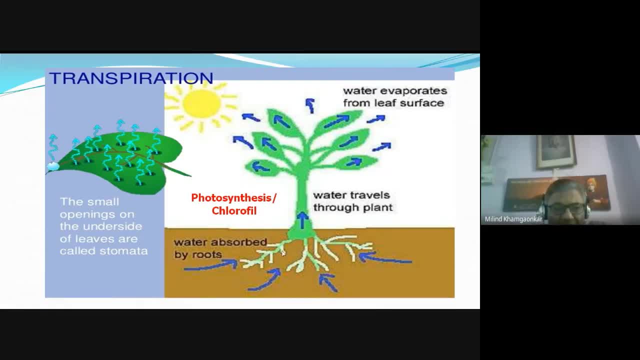 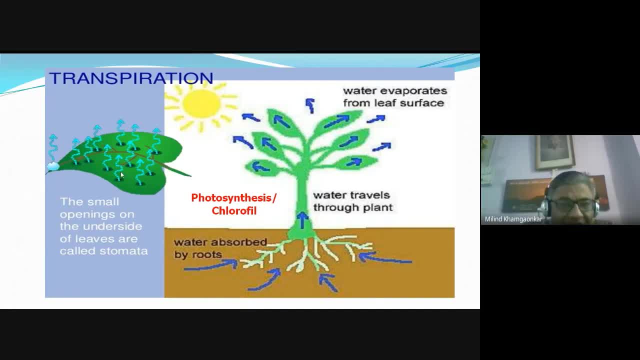 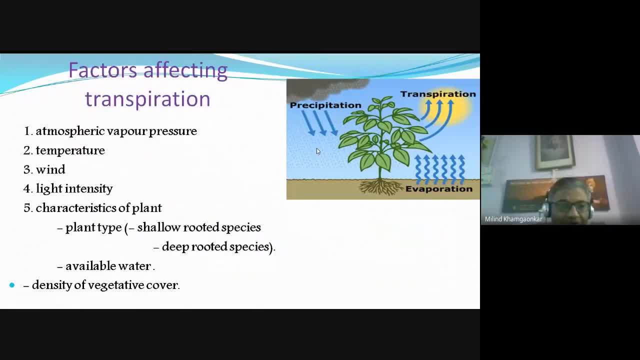 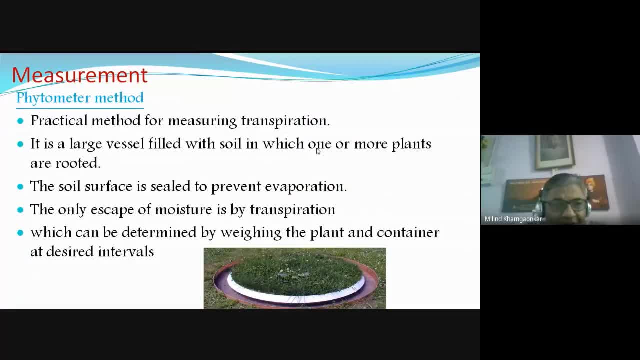 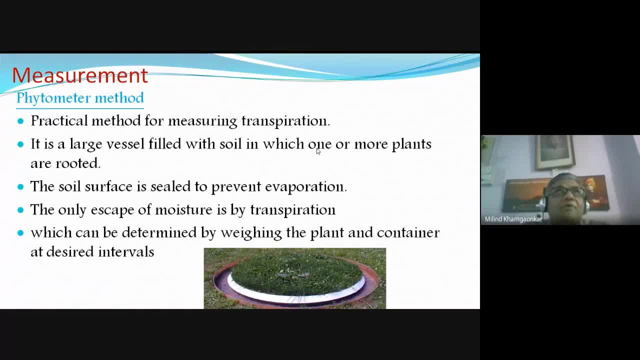 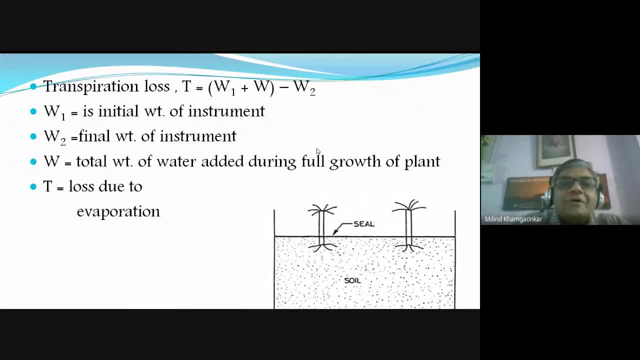 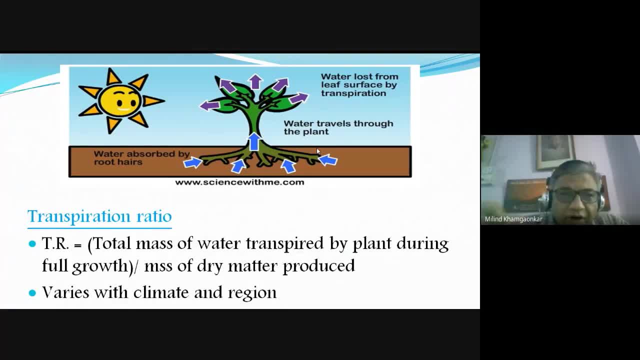 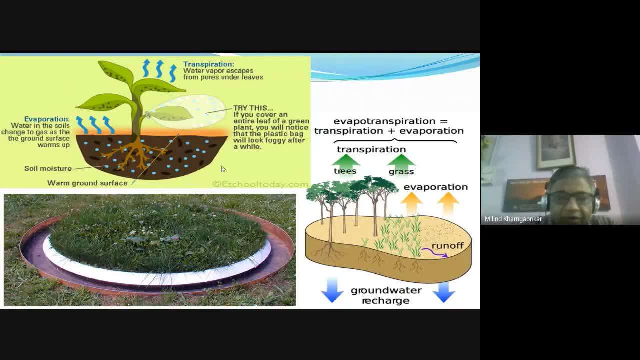 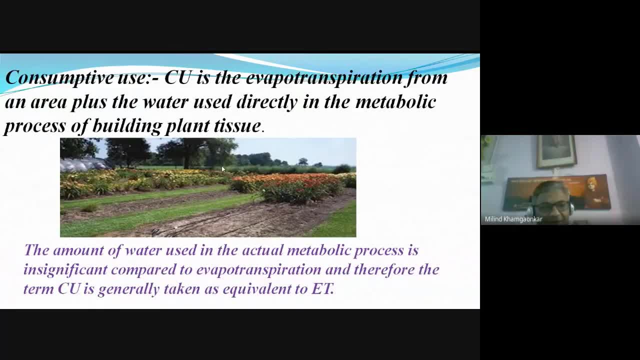 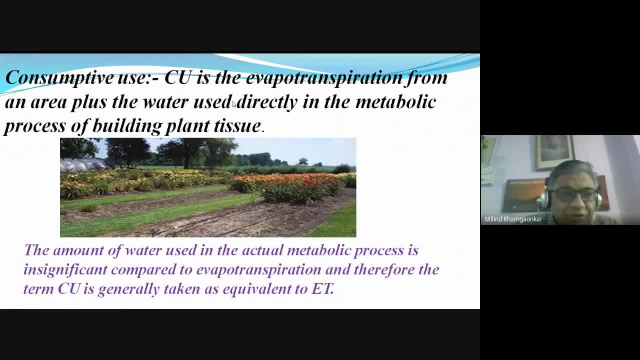 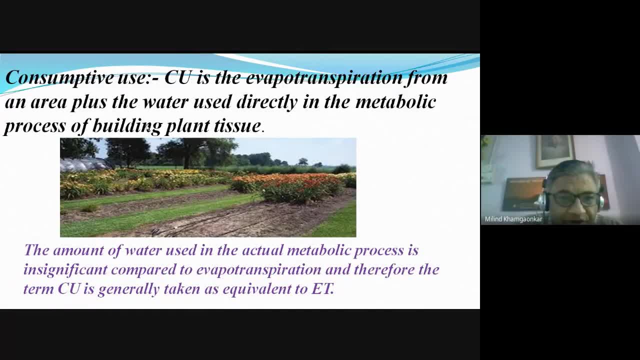 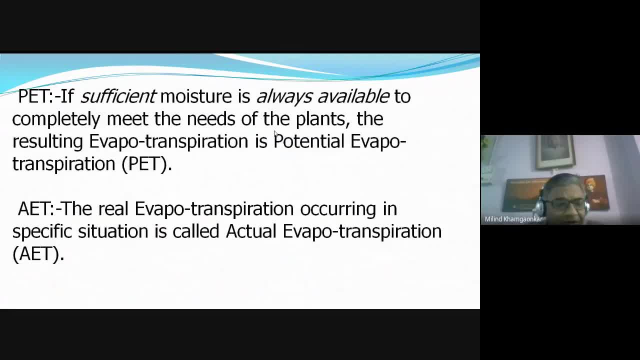 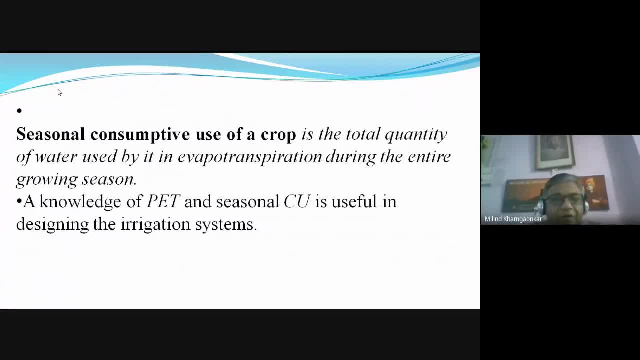 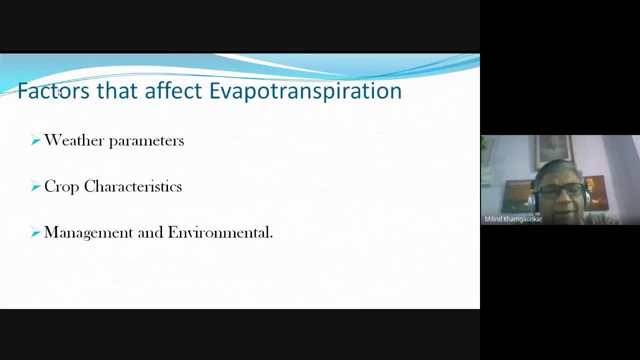 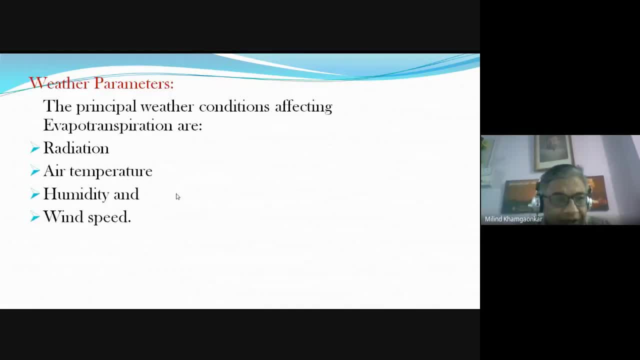 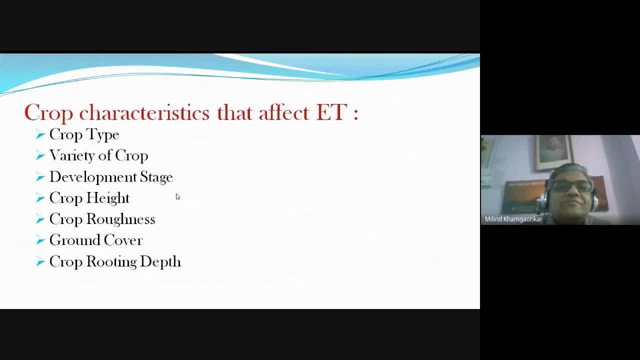 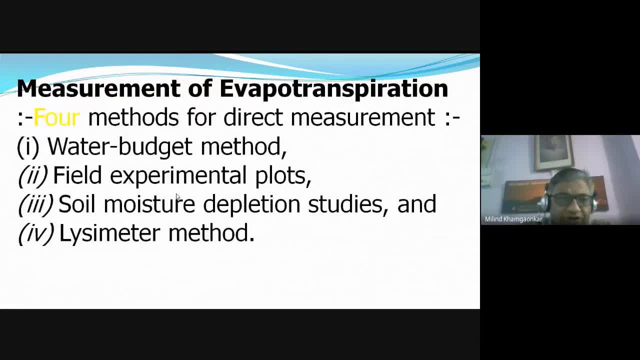 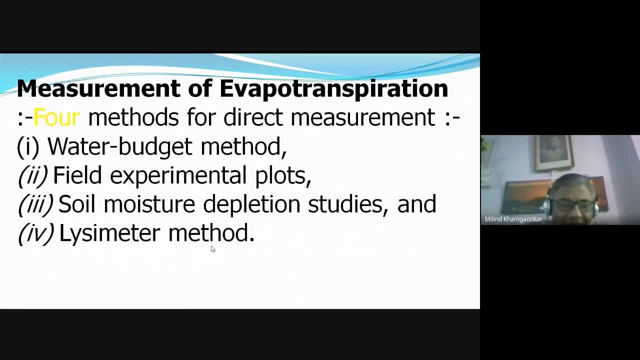 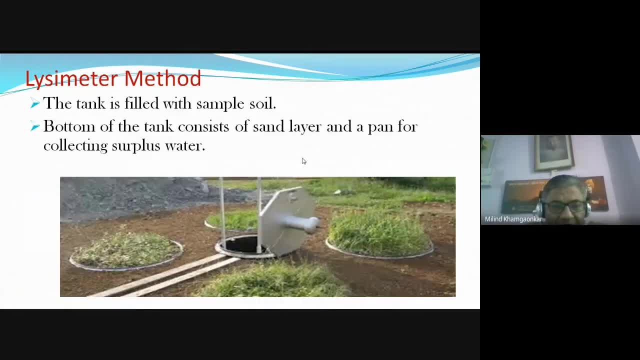 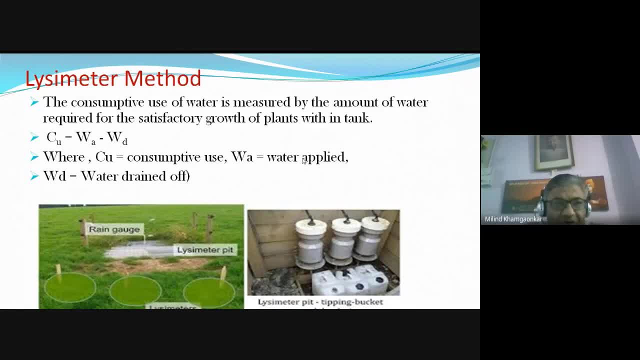 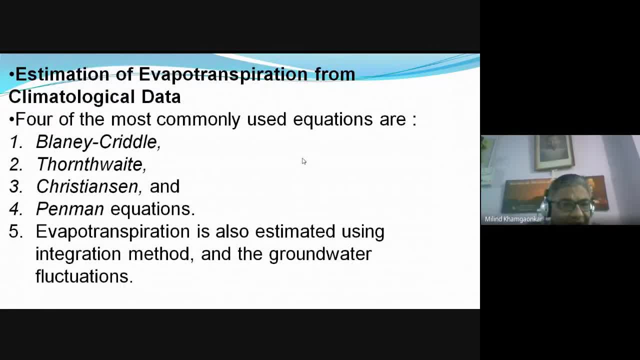 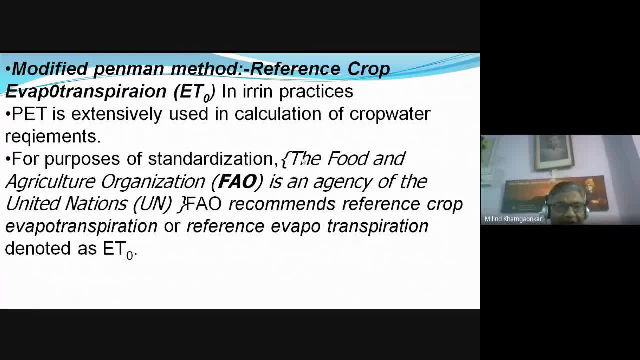 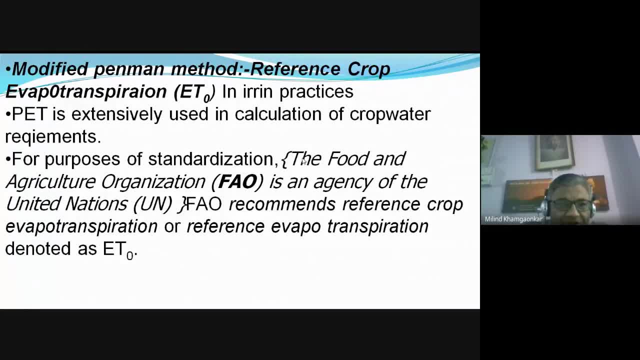 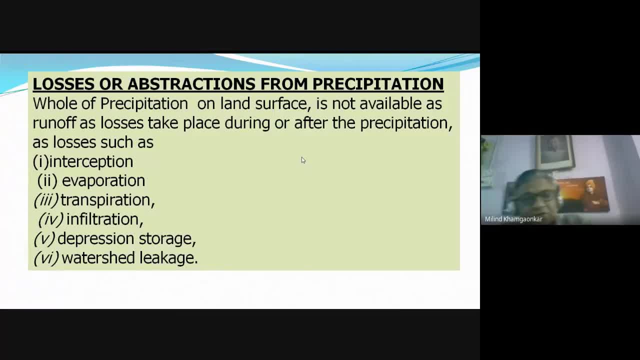 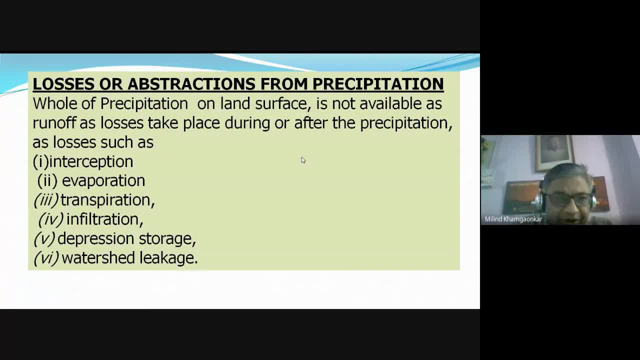 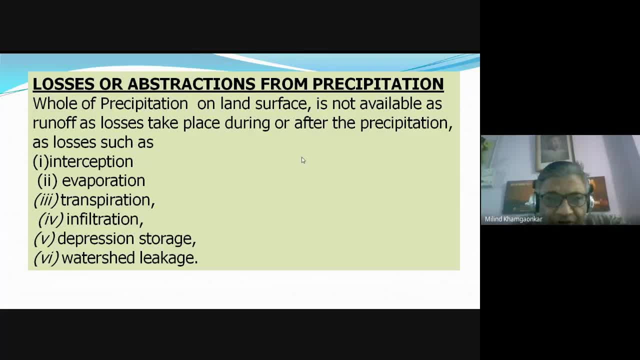 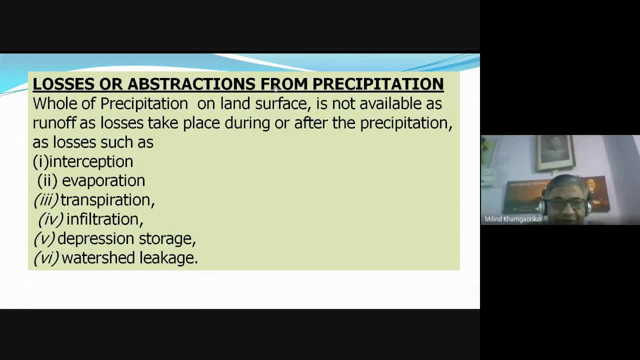 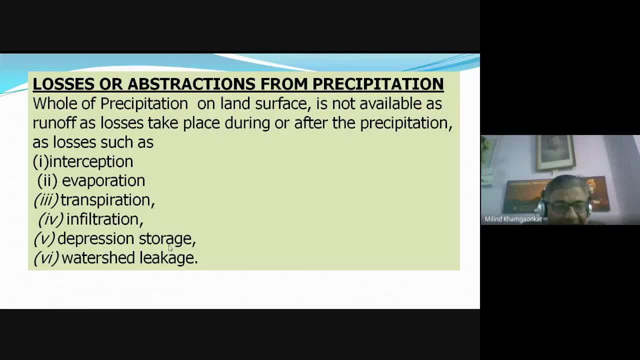 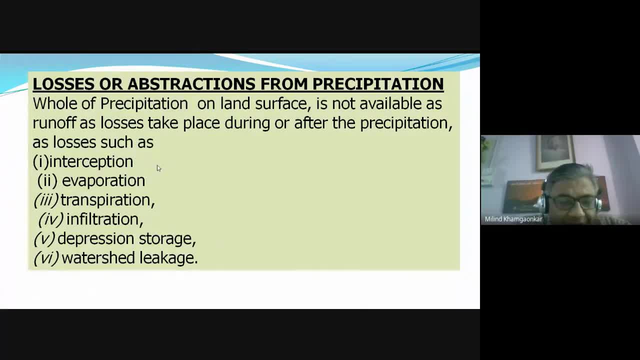 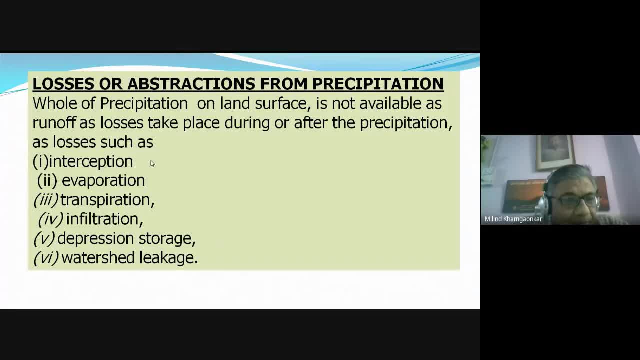 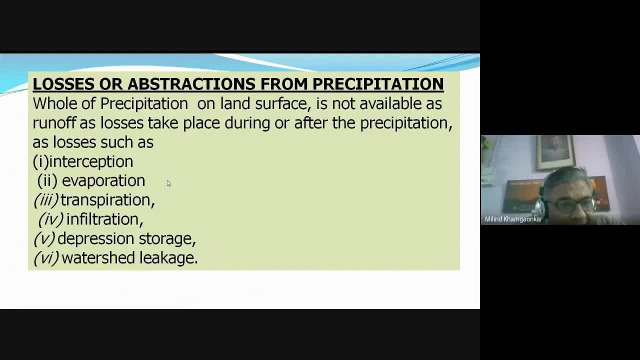 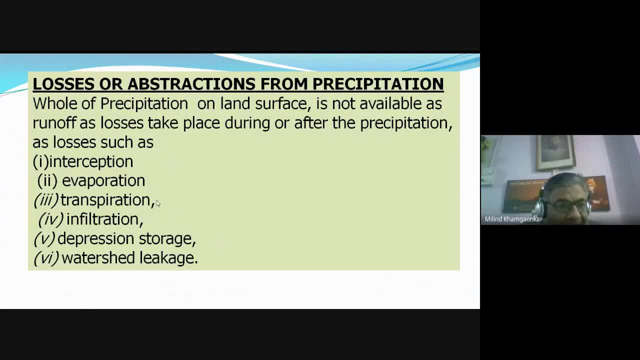 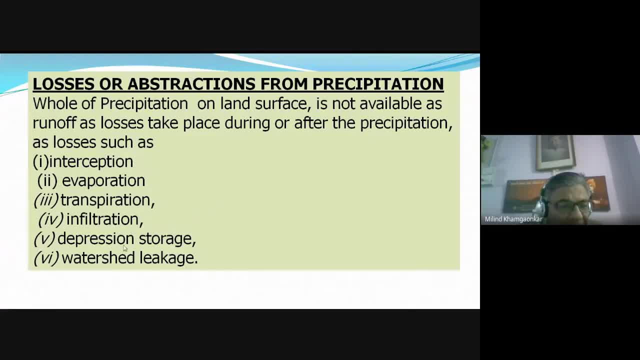 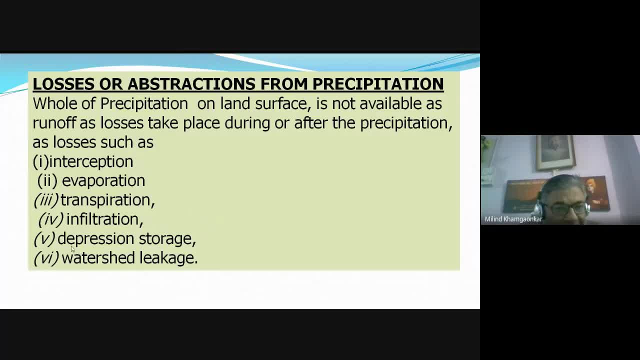 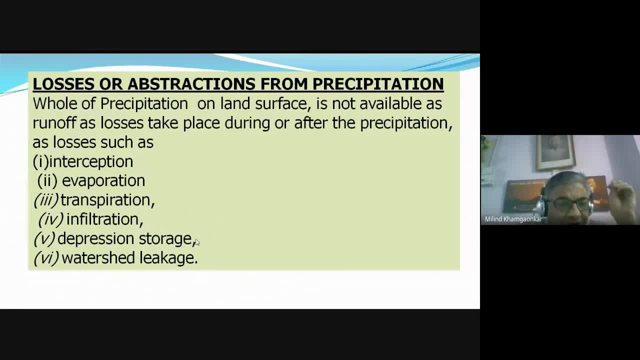 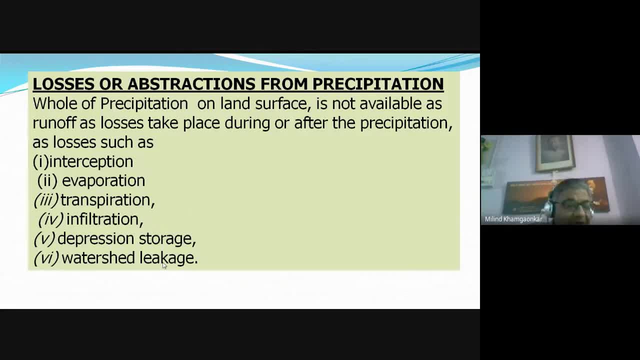 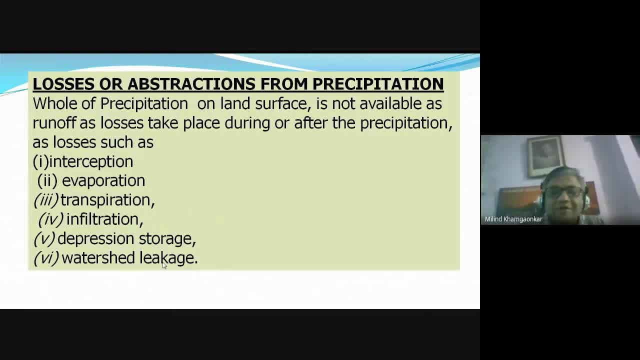 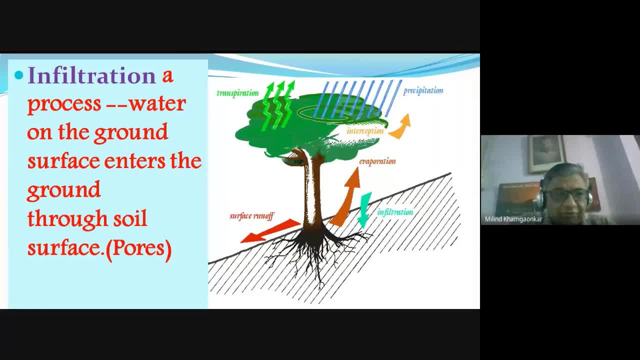 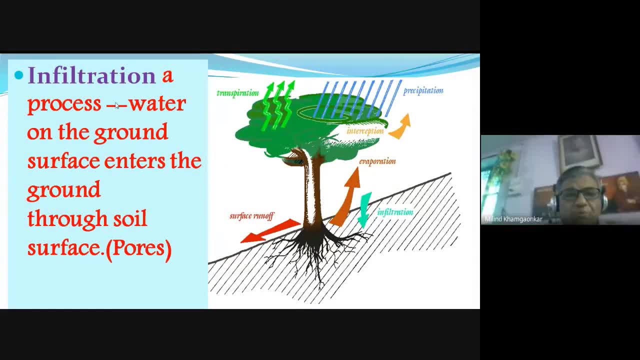 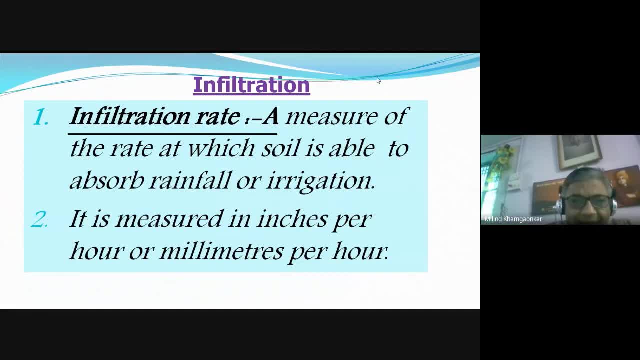 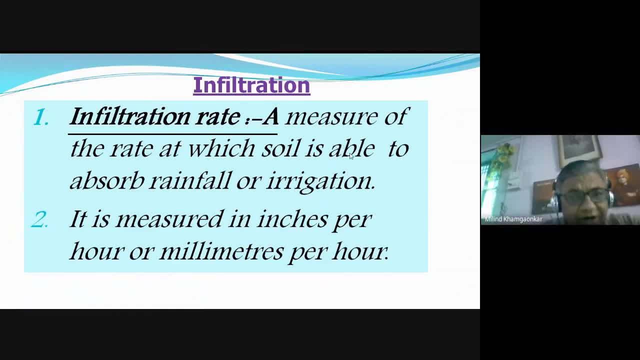 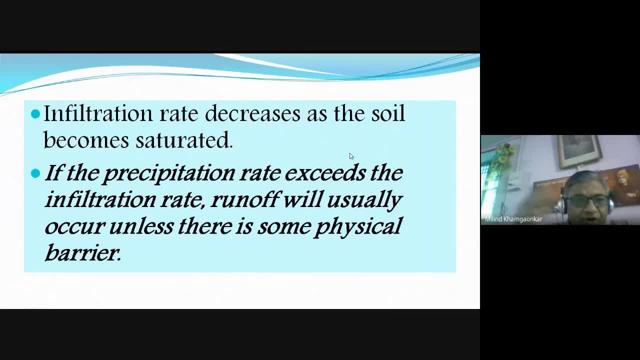 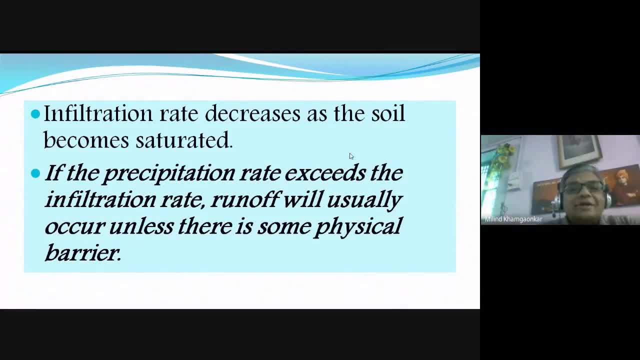 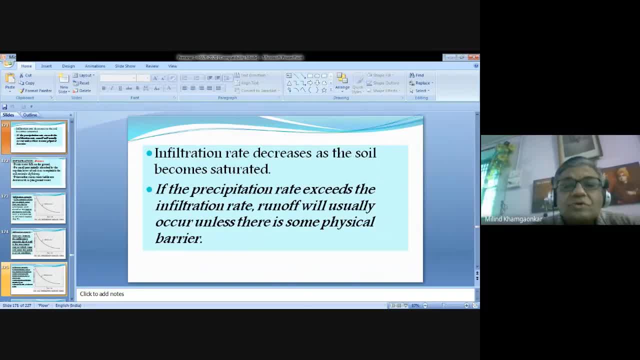 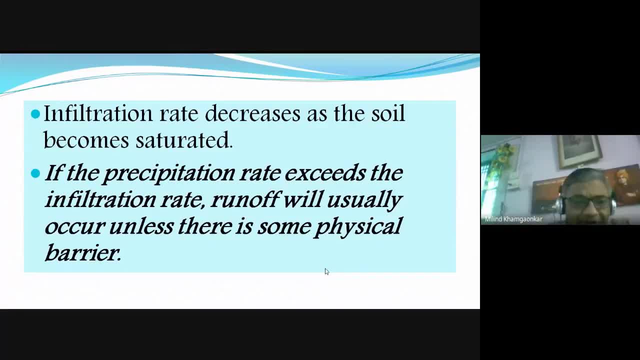 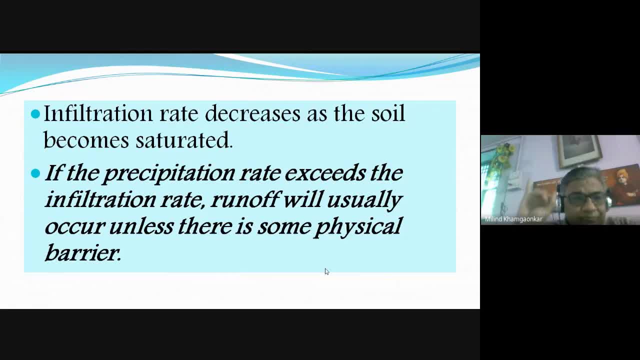 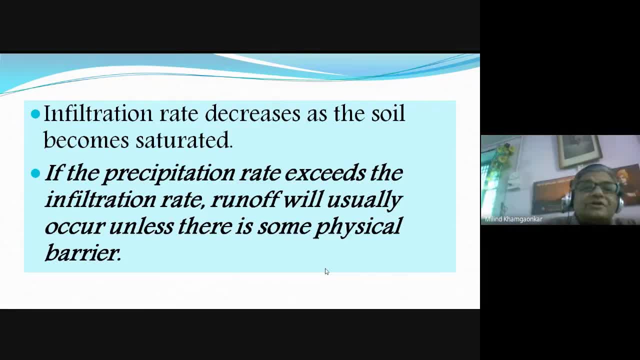 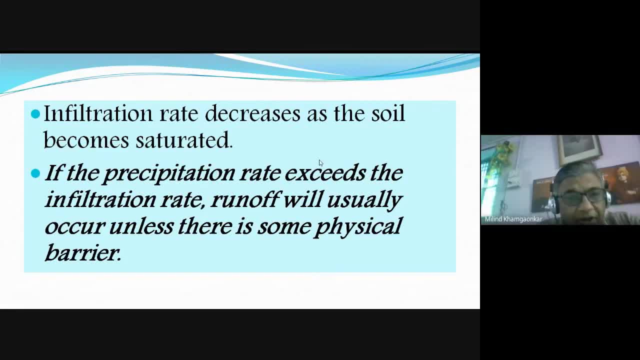 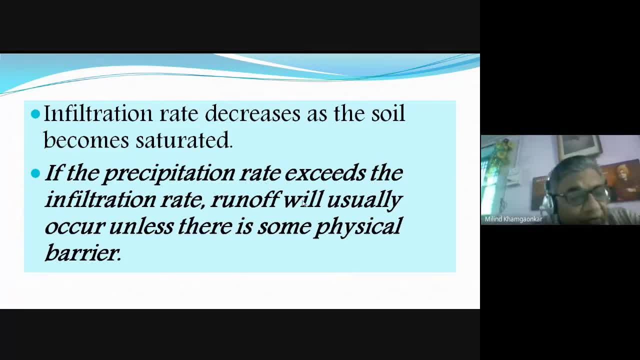 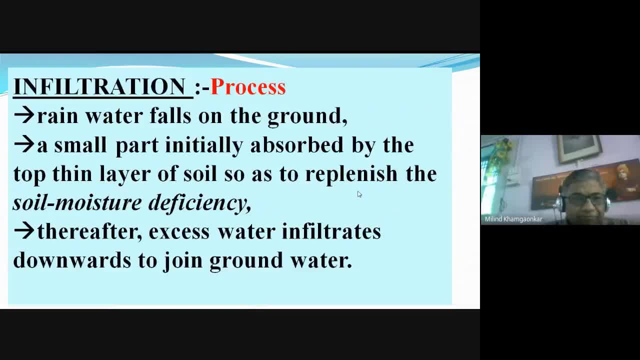 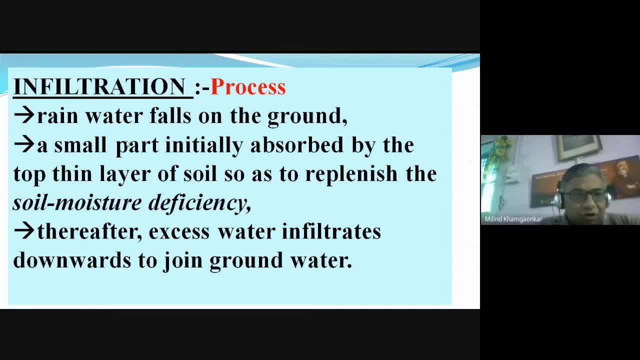 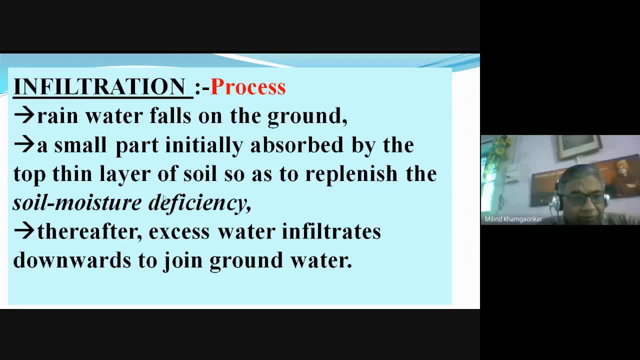 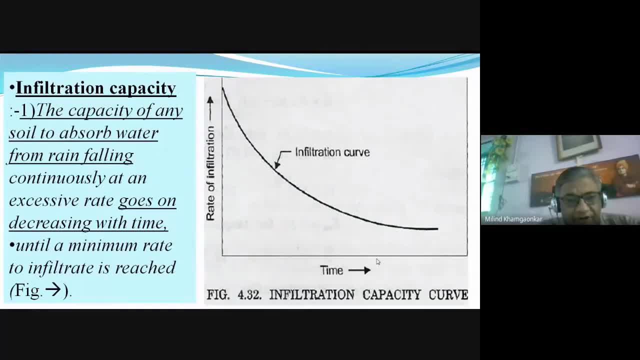 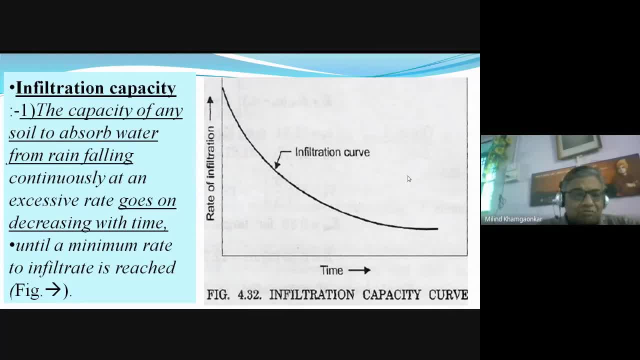 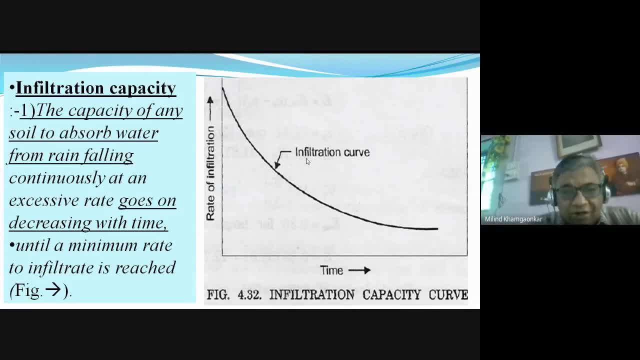 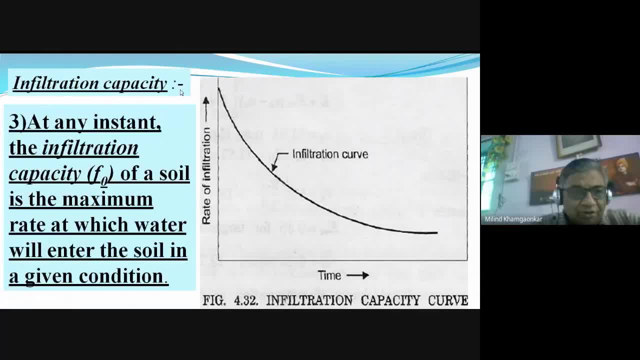 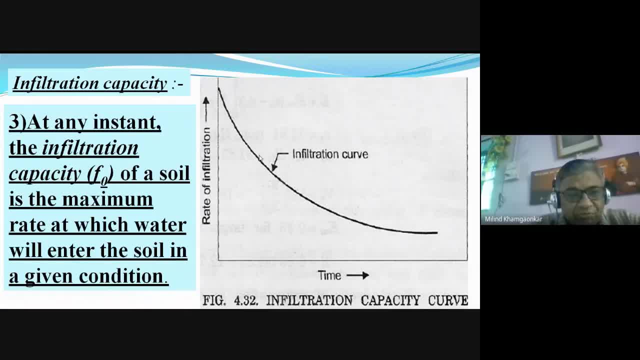 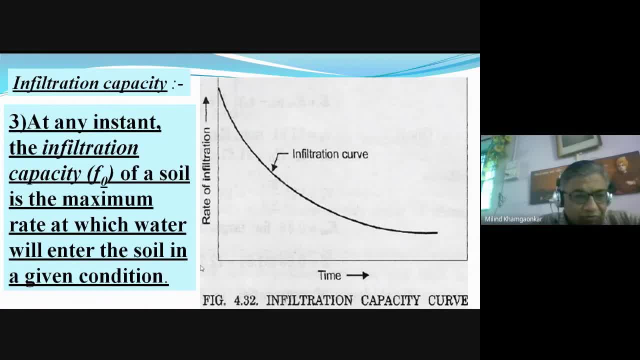 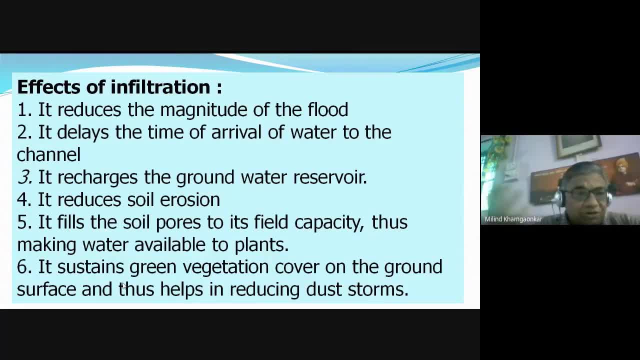 evaporation control chemical. how to measure the evaporation control chemical. how to measure the curve or infiltration rate, curve is very important. there are the effects of the infiltration. the main effect is it reduces the flood. it percolates the water into the soil, which is very helpful from the point of view of the 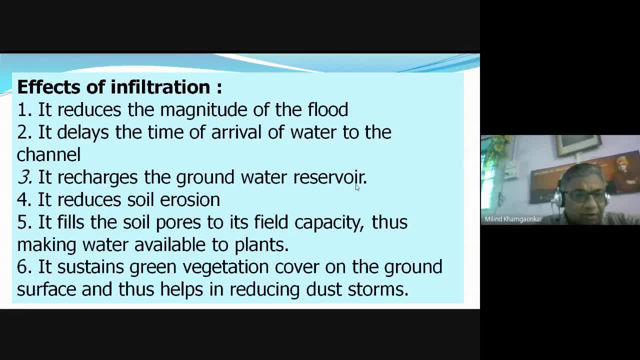 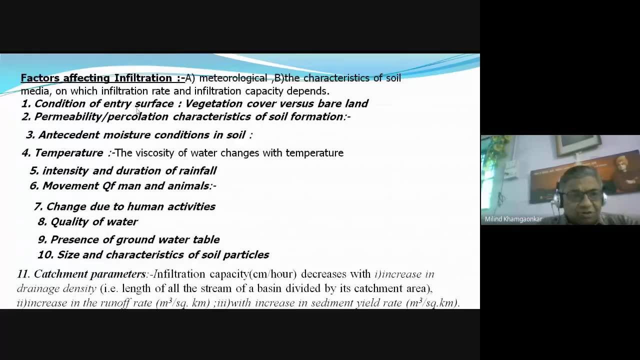 forest or the greenery. it increases the groundwater table, it reduces the soil illusion. so all these are the good effects, are the effects of the infiltration. there are various factors which affects the infiltration. again: the ground surface, whether it is forest, vegetative cover or dry, or the bare. 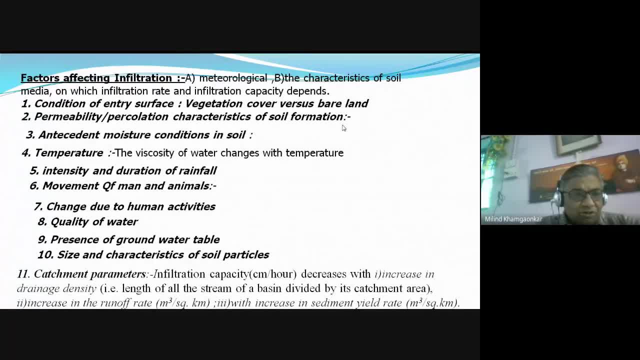 permeability characteristic of the soil. that is the geology antecedent. moisture condition means before the rainfall occurs. what was the soil? whether the soil is moist, its soil. moisture condition means before the rainfall occurs. what was the soil? whether the soil is moist, the atmospheric temperature, intensity and duration of rainfall. movement of the. 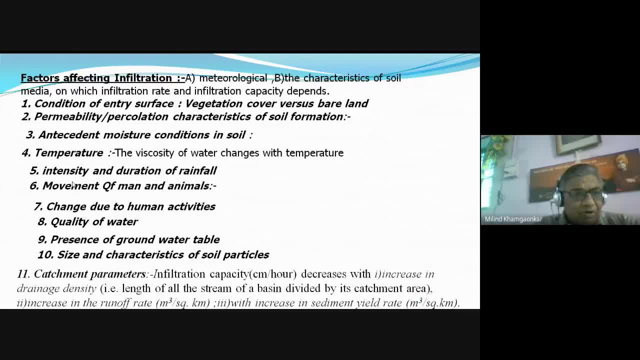 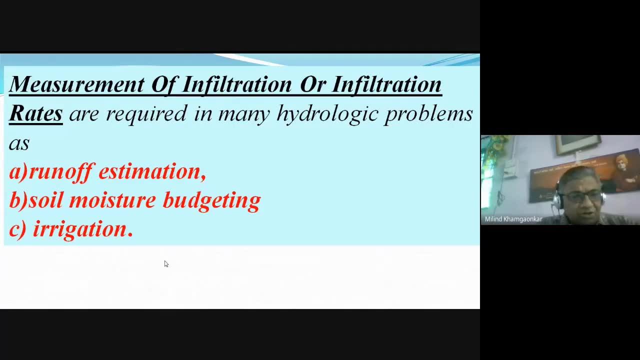 man and any fun. all these are the very important factors. the catchment parameters: where the catchment has got lot of the depressions or the storages, that also affects to the infiltration. there are various methods to measure the infiltration. infiltration is being measured by the runoff estimation soil. 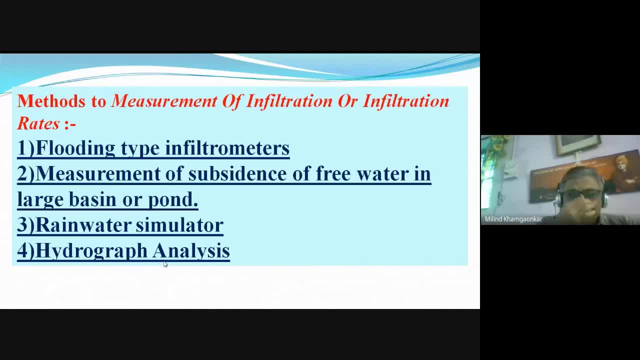 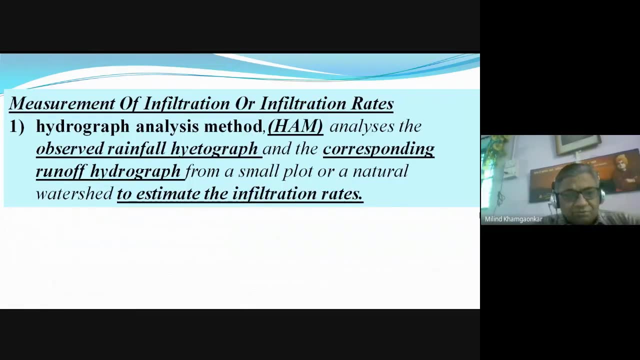 moisture budgeting and the irrigation. the various methods are: flooding type infiltrometer with the measurement of subsidence of free water in the large we see rain water simulator. hydrograph analysis. these are the various methods. various hydrograph analysis in very a hydrograph analysis method. the 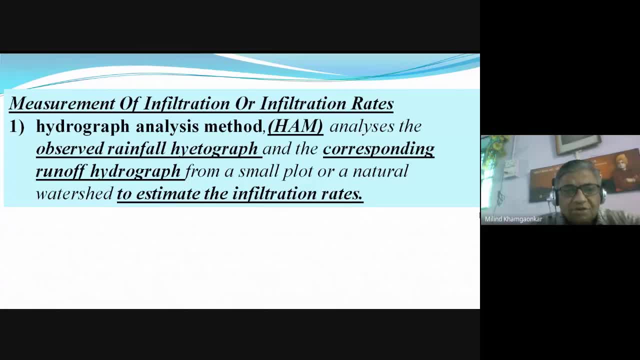 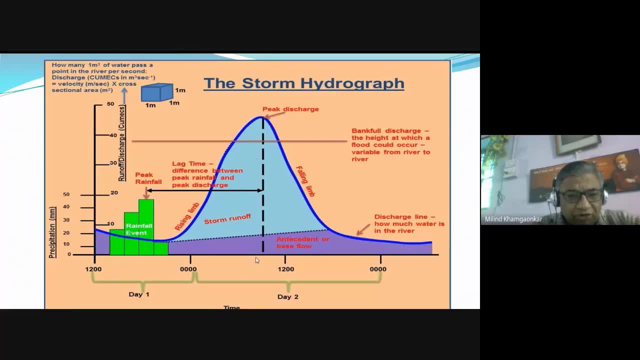 infiltrated water, which is called as the best flow, is being separated out from this hydrograph, storm hydrograph, which is also nothing but better up between the duration of time and the runoff. ascert in location. were you? you see the the portion which is shown in dark shade, dark. 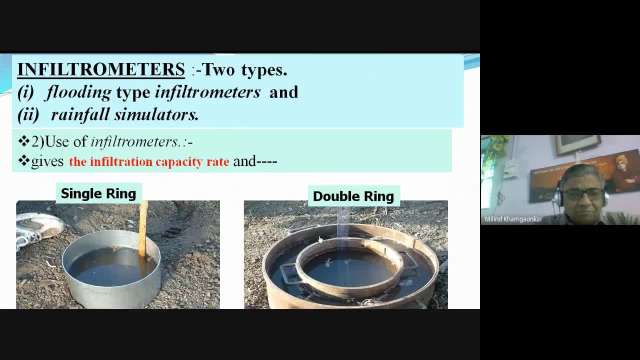 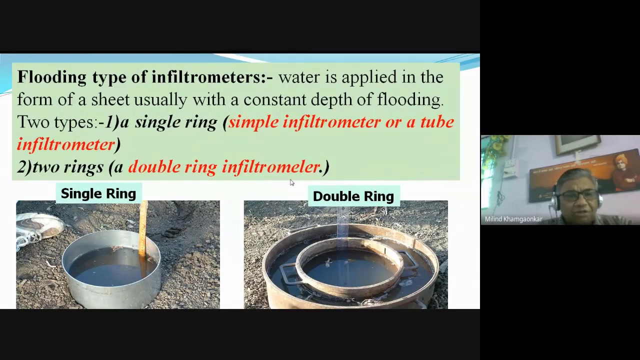 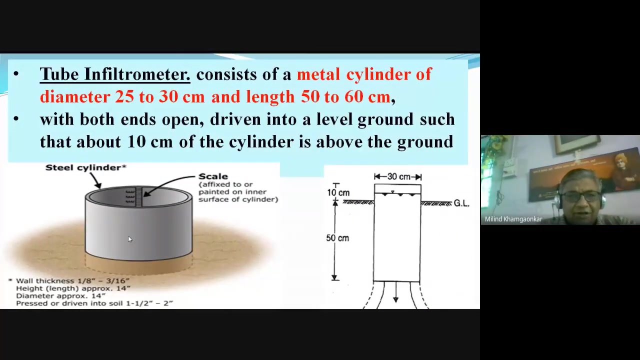 blue is the infiltrated water. there are certain equipments called as the infiltrator infiltrometers. there are two types of the hidden filter meters: flooding type infiltrometer And the rainfall simulators are there. Flooding type are also further divided into single ring and double ring of the infiltrometer. The fundamental of all these infiltrometers is that the water is being poured in. this container may be a diameter of, say, 25 to 30 centimeters and the height is 50 to 60 centimeters. 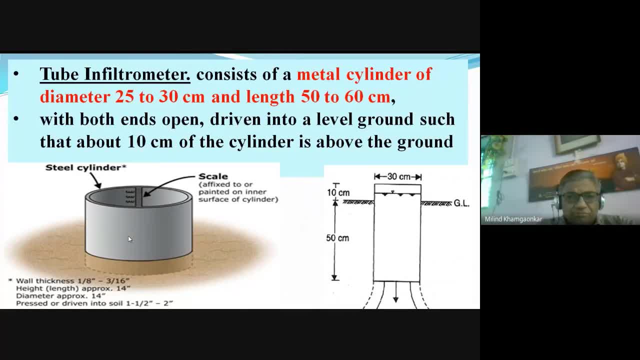 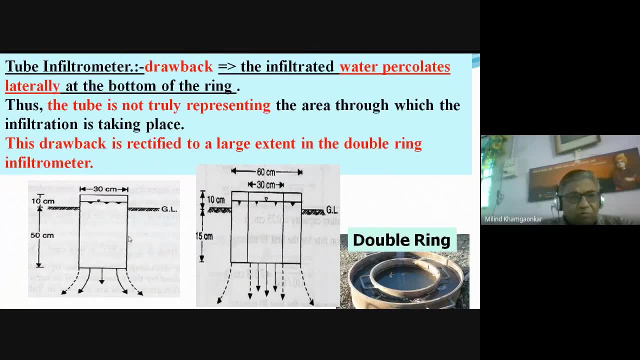 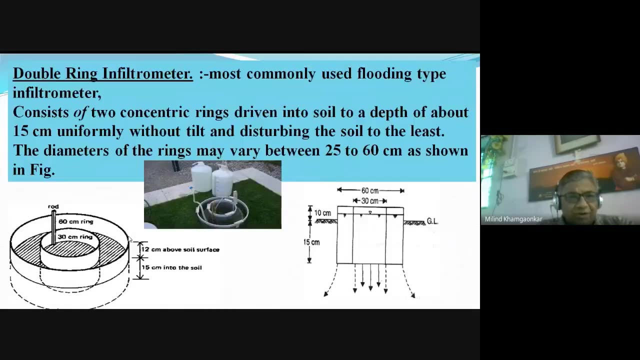 Because it is put into the ground and water is poured into this infiltrometer and the percolated water is being found out along with the time, and the percolation rate and the infiltration capacity of the soil is being found out either with the help of the single infiltrometer or the double ring infiltrometer. 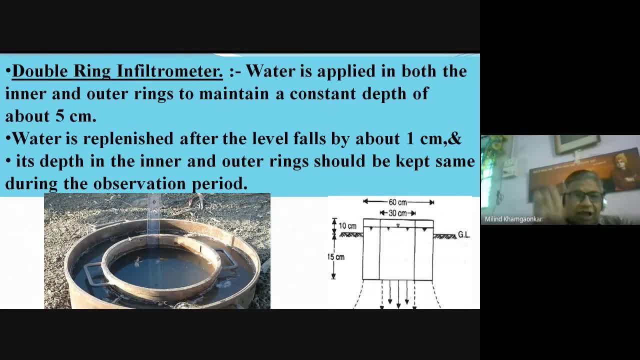 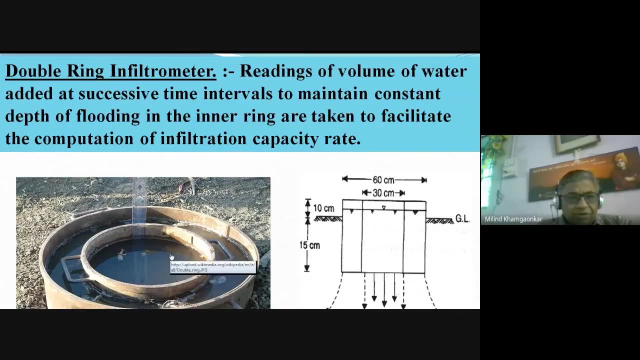 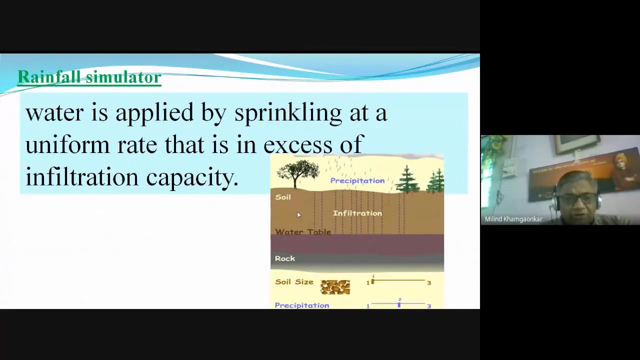 In double ring infiltrometer, the disadvantage due to the single ring is being overcome And therefore the measurement of the loss of water in the central container is being found out in the double ring infiltrometer. There are certain rainfall simulators are there wherein a certain plot is selected and on this selected plot, artificial precipitation with the help of the sprinkling of water is being carried out and the infiltration is being formed. 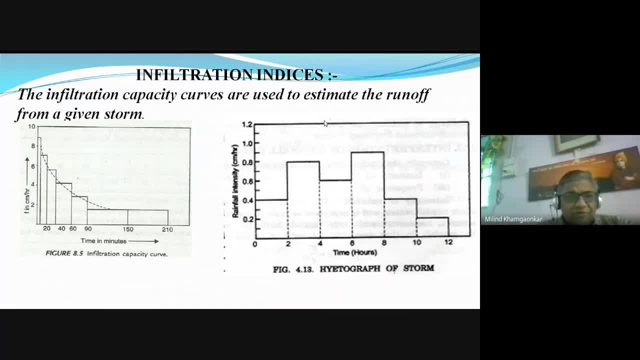 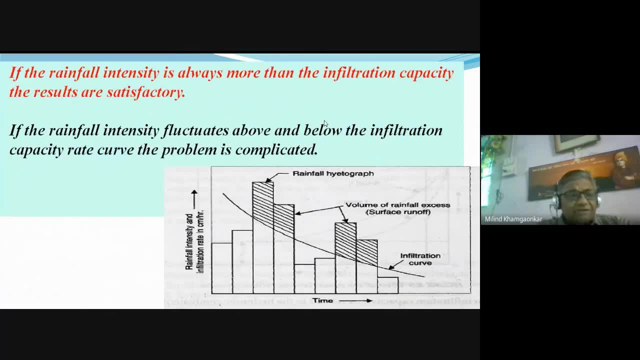 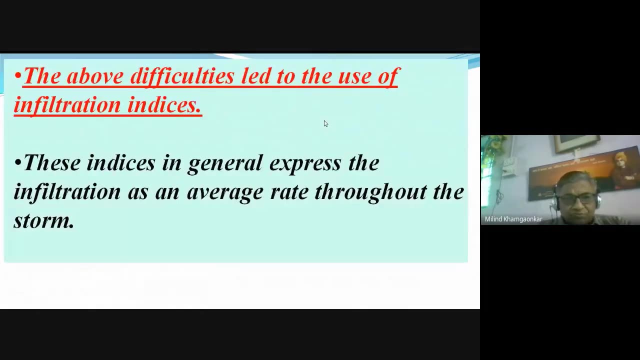 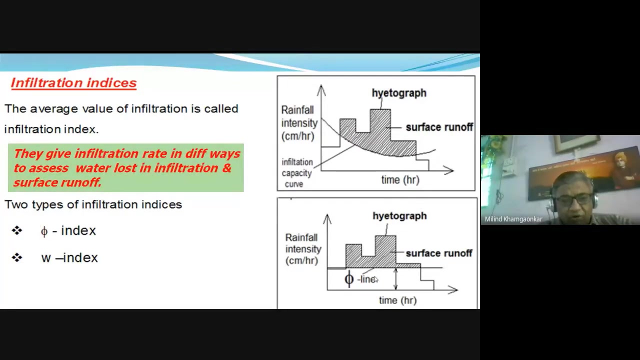 There are certain indices. they are called as the infiltration indices. They are the two types of the infiltration indices are there. They are the phi index and the W index. The phi index is nothing but the index below which, if we overlap this phi index value, it is nothing but a rainfall intensity. 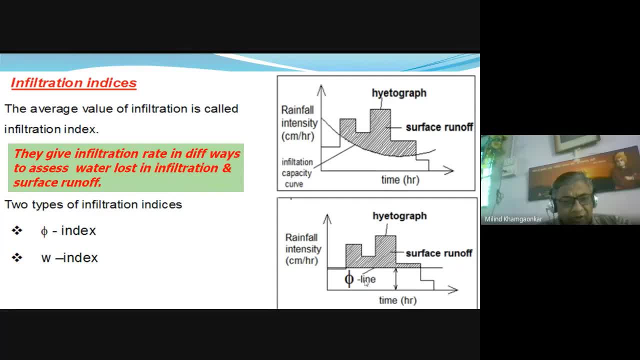 It is nothing but a rainfall rate that is centimeters or millimeters per hour. If and this phi index is constant for a certain catchment area, the W index is constant for a certain catchment area, These two indices are nothing but phi index is the precipitation rate or the rainfall intensity and the W index is nothing but the infiltration rate. 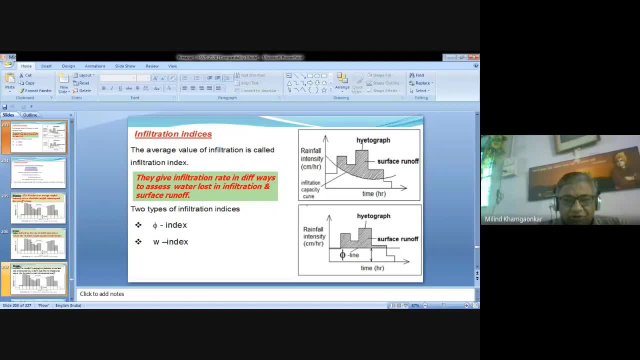 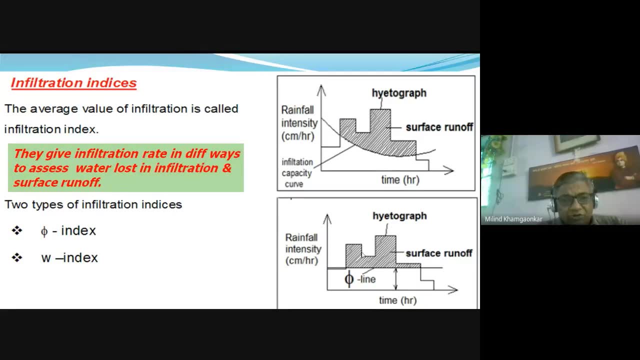 So both these indices are used to find out the exact quantity of the runoff. OK, Phi index gives, after deducting the value of the phi index or the rainfall intensity for a particular duration from the rainfall quantity, whatever remaining quantity we get. that is the surface runoff. 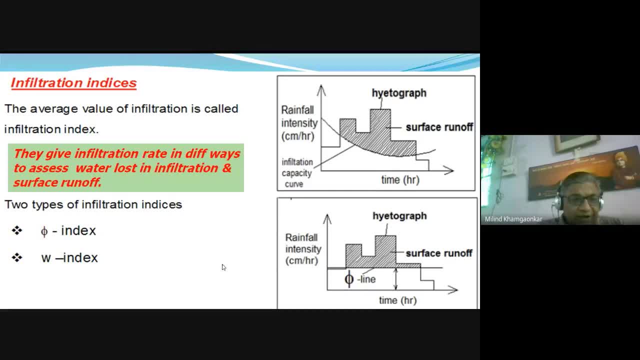 But W index is more precise than the The Fine Fine Index or it is less than the findings. The W index value excludes all the other abstractions Below this phi index value are: the phi index includes Infiltration plus other abstractions like the intersection, depression storage etc.